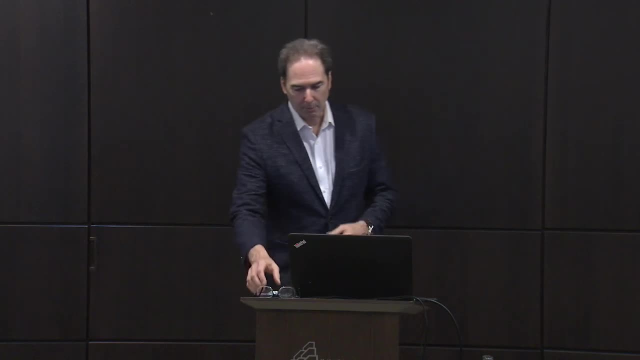 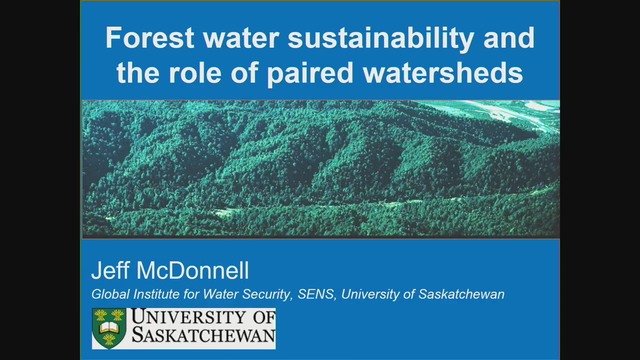 period or over a beer at Boffin's afterwards, because these ideas have been kind of gelling over the last weeks and months. This is a question of sustainability- Many of us are in SENS- And this is forest water sustainability in the context of what is the most popular technique in forest hydrology. 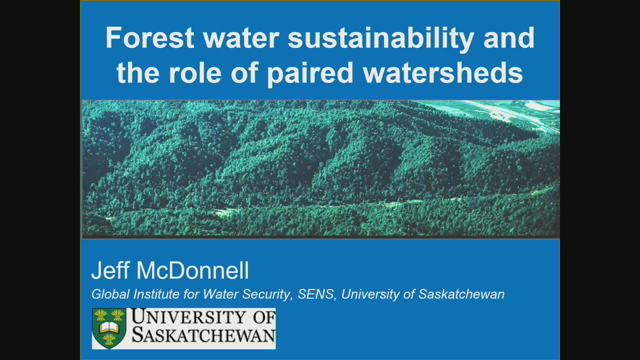 and that's something called the paired watershed approach that I'll discuss This photo. we're going to come back to this at the end of the talk. This is where I spent a lot of time in the field in New Zealand. This is the Maimai Watershed. In fact, this 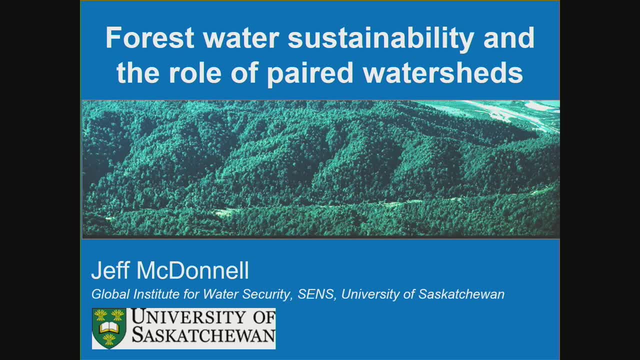 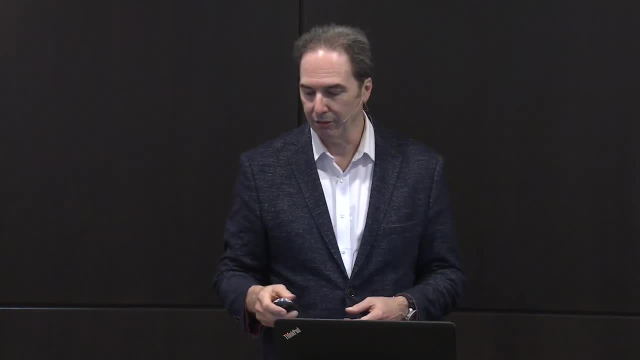 day thirty years ago, I was out on a steep slope here making measurements during a rainstorm. I'm still working there with some of my students and I'll talk about maybe some of the things that I've learned in this intervening time as it relates to forest water sustainability. 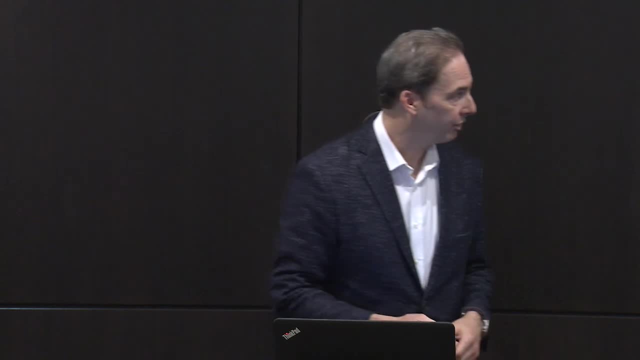 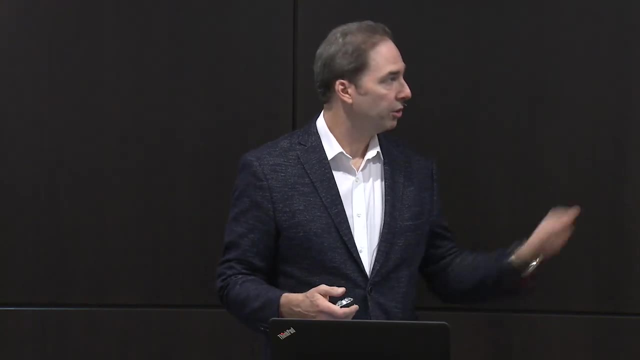 and this kind of paired watershed approach. So that's the idea going forward. So in these intervening thirty years I've been working on hill slopes in different parts of the world. This is one in Georgia. My work spans from the plot scale, maybe a chunk of 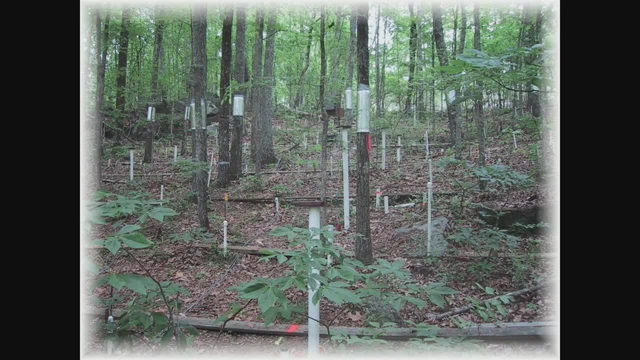 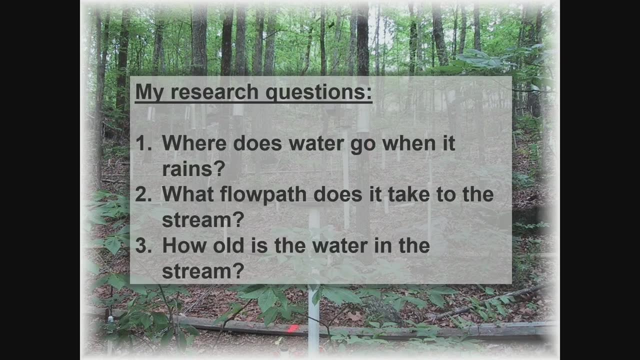 soil as big as this podium to headwater catchment And hill slopes are kind of the basic structural unit that my group often works on And our questions have been the same for three decades: Where does water go when it rains? What flow? 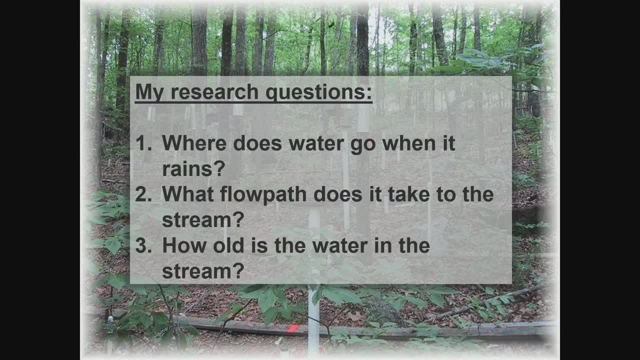 path does it take to the stream And how old is the water in the stream? These are simple questions but surprisingly difficult to tease out in diverse systems, And it's this that I want to kind of relate to as we go through the talk today: These basic questions of how. 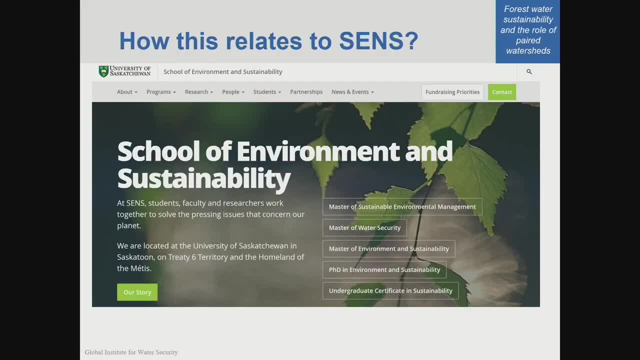 to work on a rich, sustainable environment. What does it mean? What do we do to make it work, What are the possible incentives for that And what are the skills that are required to do that, And what are some of the things that we do to make it work. So I want to talk. 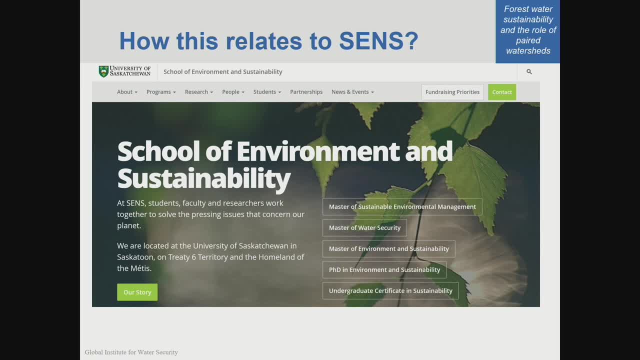 a little bit about this topic and I think the most important part is, of course, the question is actually how to work on a rich, sustainable environment, And this is something that we're going to talk about in the next few days. So the first question is really about the next part of this webinar. I want to talk 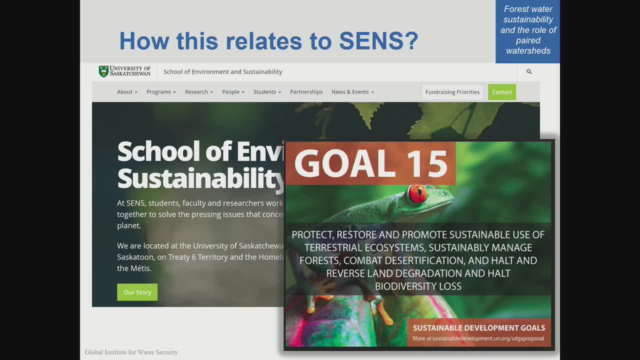 about this four-part topic here, and I'm going to start with the four-part topic, which is about the environmental impact that happens when your school develops and your school develops, and your school develops. And finally, I want to talk about the entire Sustainability, as a term was first coined in the early 70s and as it relates to forestry, this goal 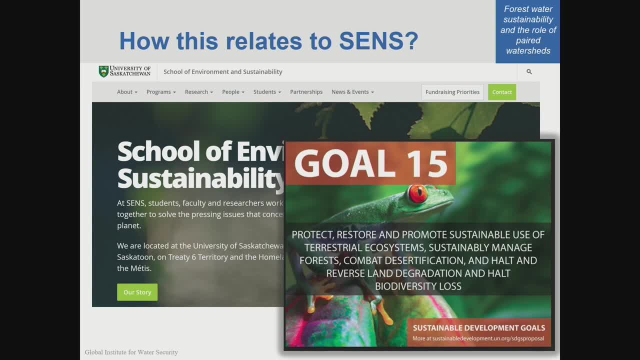 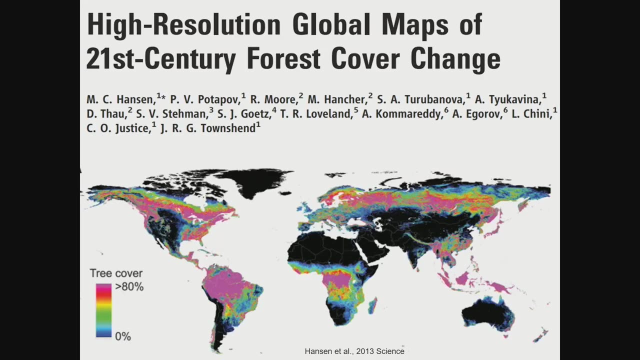 15 of the UN sustainable development goals, focusing on protection, restoration, promotion of sustainable use of forests is really how my work and my group's work kind of maps to this issue of sustainability, And sustainability is a big issue in forests. This was a very important. 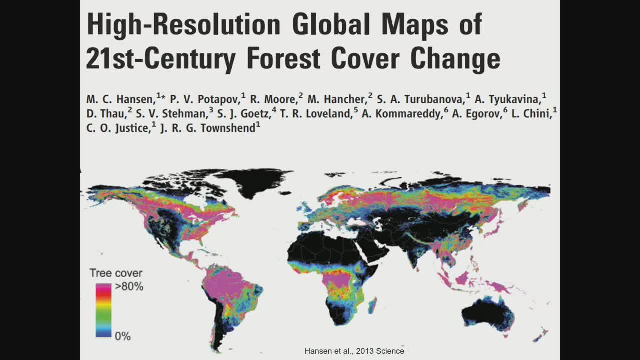 paper published a few years ago in science by Matt Hansen at University of Maryland and it was the first really high resolution mapping of forest cover globally and you can see the maps here. the scale is percent tree cover, these colors that you see across the map and the big thing in this: 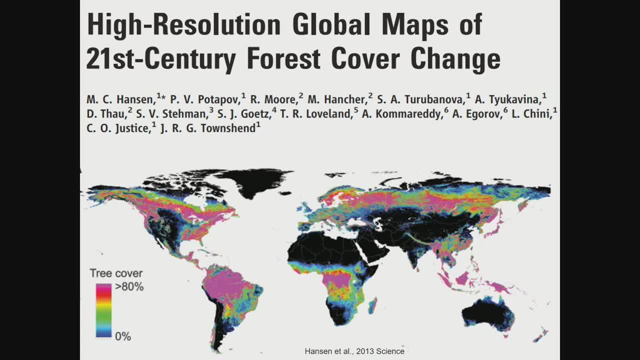 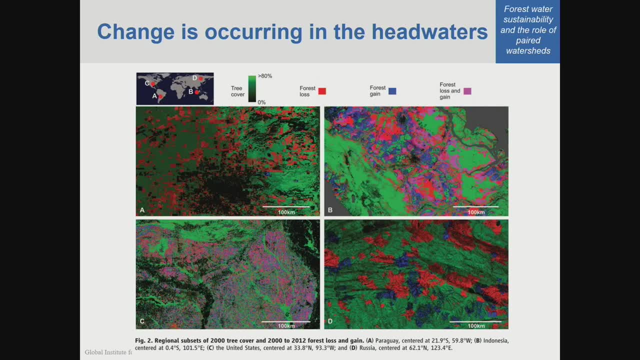 paper was a kind of a detailed outline of where change is occurring, and if you zoom in on one of the diagrams in this particular paper here you can see some places. so A is a site in Paraguay. you can see the map in the upper left hand. 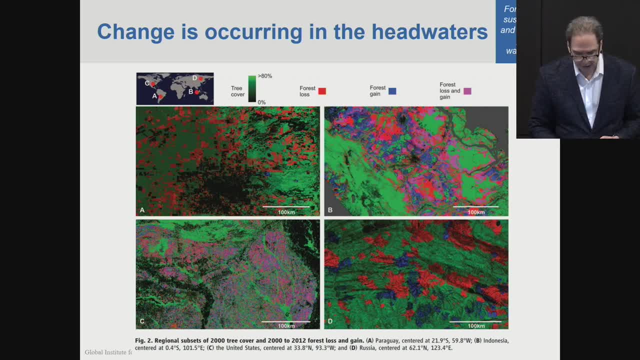 corner on your screen. there B is a site in Indonesia, C is in the US and D is in Russia. just take a look at the scales. those horizontal white bars are in as a hundred kilometers. so this is the grain, the resolution of where change is happening. it's happening in headwater systems, happening in. 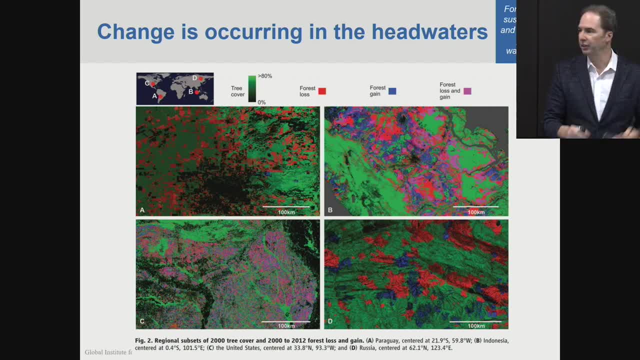 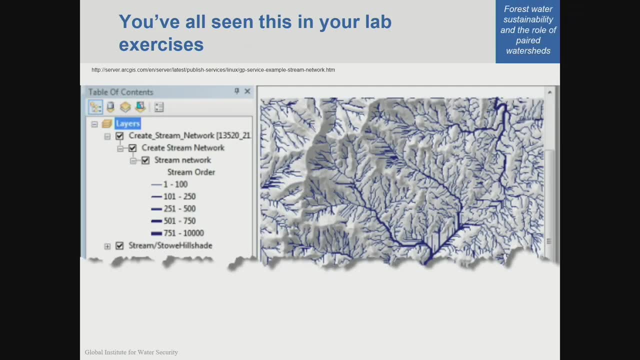 small drainages on the landscape. that's where the change is happening. That's the the granularity, if you like, of this change and this. this is what many of you have seen in your hydrology courses and if you're in the masters and water security program or you're doing watershed, 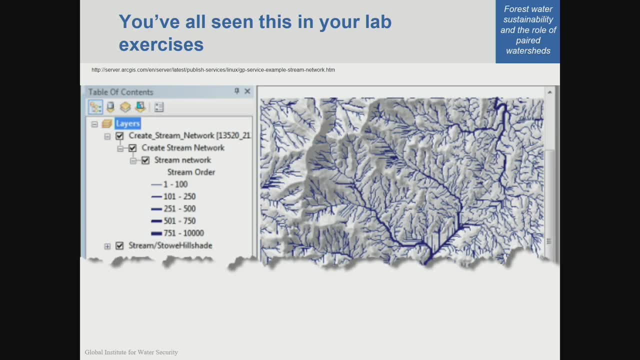 related work. you see this when you do your ArcGIS studies. here's an ArcGIS illustration of topography: lots and lots of these small headwater streams that are draining first-order watersheds that are then forming the larger watershed. The change is happening in the landscape. 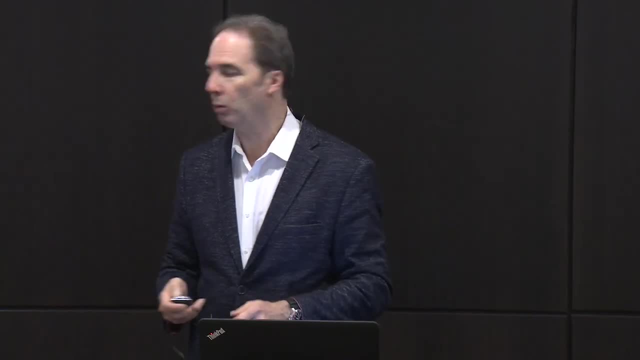 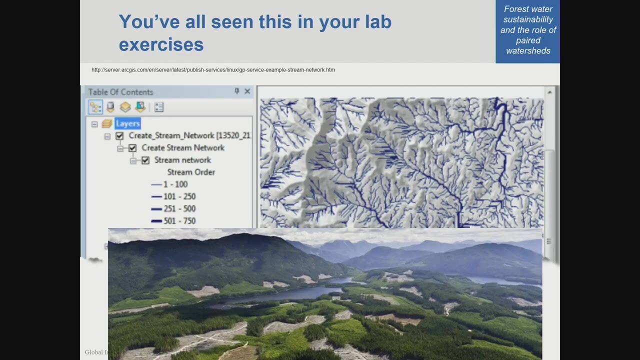 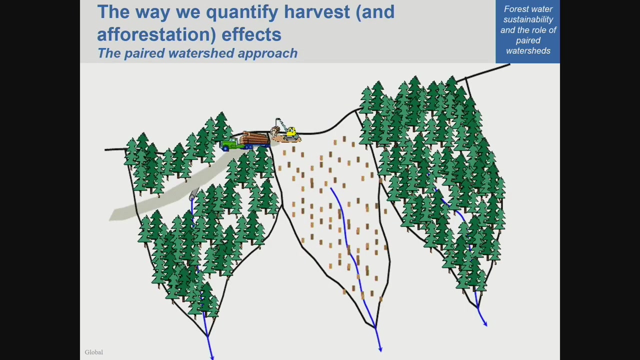 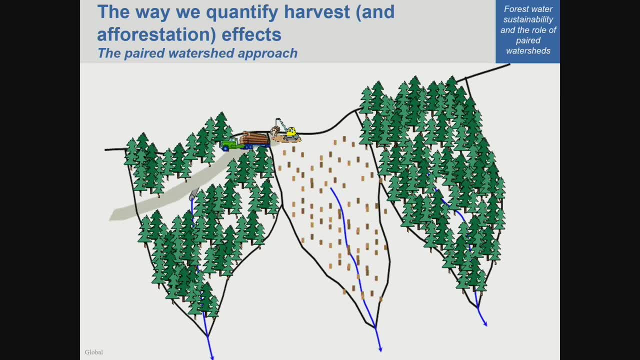 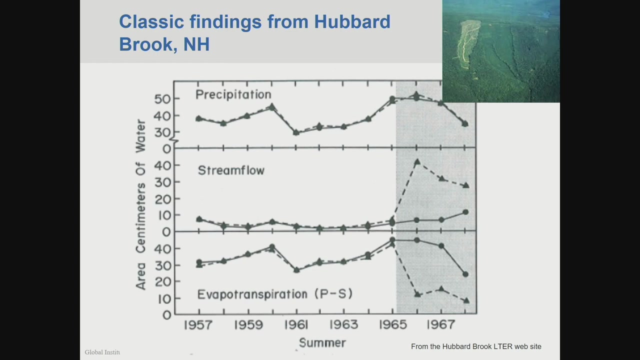 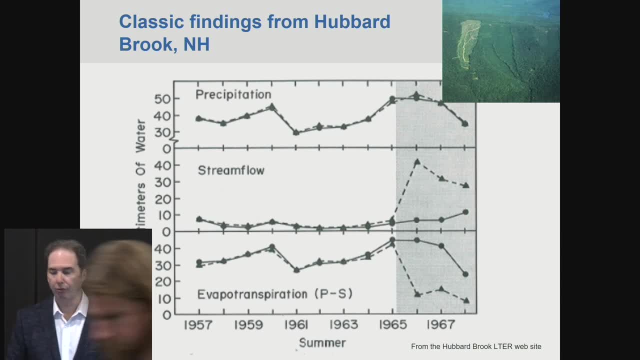 and just look at this graph. so on the y-axis this is think of these as water volume distances from 1957 to 1965. this is a classic. you see the two lines plotting very closely. and you see the two line plotting very closely: one is the overtime per acre and one is the output below its unit per acre, and one is the output above its unit per acre and one is the output below its unit per acre. and these use water pressure between the two allí plants to monitor or generate, between the two allí plants to monitor or generate. 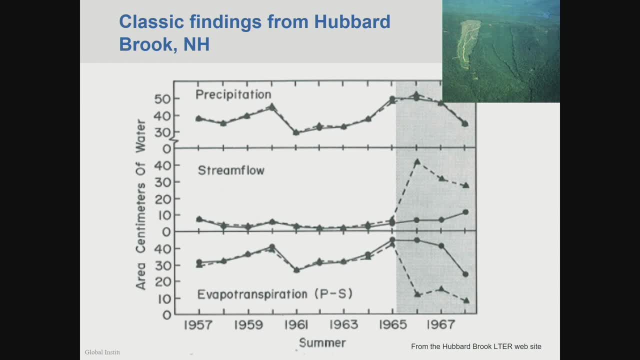 control, and the dashed one, which is almost overlapping during that period, is the one that's going to be treated. Then, after the treatment that you see in the shaded area, what happens? Well, precipitation stays the same right because the forests haven't really affected the local precipitation at 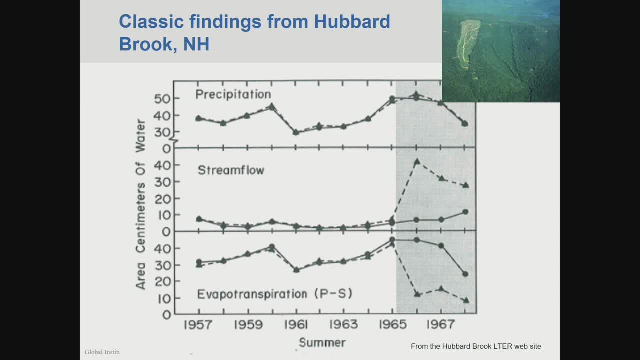 least. But what you see is a big uptick in stream flow and a big downturn in evapotranspiration for the watershed that's been harvested. This is a really, I think, vivid illustration of the power of this paired watershed approach. It's not. 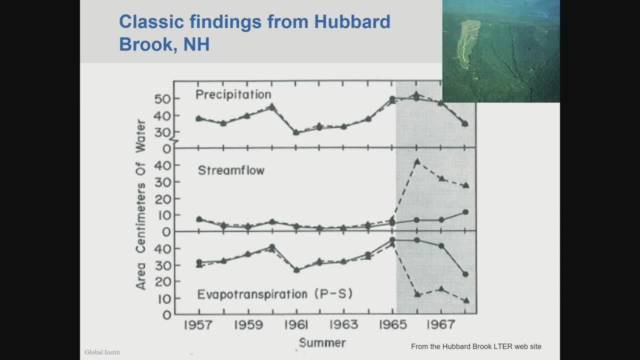 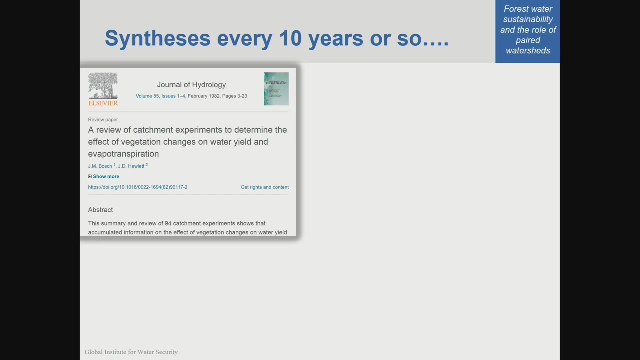 something you can get with a model so easily because there are site details. The primacy of these local conditions is so key in these kinds of responses to forest harvesting or afforestation. We've had synthesis papers now about every decade, starting with this one. This is Bosch and Hewlett 1982. It reviewed at: 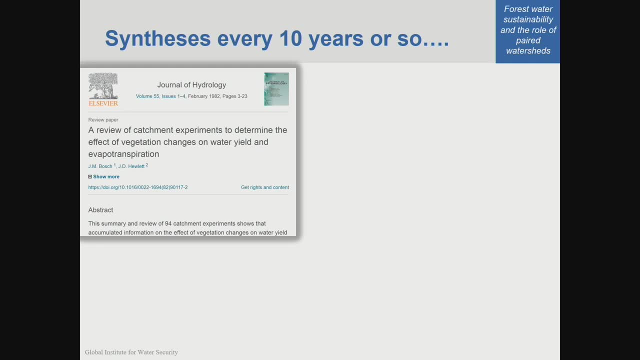 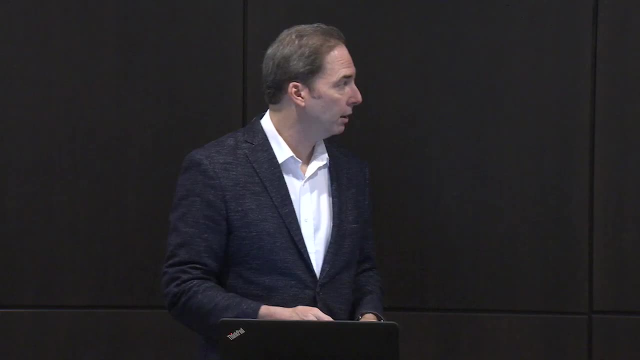 the time about 50 or so paired watershed samples studies that had been done. This started in 1929 with the first experiments done in Arizona at Wagon Wheel Gap And this was the first kind of review of these studies. This was updated by John Stednick in 1996,. 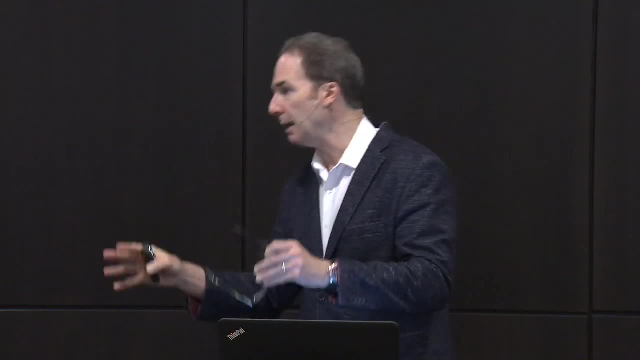 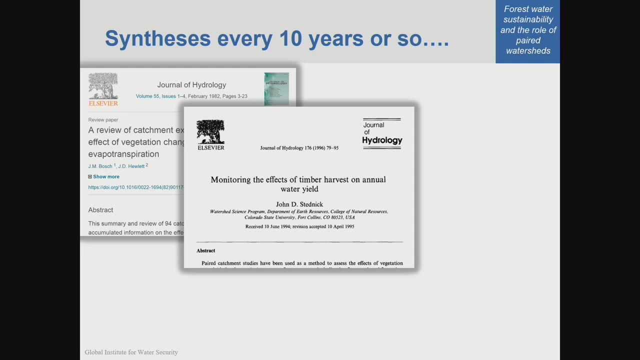 adding a few more data points, maybe in different climates, And each of these updates really focused on: well, what does the accounting model say in terms of how much increase or decrease in stream flow did we have in response to forest treatment? And, surprisingly, it was highly variable. 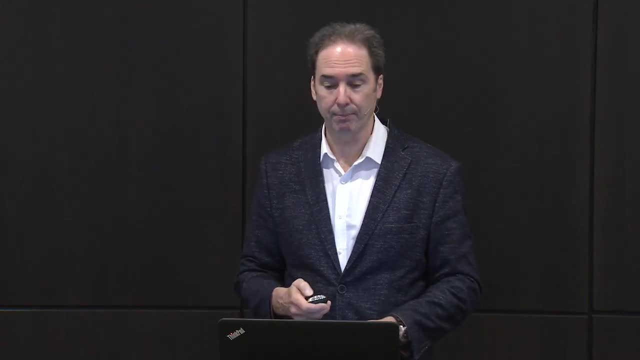 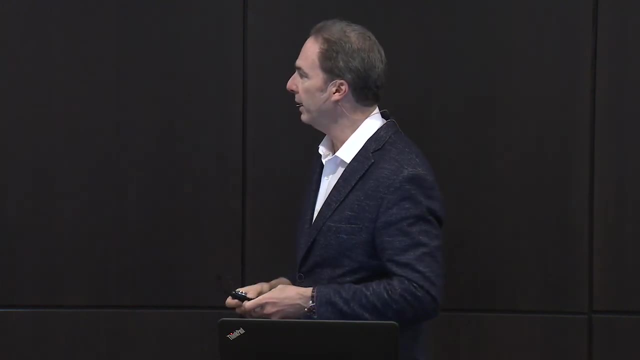 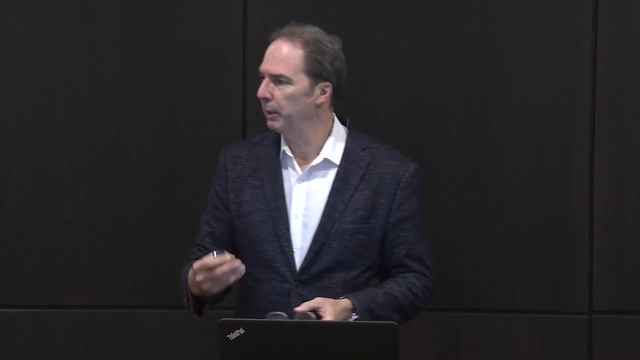 Sometimes it increased, sometimes it decreased, sometimes it stayed the same. This is a more recent and this is the most recent update. I think this was done in 2005, led by a group in Australia at University of Melbourne, And they applied a little bit more. 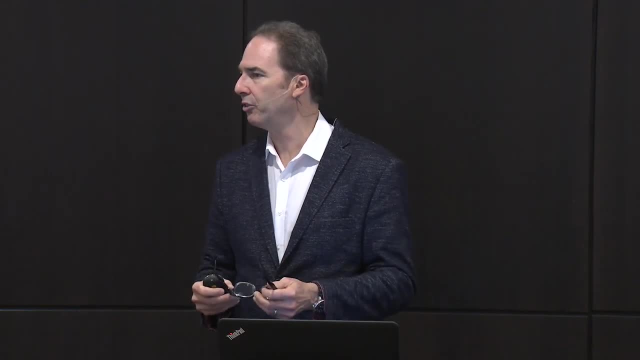 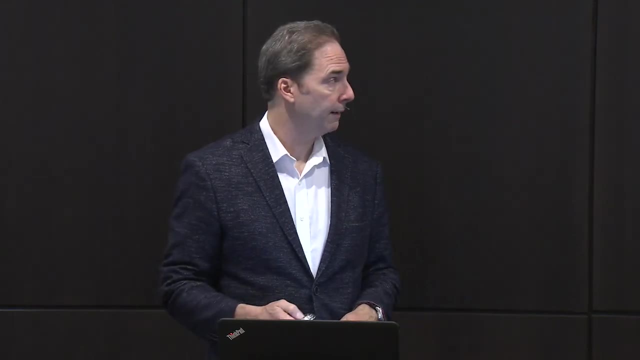 in terms of flow duration, curves and other flow characteristics. But the bottom line, these were all based on these outputs from paired watershed studies showing a lot of variability. To date there's been over now 300 papers, 370 at last count. 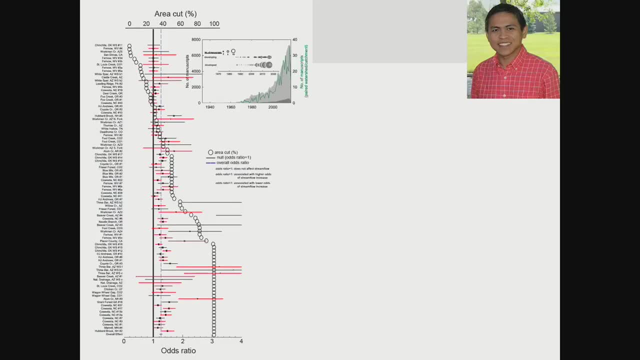 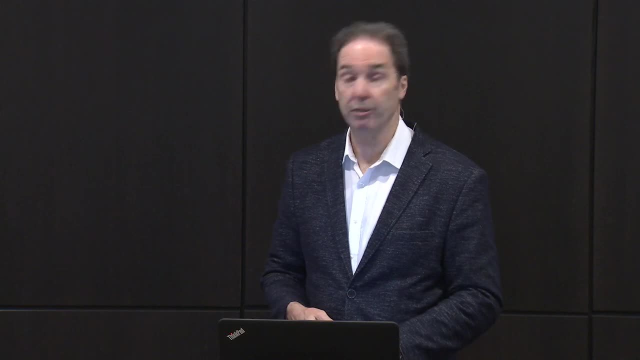 with at least 120 paired watershed studies, And Habame Evaristo, a recent PhD graduate from here in SENS, who's now an assistant professor at the University of Nevada Reno, is leading the next update, if you like, or meta-analysis of these data. 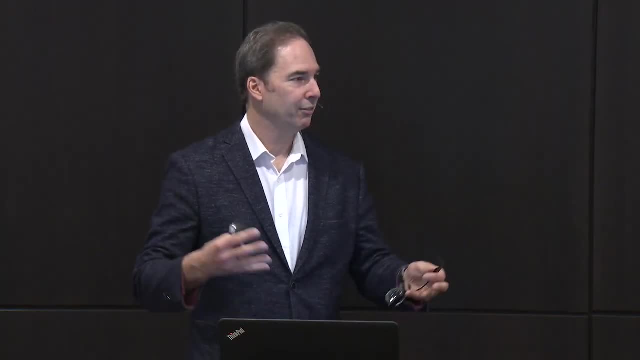 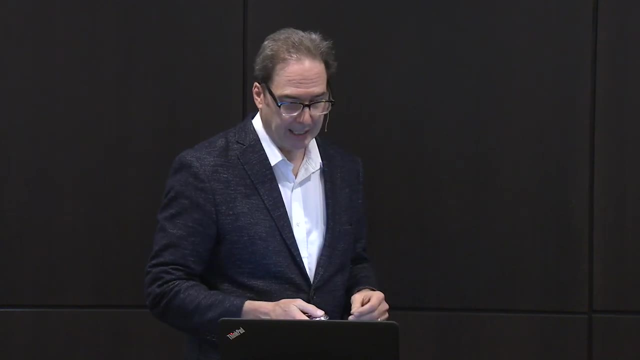 And you know, being in Nevada now- and Reno, he's taken a kind of a gambling approach. This is an odds ratio he's showing here. Let me try and walk you through this graph. It looks more complicated than it is. Just focus first of all on that vertical line. 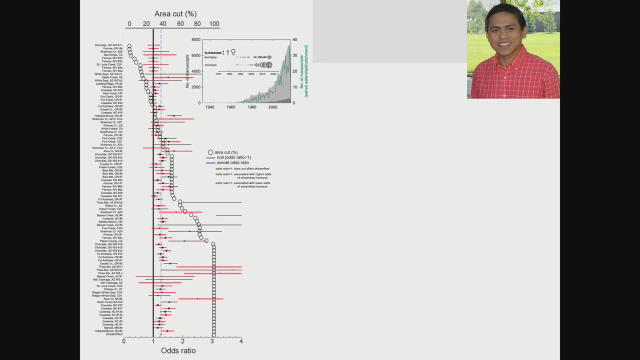 Those are the 90 or so studies that have been published in the US, paired watershed studies, And what he's done is plotted along the x-axis up top the area cut. So zero would be- none of the watershed was touched, and 100% would mean it was clear cut. 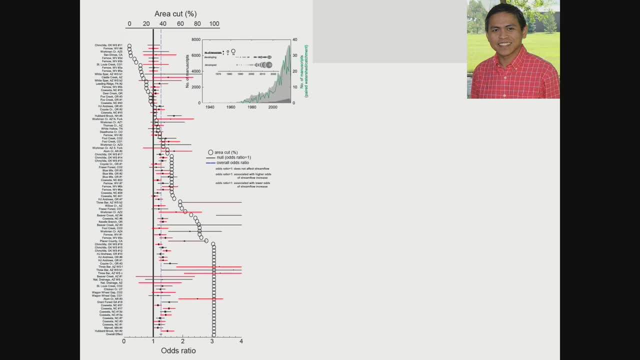 And look at the open circle, The circles that start in the upper left and kind of continue down and move to the right. This is how the studies are ranked. They're ranked from small cut to large cut area. Now the interesting thing in this diagram: 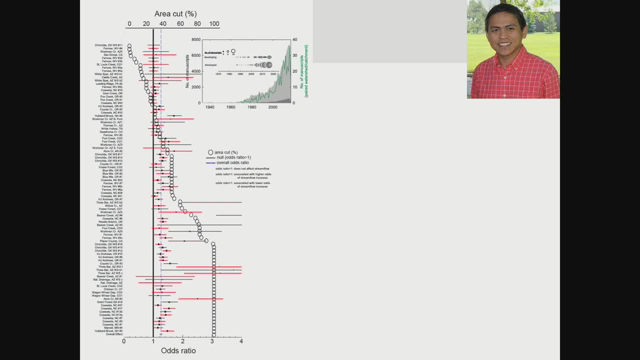 is. the red line shows the flow response, either up or down or what's happened. And the curious thing is, for areas that have very small amounts of cut, you can have large change Or you could have areas that were 100% clear cut. 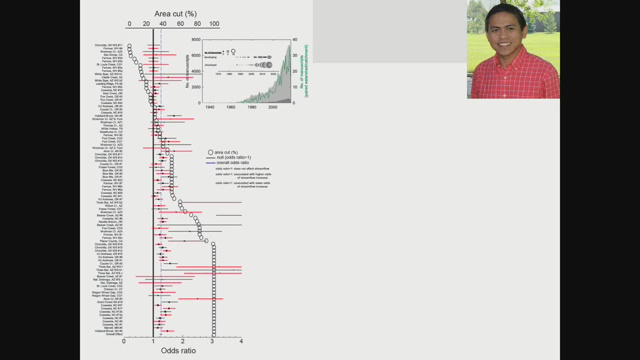 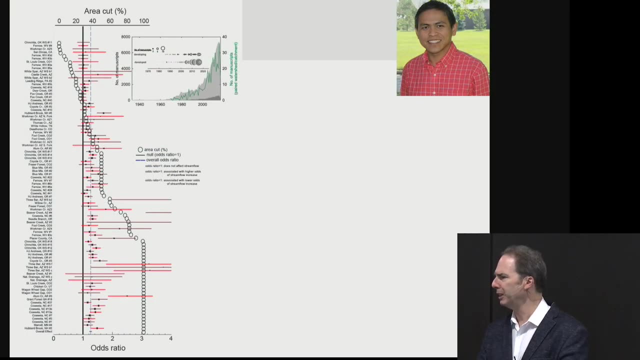 and had minimum change, And change is defined by this thing called the odds ratio on the bottom there. So one to one odds would mean there's no increased possibility of change And, as you go, positive. so an odds ratio of two to one. 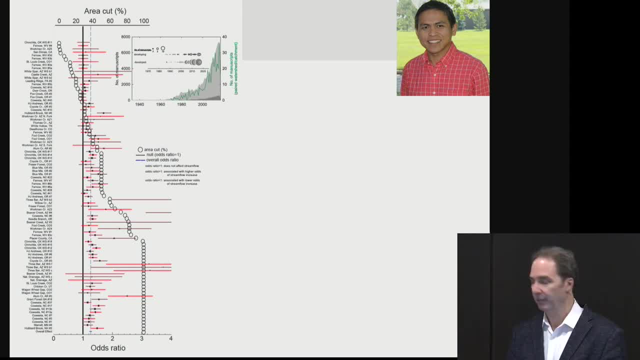 three to one. this is increasing the odds of getting a response And if you go negative, it means that flow went up rather than went down. This gives you an idea of the difficulty. Individual sites: this is a very powerful technique: Looking across sites. 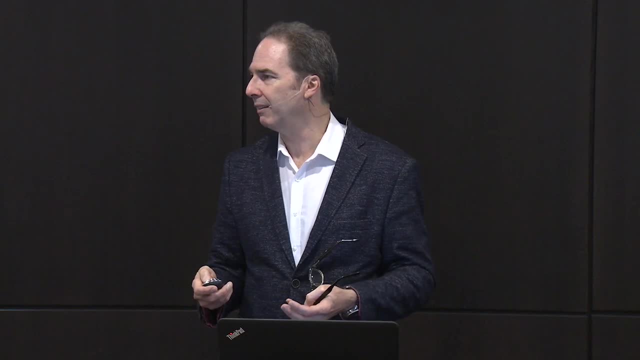 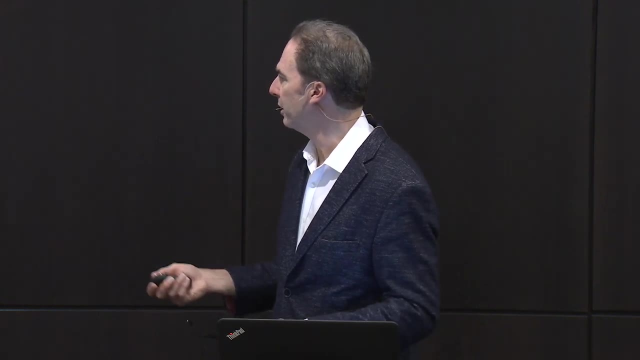 It's tough to kind of make sense of all these data And this is what I'm trying to do in this little paper. I've had an invite to lead. It's a new journal launching in January And I was mentioning to Saman I've got many co-authors here. 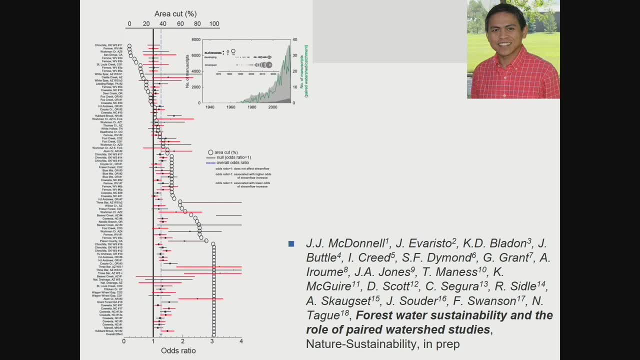 18. And I sent them all a version, first draft, of the paper And I've had about 20 different perspectives now on the paper. So this talk is kind of a way for me to organize my thoughts in terms of maybe how to respond. 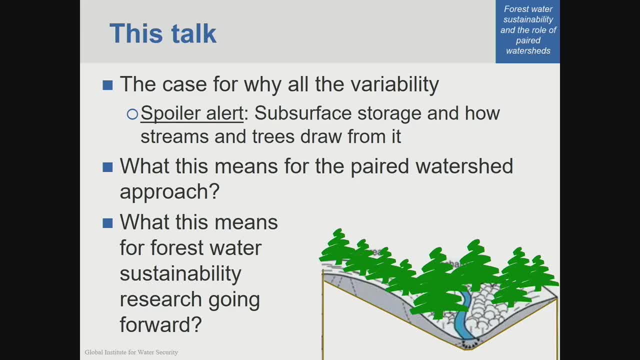 to my 18 co-authors. But what I want to do now- this is the outline now for the talk over the next half hour or so. I want to make a case for why maybe we see all this variability, And the spoiler alert is that I think 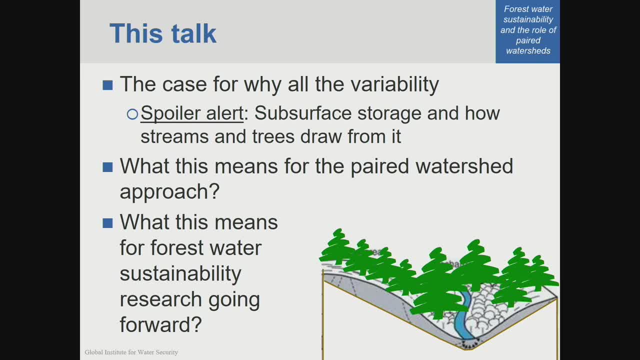 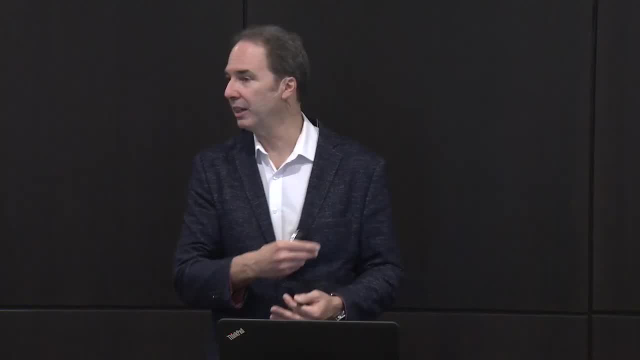 it has to do with what's below ground, And this is the thing we've never really come to grips with in any of these paired watershed studies. We always look above ground. How many trees do we cut down? How did we affect the interception? 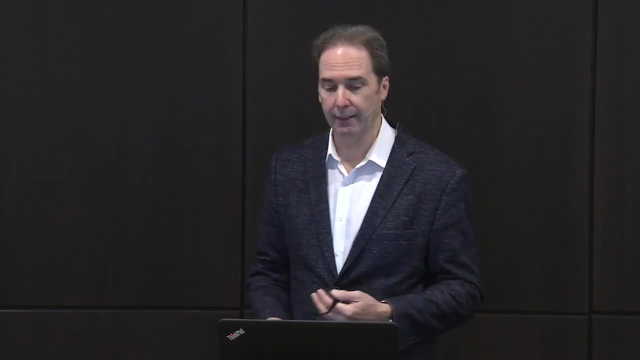 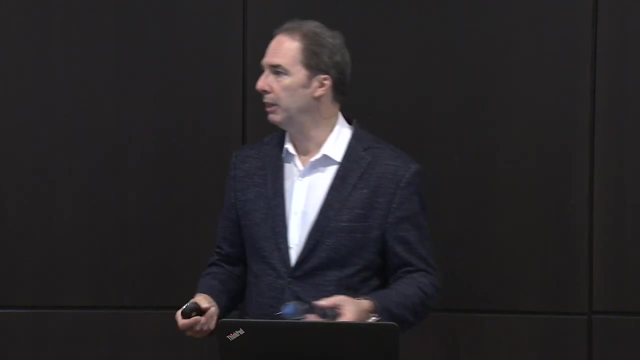 We've never thought about What's below ground And we don't have data for that. So I want to talk about how this might relate to the paired watershed approach generally and what this might mean for forest water sustainability. So this is now the roadmap going forward. 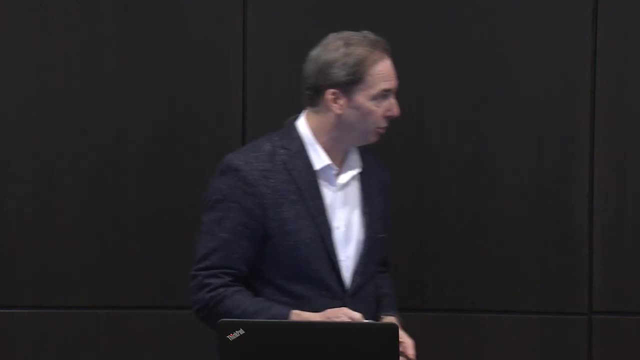 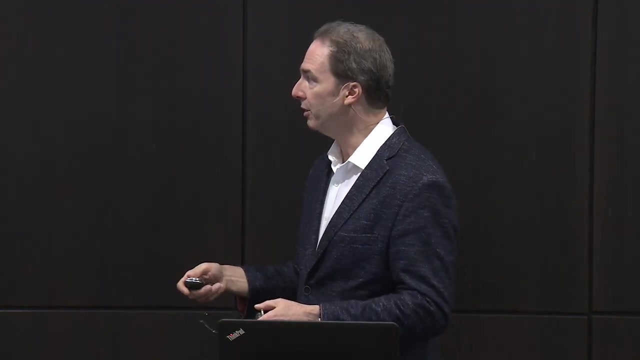 So let me give you a little bit of background, just because I know I'm not talking to a group of forest hydrologists. What do we do? Well, in most of these studies, again, they're in the headwaters. We measure precipitation and runoff. 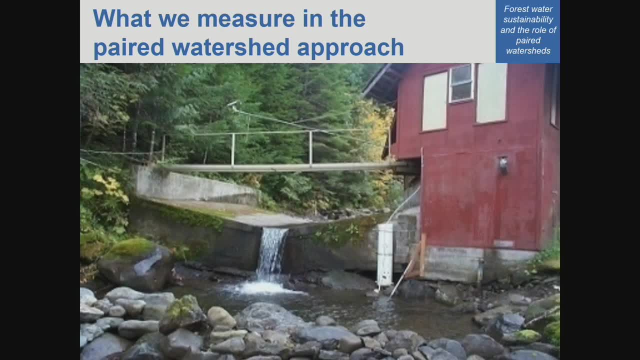 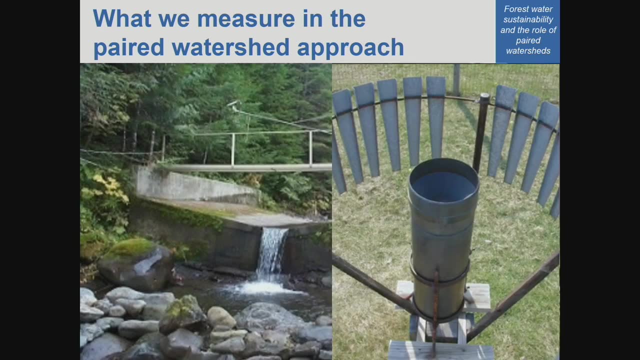 Here's a very fancy runoff measuring station. This is at another long-term ecological research site in Oregon, at the HJ Andrews. So we're recording the stream flow And we measure precipitation in various ways. If it's snow-dominated, we're using snow pillows and things. 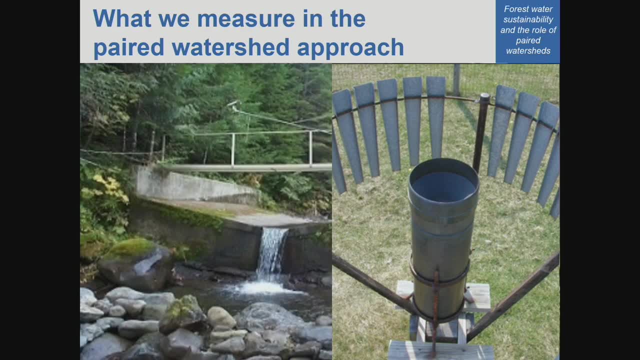 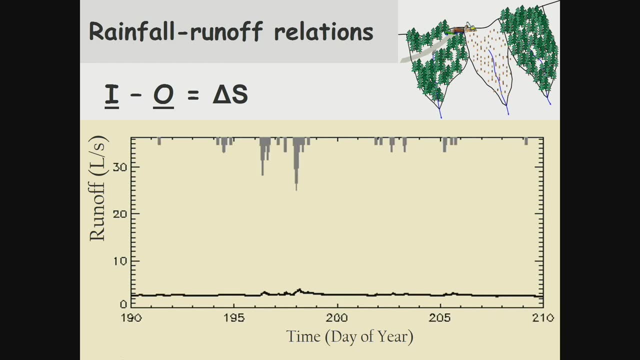 If it's rain-dominated, we're using various types of rain gauges And with these data we do the classic water balance. Again, this is hydrology's most basic equation: Input, which is precipitation minus output. Input, which is stream flow or evapotranspiration. 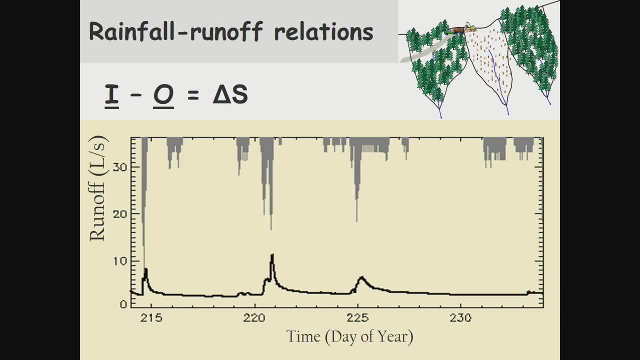 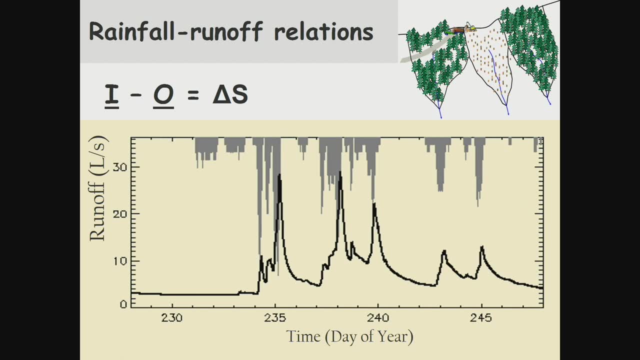 equals change in storage. We think of this in a long-term steady-state mode, So we never think about the change in storage. Here's an example of what these data often look like. You're seeing a scrolling plot. This is day of the year. on the x-axis. 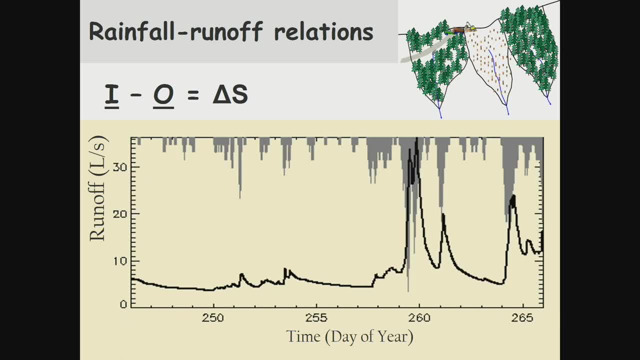 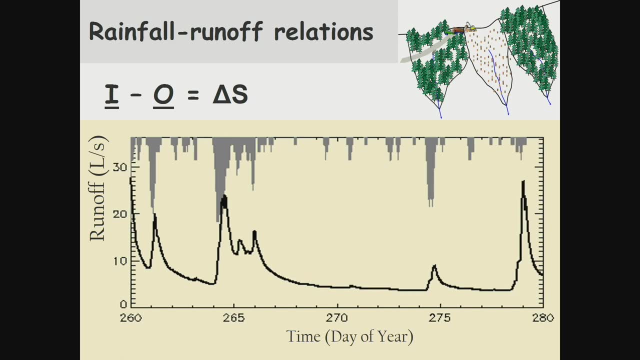 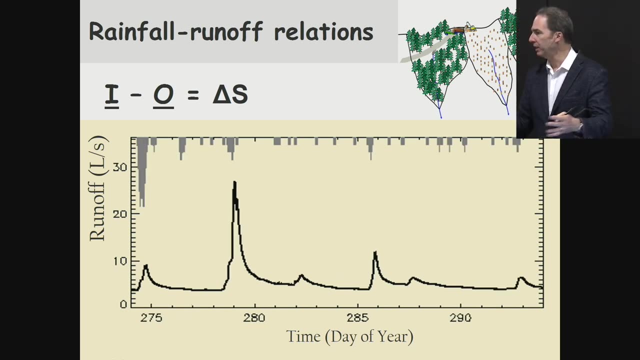 On the y-axis. you're seeing runoff in the solid line In response. this is a small headwater, forested catchment in southeast Alaska. You're seeing the stream respond to these rain events And it's these changes in response, whether it's during events, monthly, seasonally, annually. 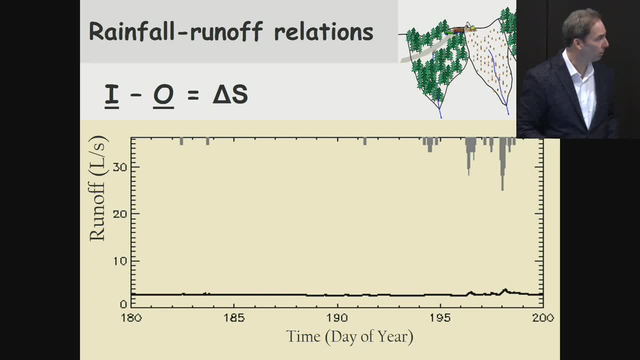 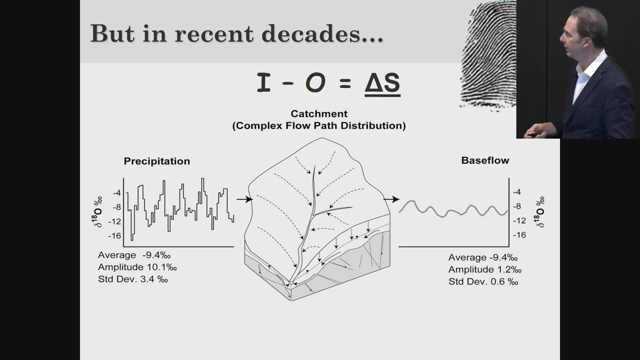 this is really what's at the heart of this whole paired watershed approach. Now there's been a technique that's come into vogue in recent couple of decades, And this is still going after the watershed, using the watershed as the basic unit. 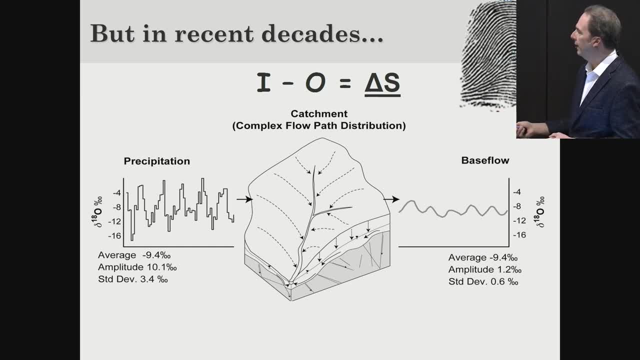 But it's tracing the water molecule And this is isotope hydrology, And some of you have heard things about this. Basically, it's a fingerprint of the water, So you can almost track the raindrop through the forested watershed. So here's our watershed. 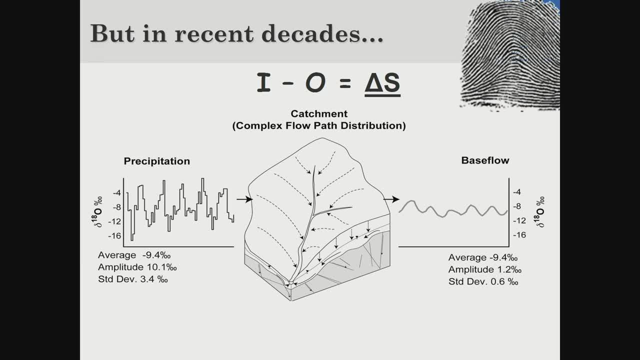 It's shockingly devoid of trees, I guess in this diagram. But on the left-hand side you see a time series of precipitation isotope composition. It's covering a period of seven years or so. It's negative in the winter. 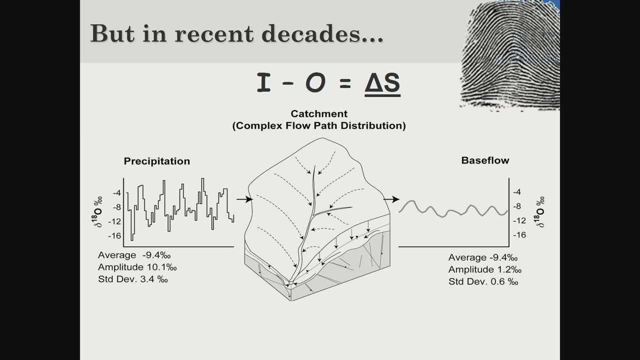 It's more positive in the summer And you get this nice cyclic input. And on the right is what you see. you'd sample from the stream in the form of base flow, a water sample you'd take when it's not raining, And what it shows is a lagged and damp version. 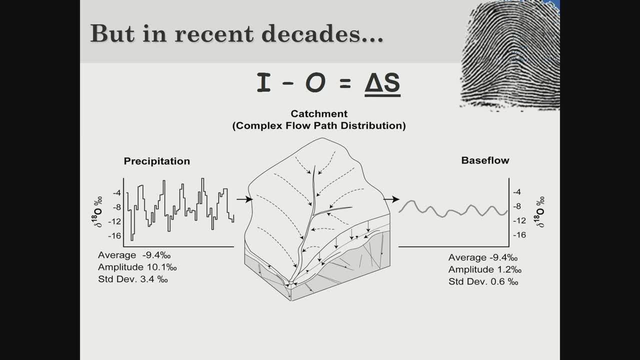 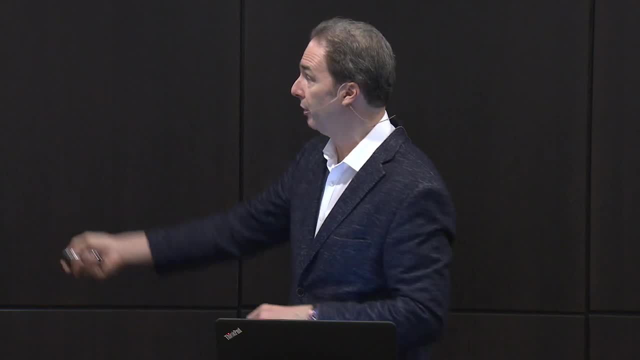 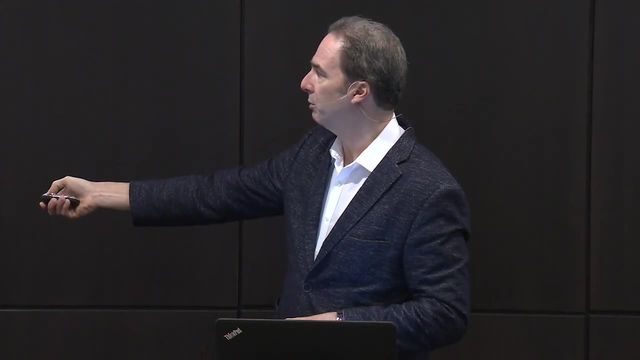 of that input on the left. So the watershed is filtering this input And the amount of that filtering really is defined by how much storage there is. So if this was a parking lot on the surface of this watershed- the Costco parking lot, then the right-hand side. 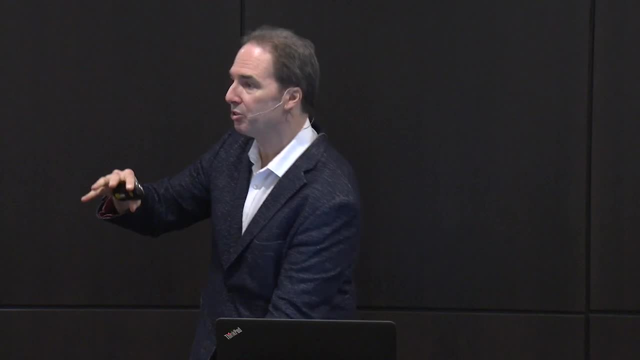 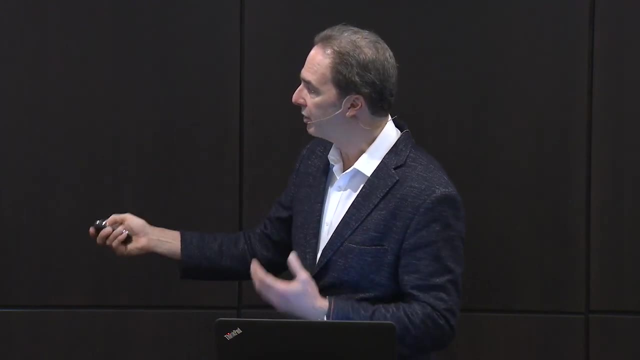 would look identical to the left-hand side, And if it was an infinitely deep sand tank, maybe it'd be a completely flat line on the right side. But this is a different type of information And it's giving us some insight into storage. 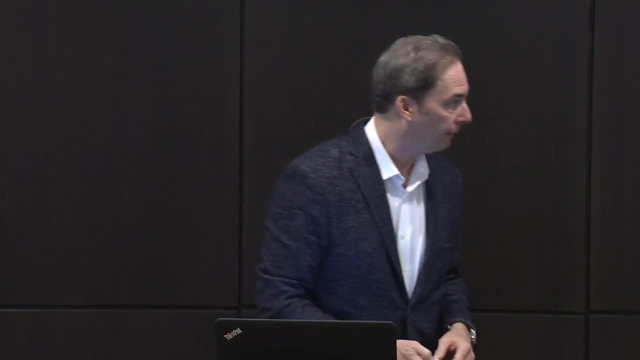 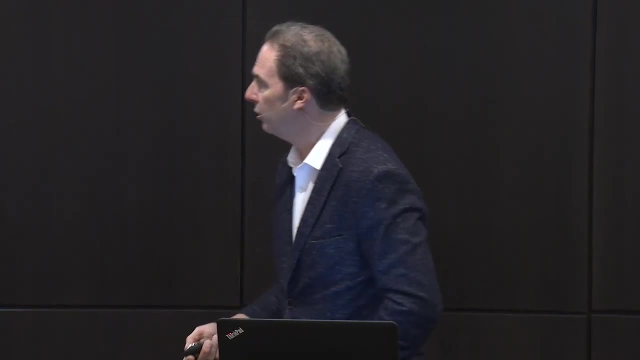 the thing that the rainfall runoff relations don't really do, And let me illustrate this with some data from a field site. This is a site in Scotland where I've been working with Dorte Tetzlaff and Chris Soolsby. some of their data: 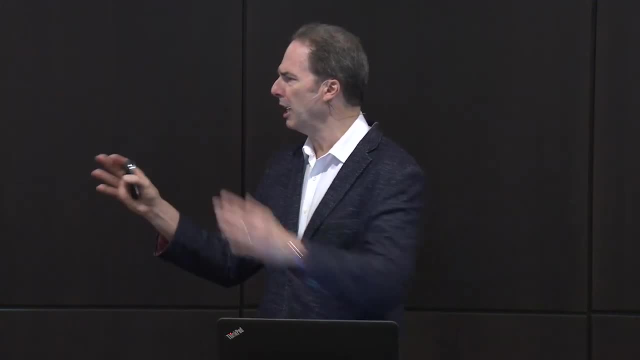 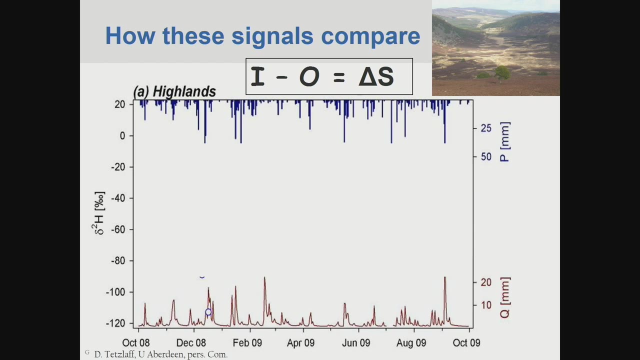 You're seeing about a year's worth a year of time on the x-axis And this is the rainfall runoff relation for this very wet response of Scottish site in the Scottish Highlands. But if you look at the isotope data that go with this, 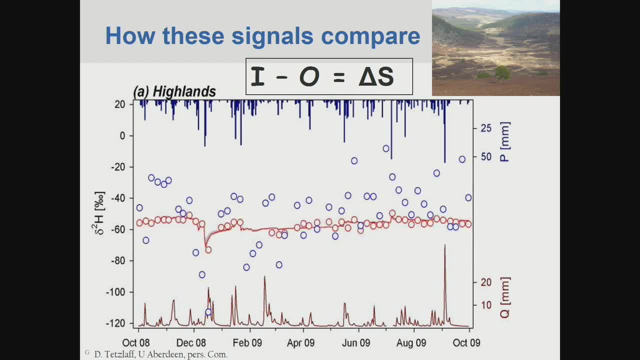 you see really quite a different picture. The blue, so the blue, of course. up top is the rain hyatograph coming in. It's raining all the time. If you've been to Scotland on holiday, you know it's raining every two or three days. 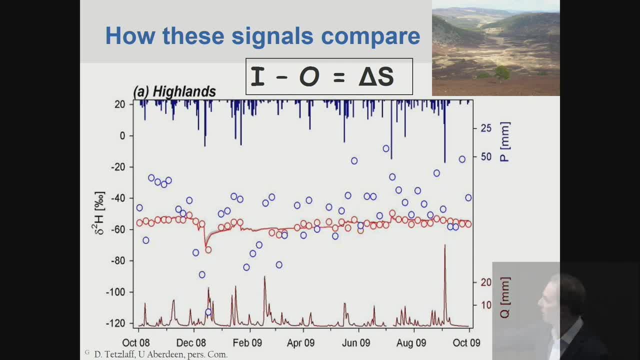 in the Highlands And you see, with each rain event you're getting a runoff response along the bottom. The blue dots now are the isotope compenetration of the rain and the brownish dots are the isotope composition of the water in the stream. 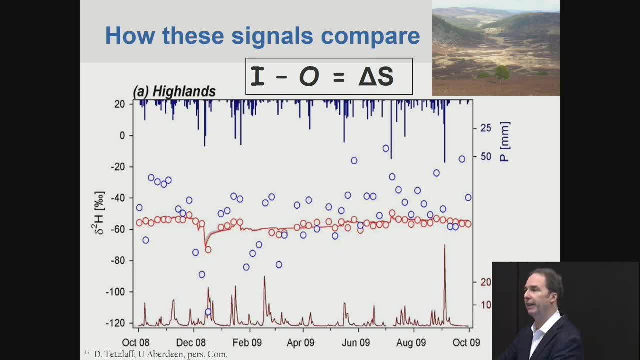 So very lagged and damped, very flattened, And this is suggesting, then, that the water in the stream is not yesterday's rain. It's much older water, It's water that's had some mixing in that tank. that is the, the watershed. 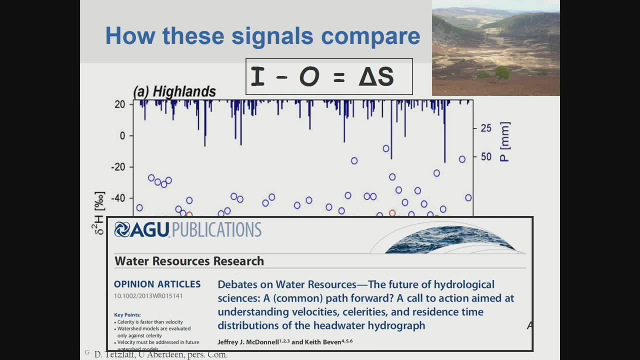 And Keith Bevan and I have been writing about this a little bit. This was a Debates article a couple of years ago, really trying to make the case for the differences between these different signals. The celerity of the hydraulic potentials as illustrated by the rainfall runoff response. 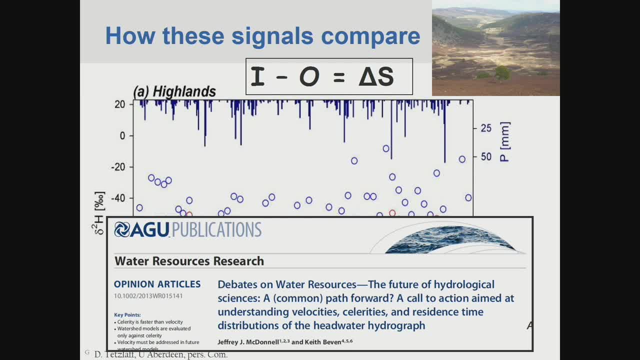 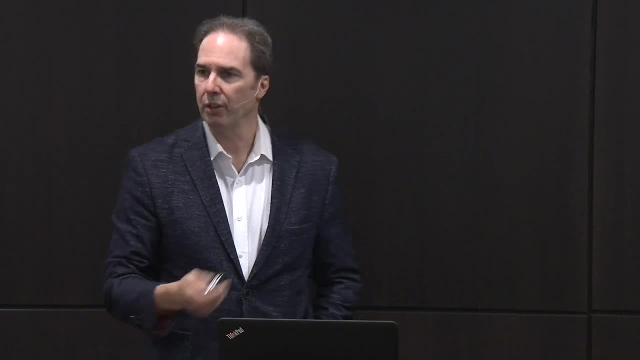 kind of a fancy way of saying the pressure propagation through the landscape versus the particle velocity, if you like. as represented by the tracer, These are two very different signals In the context of the forested watershed. what all this means is that the water in our streams 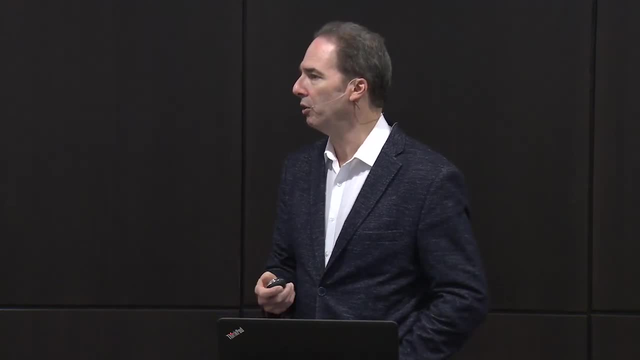 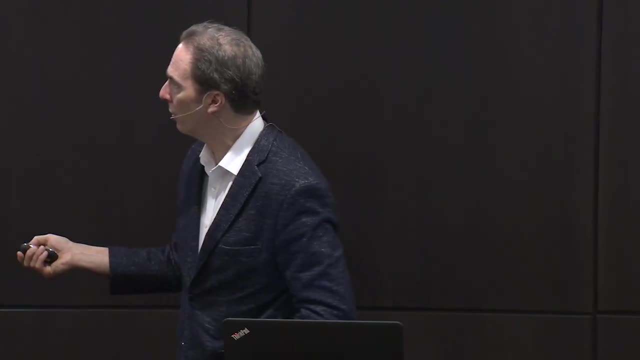 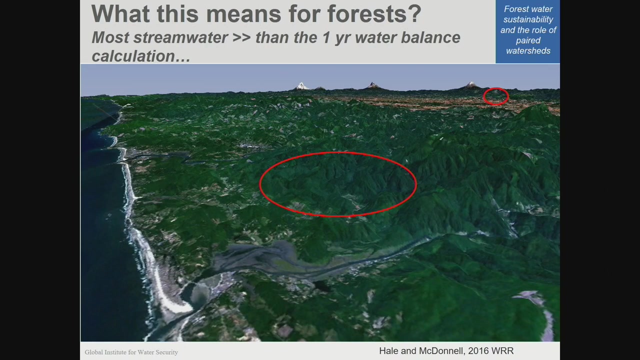 So already there's a bit of a problem. Let me show you this for two watersheds in Oregon. one in the coast range on the left-hand side. So Oregon is just one state above California, Pacific Northwest, a little bit down from British Columbia. 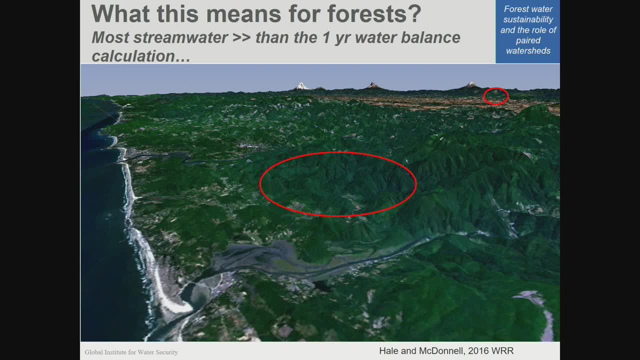 On the right-hand side, the smaller circle. this is another set of catchments. These are paired watersheds, They're called watershed studies and they're in a different geology. You might already guess it's a volcanic terrain. So up here on the right-hand side it's a more tight volcanic bedrock. 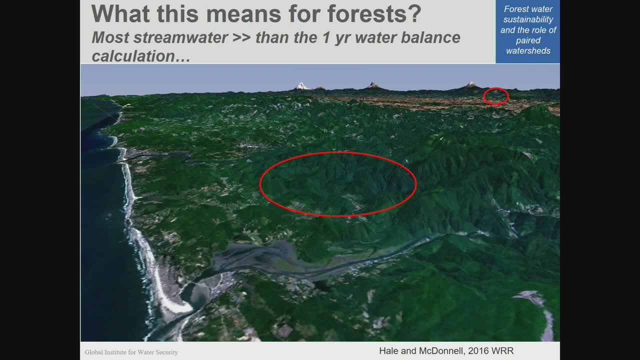 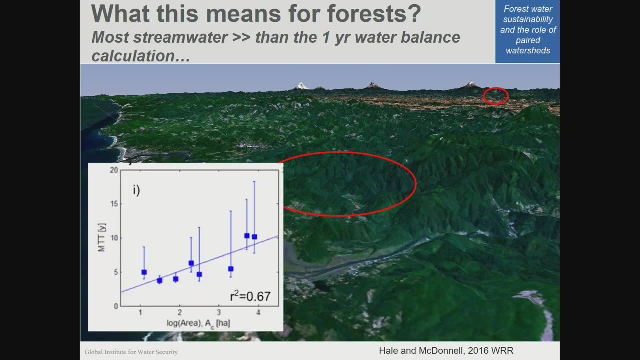 whereas the bedrock on the left is more of a permeable coastal sedimentary rock. So let's look at some data. These are eight catchments that we gauged kind of headwater catchments, ranging in scale from about five hectares to a couple hundred hectares. 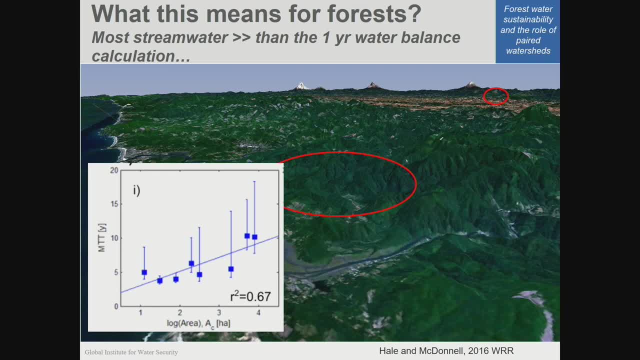 And on the y-axis is the mean transit time. Mean transit time is kind of analogous to the age of the water and it's a measure of how damp that isotope signal was. So the more damp, the more flattened. the older it is, the higher the mean transit time. 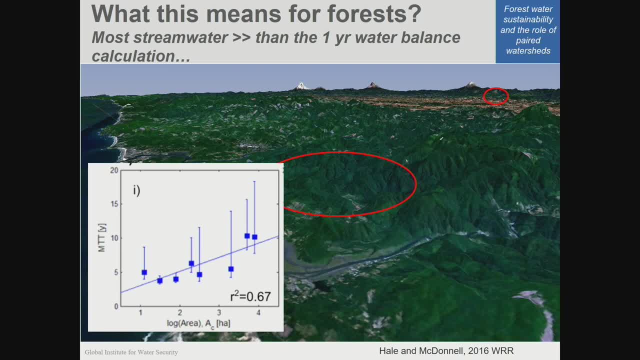 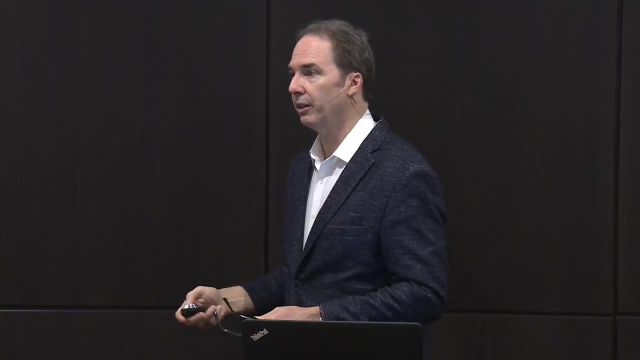 So the first thing we see is that these streams are ranging in age from about oh, four to ten years old. That's the mean age of the stream water, And it's scaling with area. So the bigger the watershed, the older the water in these forested streams. 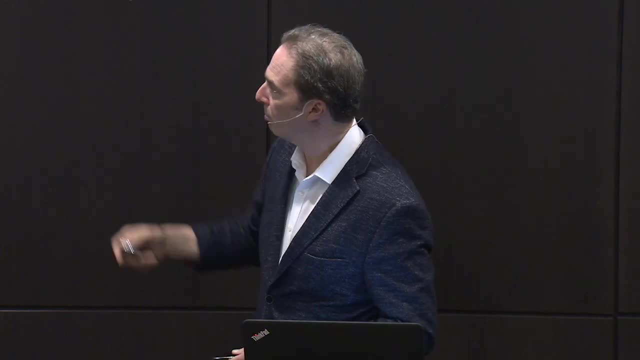 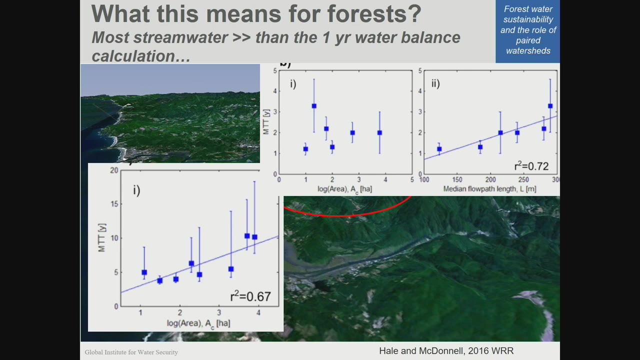 Over here in the tighter geology. if you just look at the left plot, what you see is transit time again versus area. In this tighter geology we see no relationship with area of the watershed and the water is much younger. 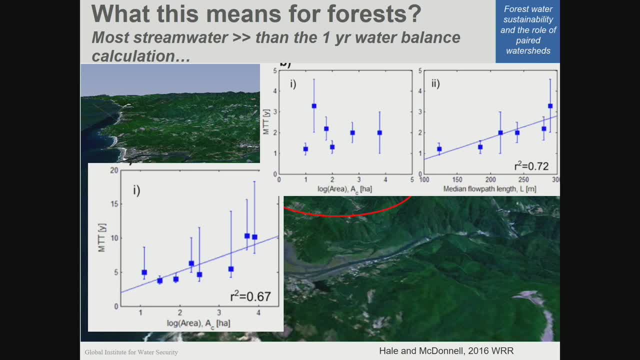 You can see for these watersheds. these are ranging from about ten hectares to 60 square kilometers. They're ranging from maybe one to three years old, And then the upper right plot there is just reorganizing these data and showing that it. 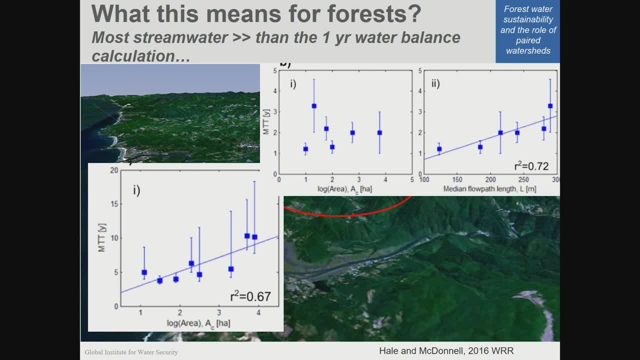 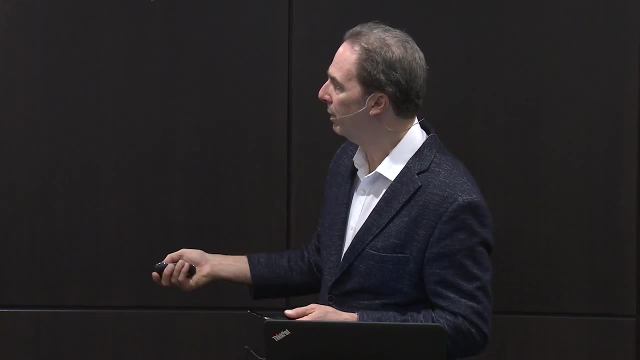 actually is really influenced by the topographic structure, meaning how steep the slopes are, how long the slopes are, is explaining 70% plus of the variance of these residence times. What all of this means is that if we go back to this map, all bets are off. by looking at 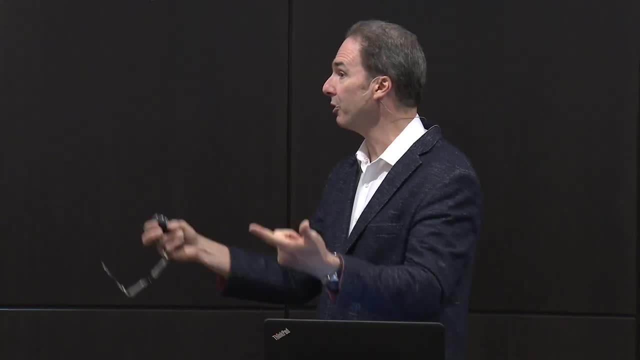 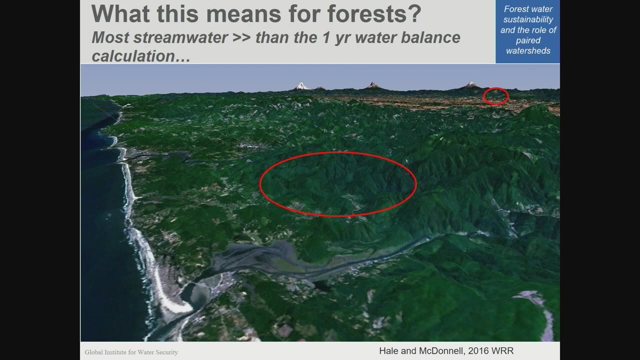 a rainfall runoff hydrograph A, how old the water is and how it varies across the landscape. And this is a great illustration of two sites with almost identical rainfall runoff response. very similar climate. The only difference is how permeable it is. what's below? that's conditioning the age. 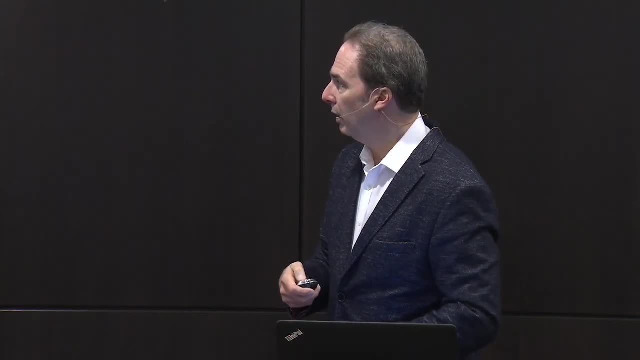 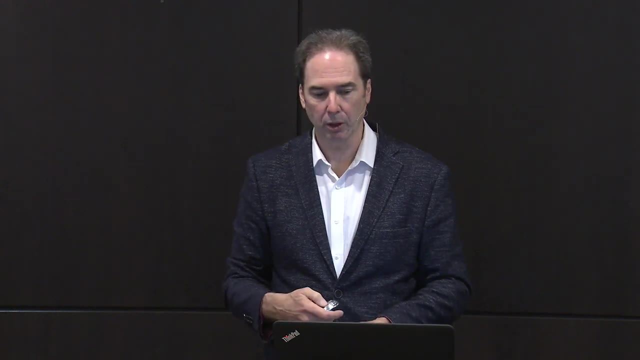 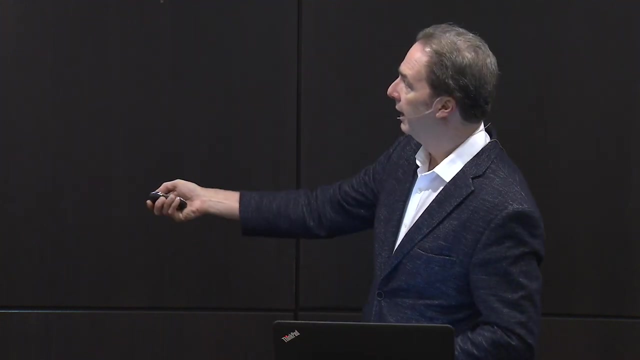 of that water. Well, what does this mean for forest streams and storage- this possible issue that could be at work. Let's go to Luxembourg. This is a place where I've been for a long time. This is a place where I spent last winter working with a colleague there, Laurent Pfister. 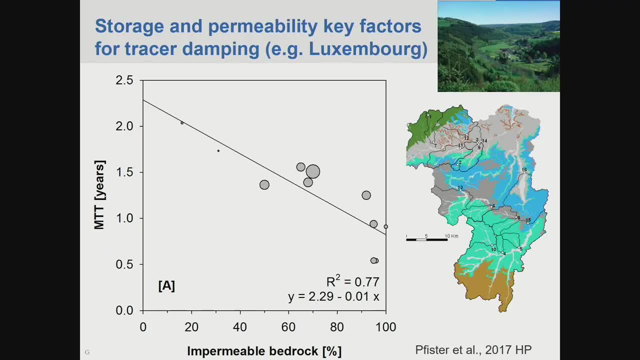 The forested landscape. the beauty of this site is that each of these colors you see on the map on the right is a different geology. These are clean and mixed expressions of different rock types: sandstone, marl, schist and these. 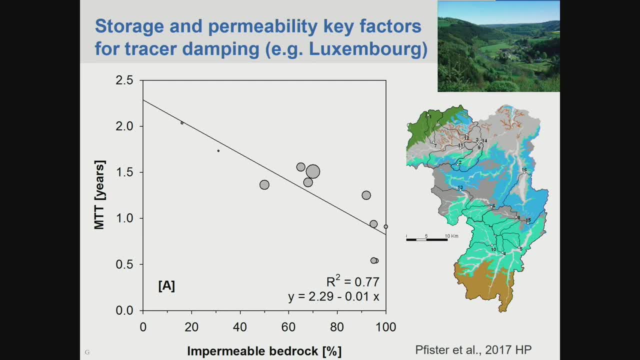 are rock types with different permeabilities. So on the x-axis you see kind of a permeability measure and on the y-axis you see this again: stream water age. This means transit time And what you see is a really strong relation between how permeable the bedrock is and how 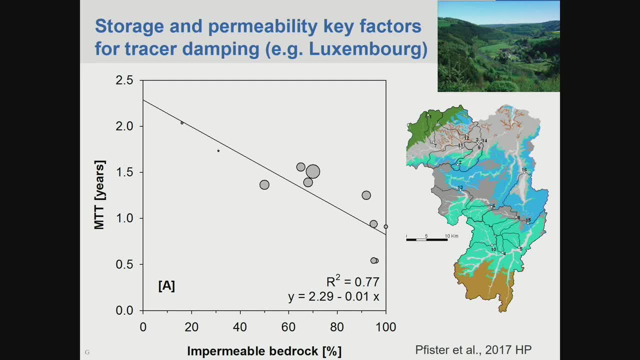 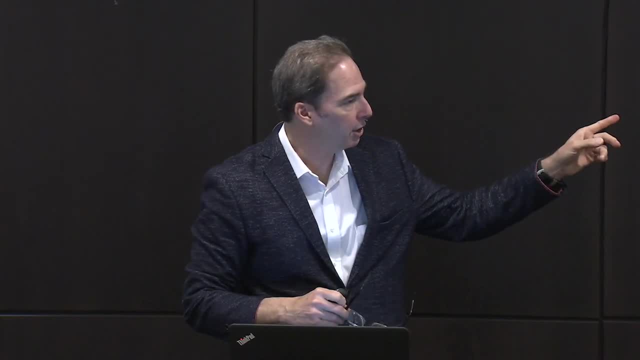 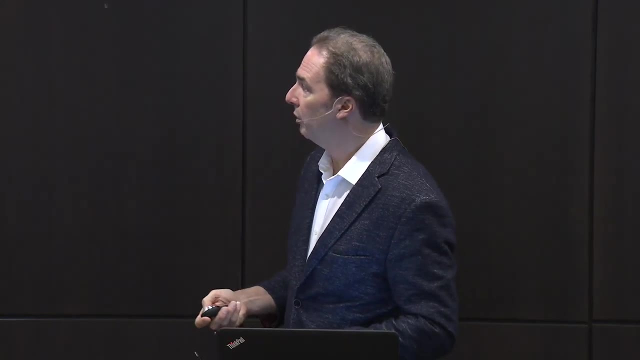 old the water is, where the more permeable the bedrock or less impermeable the older that water is. And you see a small dot in the upper left there on the plot. the size of those dots are scaled to how much flow is coming out of the basin during the sampling. 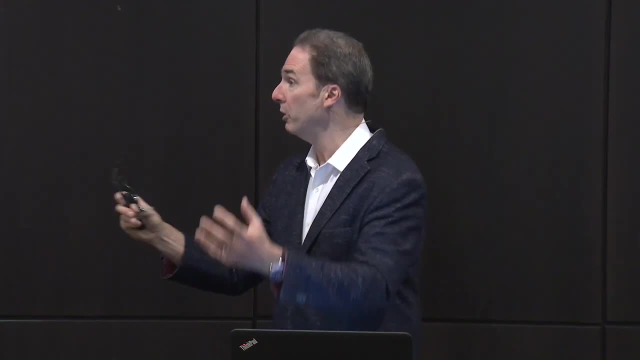 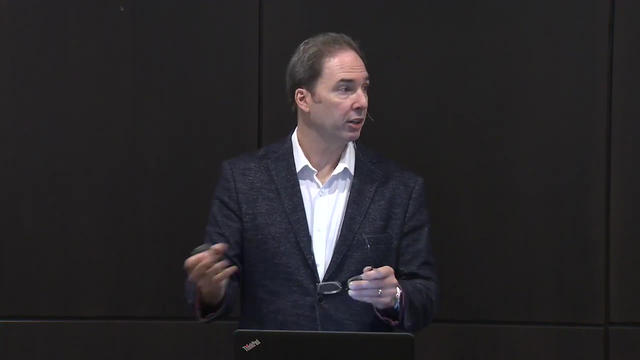 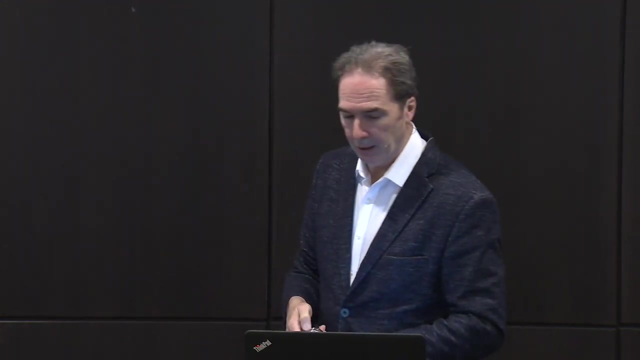 So this is suggesting, then, that not only, like in Oregon, we see these different relationships, different ages. This is based on: is it permeable or is it not permeable? the volcanics versus the sedimentary? Here we can dial in it even more and relate it to really the relative permeabilities. 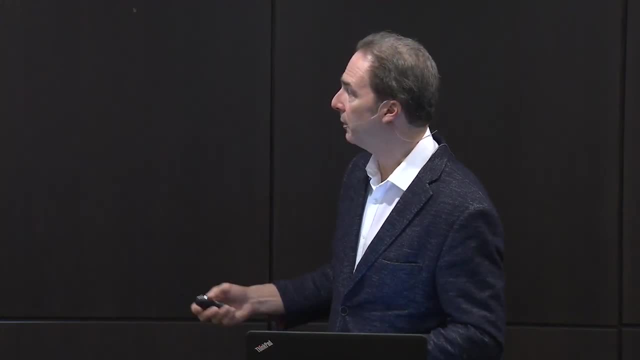 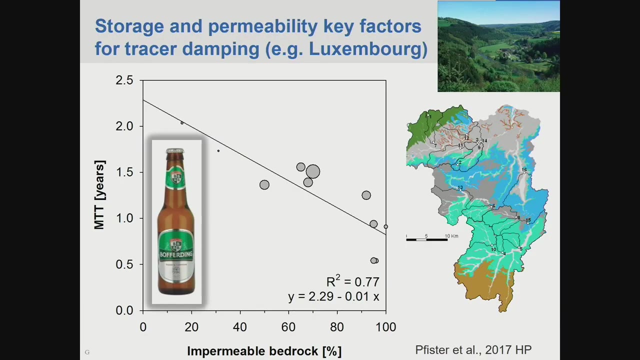 One interesting thing: I was working with a brewery in Luxembourg. there's a whole back story to that, but this beer they draw from the same sandstone, aquifer, as you can see in blue here on the right hand side, And this beer they've done carbon 14 age dating on the ground. 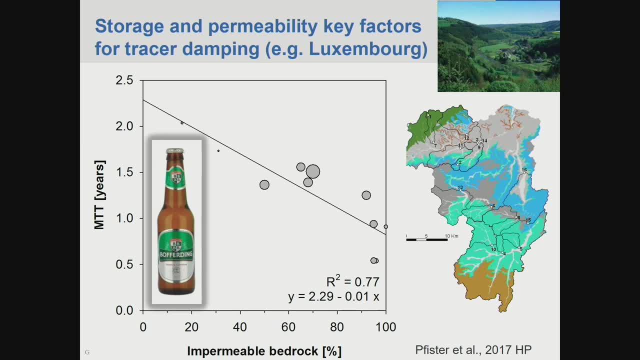 And they've done carbon 14 age dating on the ground And they've done carbon 14 age dating on the ground And they've done carbon 14 age dating on the ground. So this beer is made with the ground water and the water is 27,000 years old. 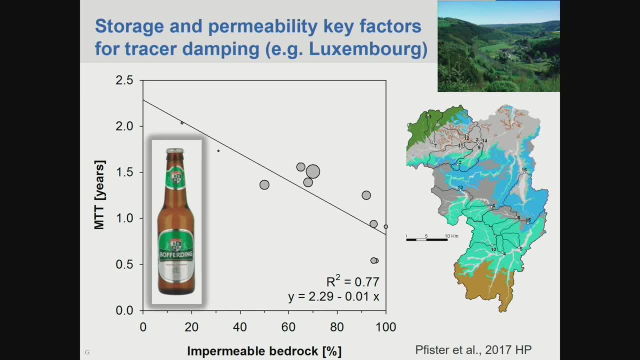 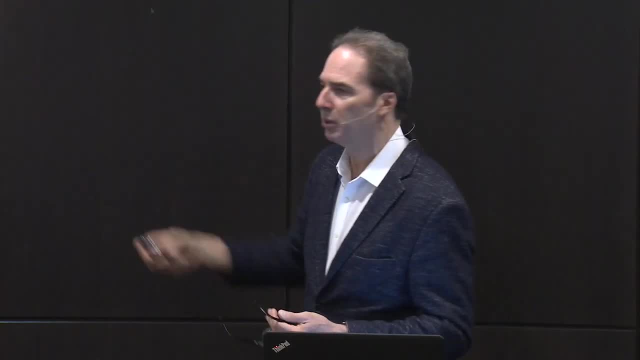 So this beer is made with 27,000 year old water. The question is: well, if the beer is 27,000 years old, being drawn from a deep aquifer in that sandstone, why is the stream so young? And this is an issue, almost a fatal flaw with the stable isotopes. 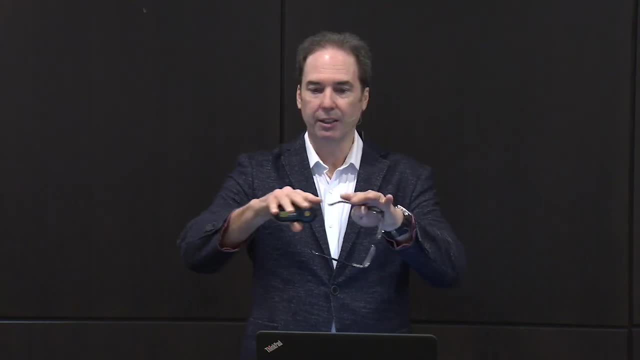 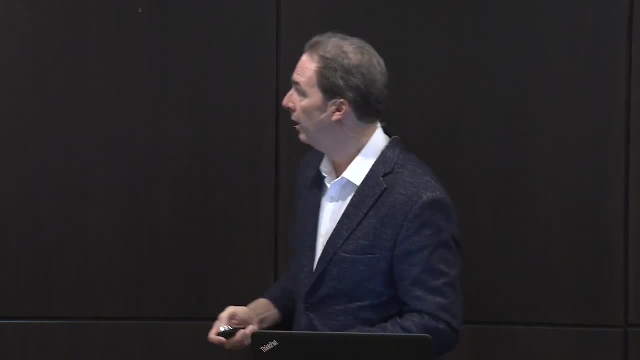 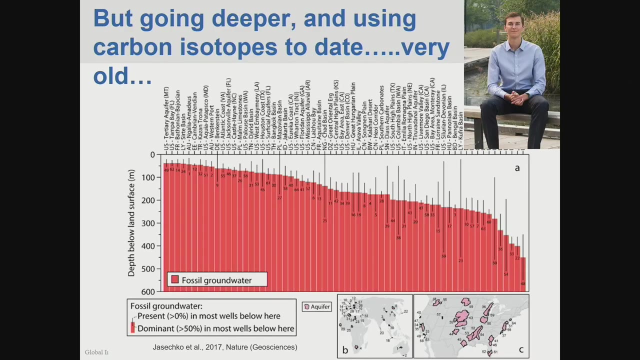 So you need to use other isotopes. So you need to use other isotopes, tope tracers, if you like to get at some of these ages. Scott Giusecco has done this with a global database he's assembled And you see some of the sites where. 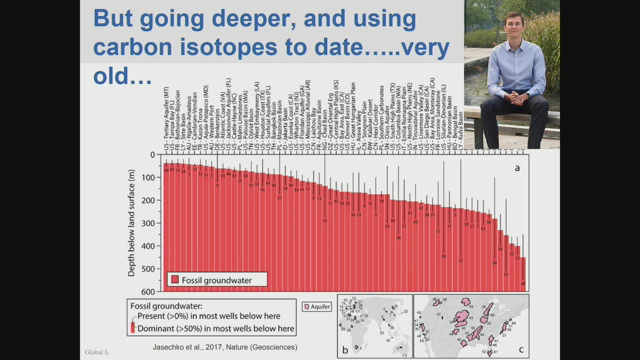 he's extracted these data. Scott was a postdoc here briefly before he went off to the University of Calgary and now he's at the Bren School at UC Santa Barbara. This is a very nice analysis he did. Grant Ferguson was also involved in this paper. 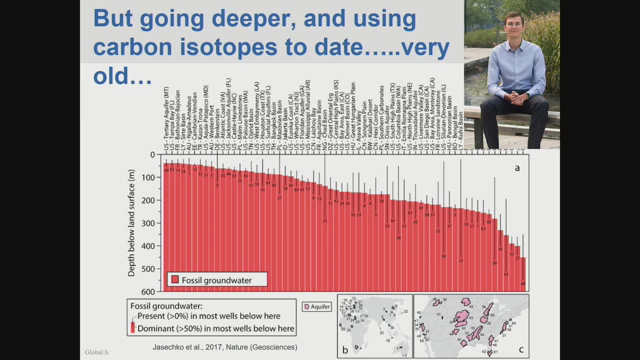 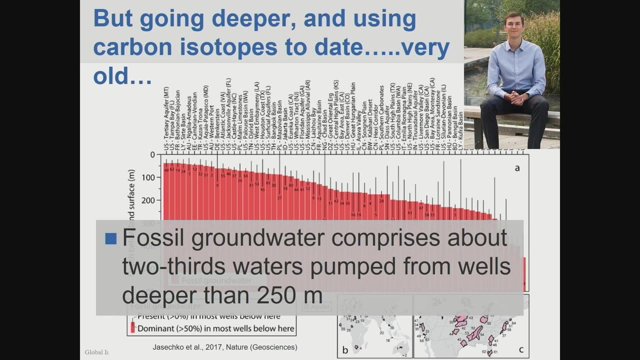 And you see some of the study sites along the top, there above And on the y-axis. what you see is depth below the ground surface and this measure of a thing called fossil water And what the punchline of this paper was, that this fossil water, that is, water older than 10,000. 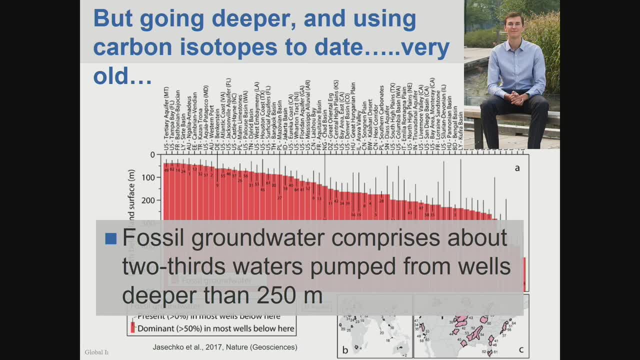 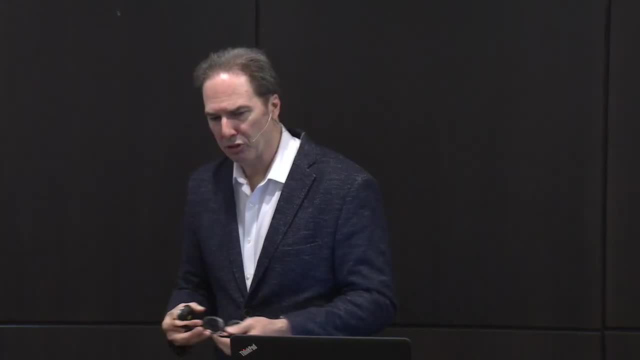 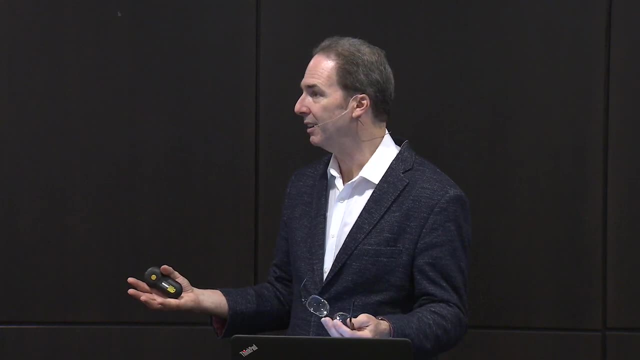 years is representing about 2 thirds of the water deeper than a couple of hundred meters. Maybe it's not so surprising that things get old when you go deep, But you know, in steep forested catchments a couple hundred meters is not a lot of relief. 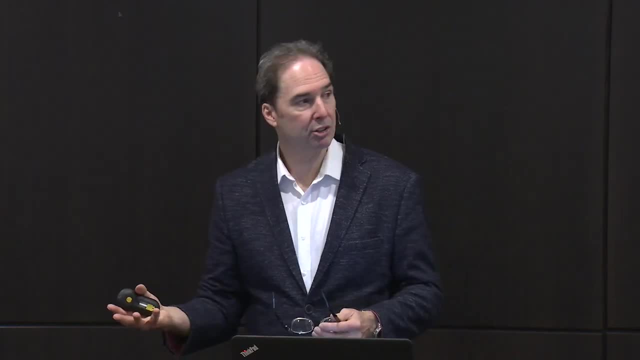 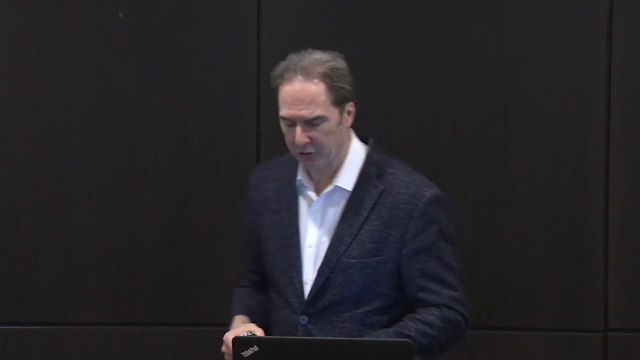 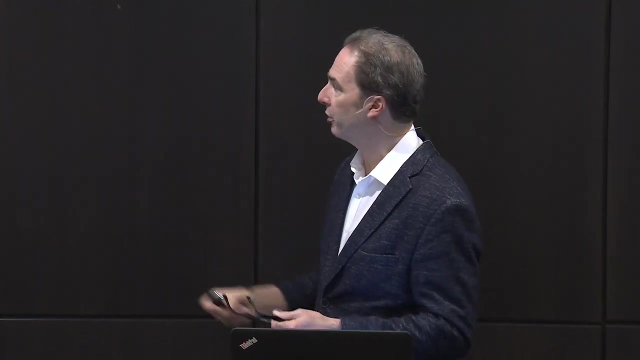 This is quite old water And we're talking about streams that are relatively young. Let me show you one other bit of analysis Scott did when he was during his postdoc, supported by CCRN. This was of streamflow age. This is a separate study. 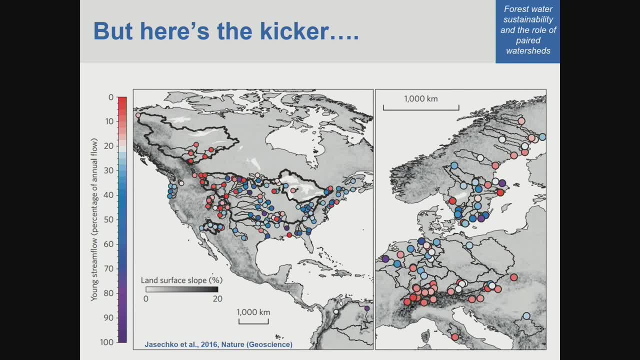 And he was able to amass streamflow isotope data, mostly from the US, but also a bit in Canada, some in Europe and elsewhere, and was able to ask the question: well, how old is this global streamflow? And what he found was that, if you 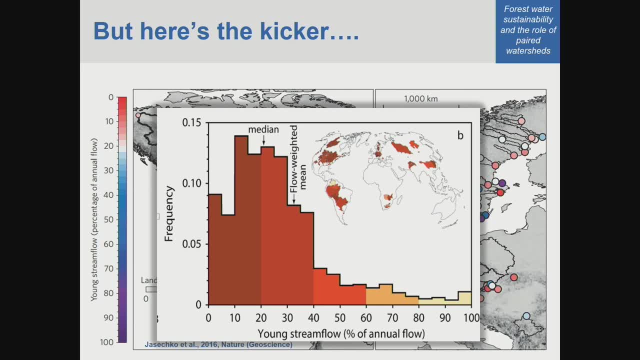 look at the distribution of these data in terms of frequency on the y-axis and the age of this water in the stream and young streamflow we defined here as three-month-old water. This is using a technique that I won't go into details on for this presentation, but about a third of global streamflow. 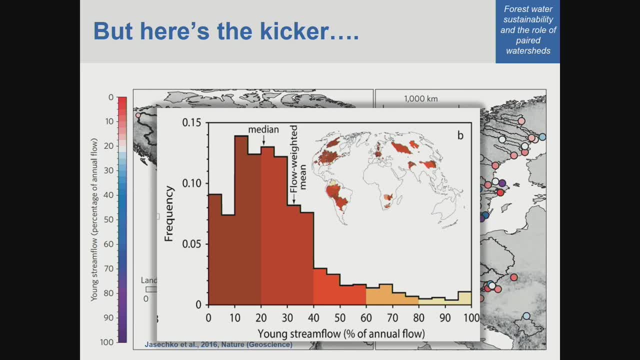 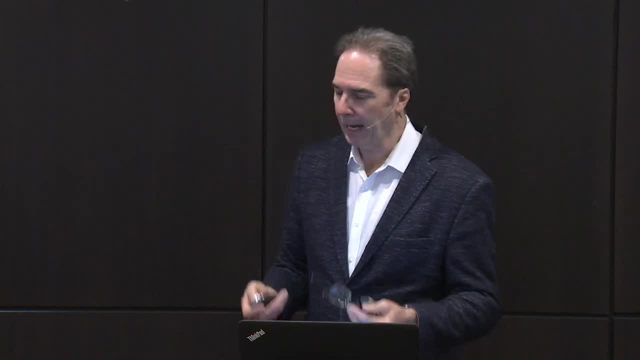 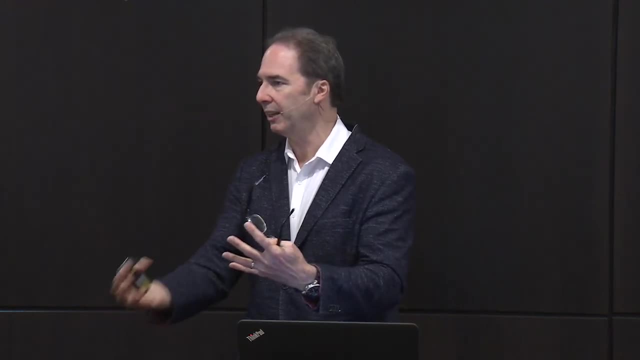 global meaning from these sites, for mostly forested watersheds, was three months old or less. So what we have is a really almost bimodal distribution of water ages. You've got little bits of super old water trickling in forming a long tail of that transit time distribution. 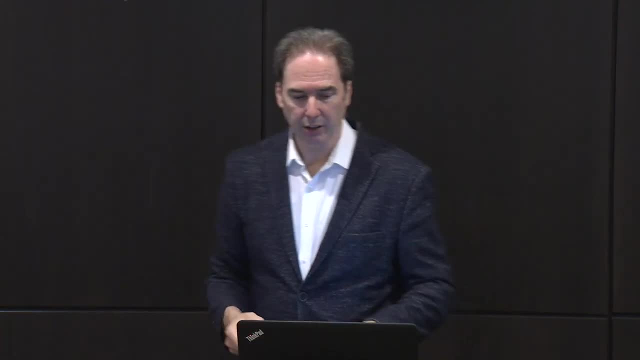 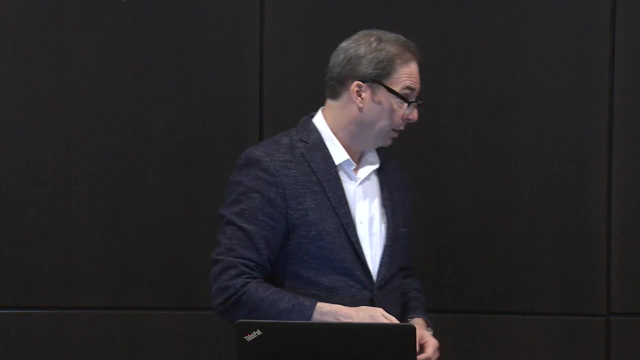 and a significant amount of this younger water. If this is a research area that interests you, there was a paper that came out a couple of months ago by Wouter Burgess and Jim Kirschner that really did a great job at explaining these contrasting ages. 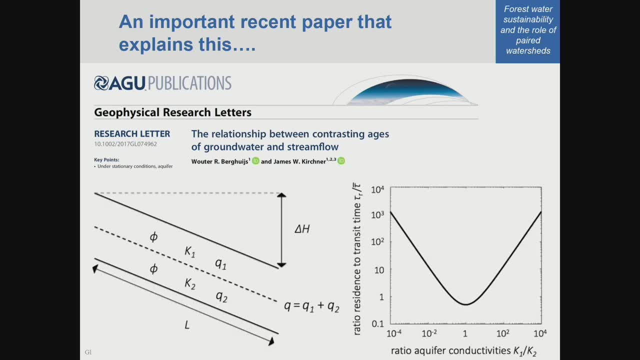 between groundwater and streamflow, And I'll just tell you this before I move on, in case you're interested. It really boiled down to permeability contrasts between the shallow soils in a forested catchment and what was below in the form of bedrock. 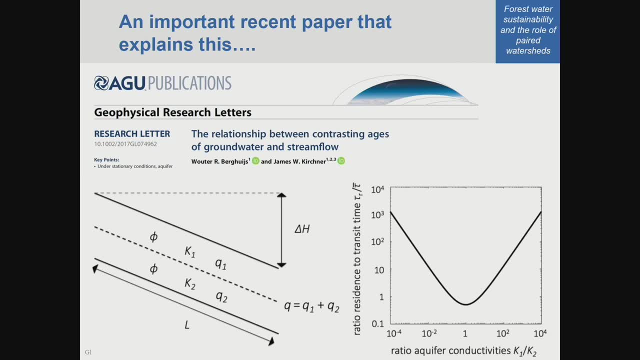 And this plot on the right. so the plot on the left is showing you these two layers, if you like, And the plot on the right is showing, on the x-axis, the ratio of aquifer conductivity. So the shallow and the deep is a small or a big contrast. 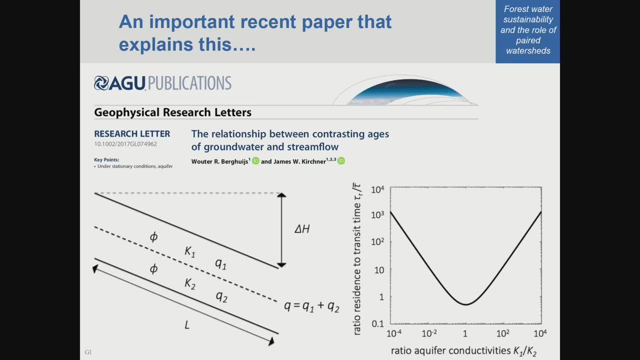 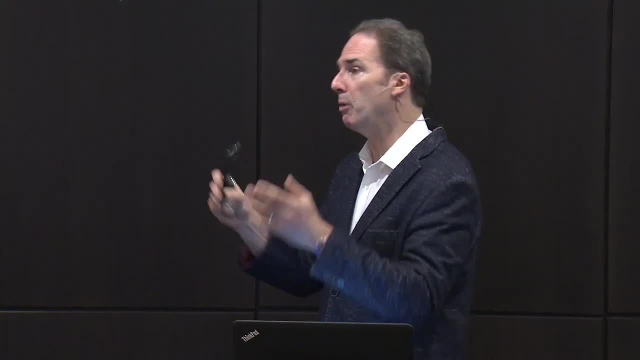 And then on the y-axis, is this ratio of residence to transit time, meaning what's in the ground, the residence time- versus what's in the stream, the transit time. And if you have big contrasts, what that means is you have then a big difference. 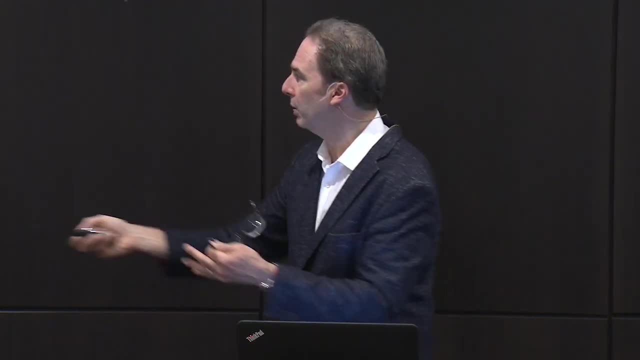 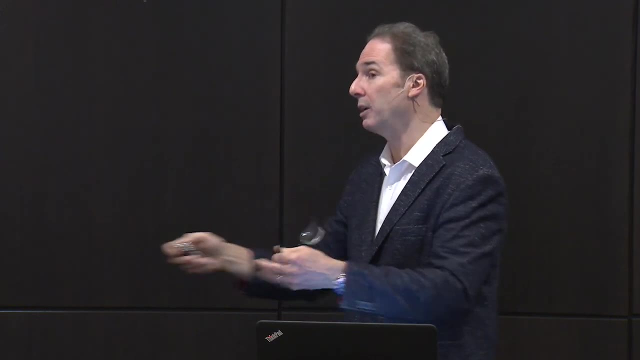 in the ratio of the two Or if they're very similar, they're very similar. let's say you have the soil and the bedrock having identical conductivity, then the two ages or the residence time and the transit time will be very similar. Anyway, a level of detail that maybe you're not interested in, but if you're studying this, I found this paper particularly helpful And it helps to explain the beer issue in terms of why you'd have such old water in that sandstone aquifer when the water in the stream. 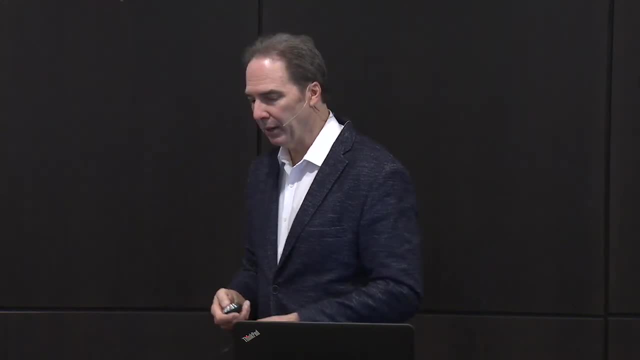 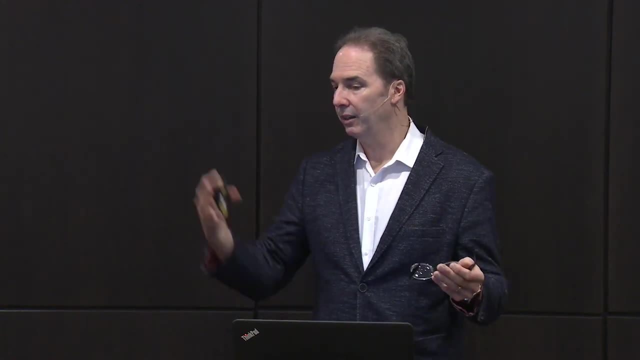 is so seemingly young. All right. so we've talked about stored water. We've talked about the fact That the water in the stream is old, certainly longer than the annual drumbeat of the paired watershed analysis we often do. What else uses this stored water? 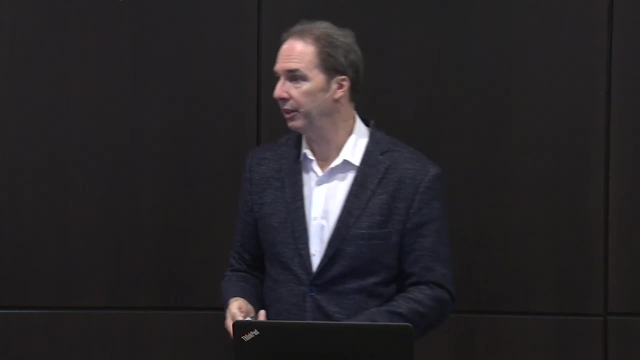 Well, of course, the other half often of the water balance equation is transpiration. There was some really important work published by Todd Dawson, who's now at Berkeley, back in the early 90s. This was a paper that caused a lot of stir: stream-side trees. 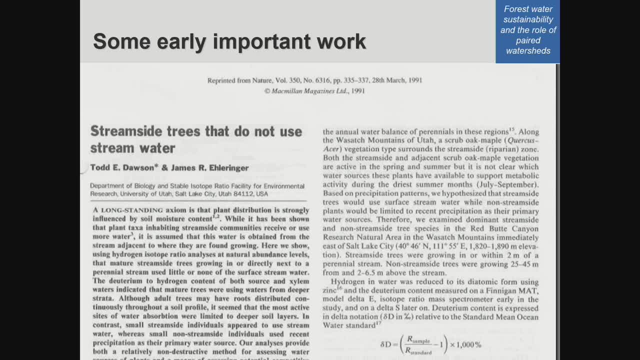 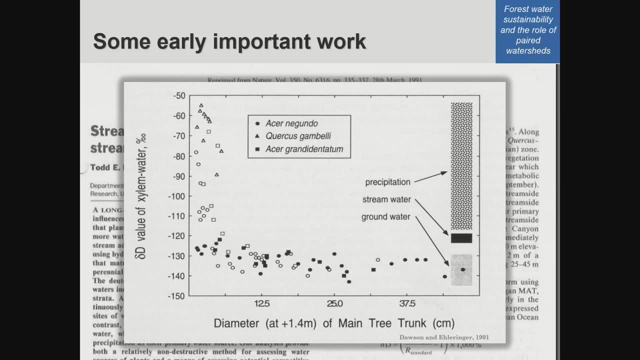 that do not use stream water. This was really one of the first. Most of the uses of stable isotopes ask where trees get their water. So, looking at this plot, you're seeing stem diameter on the x-axis And on the y-axis is the isotope composition of the water. 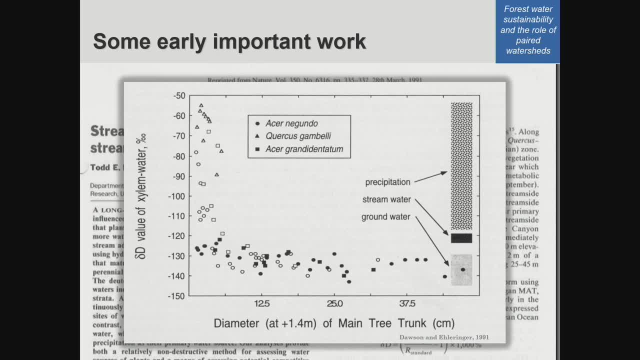 that they're sampling here On the far right. you're seeing what the range of precipitation is. Remember precipitation was like a sine wave going up and down. It's covering a range. You're then seeing stream water in black and groundwater below. 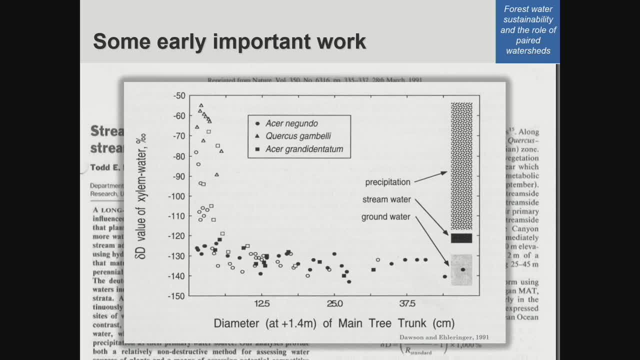 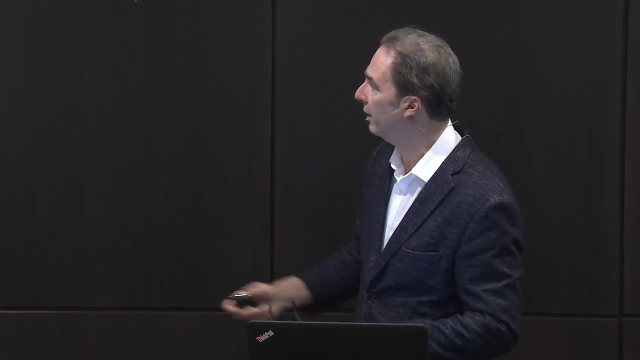 So what was this? What we see on this graph and what they were able to really excite the community with, is that, by sampling different vegetation when it's very young, when the stem diameter is very small, those trees were going after what seemed to be rainwater or very shallow water. 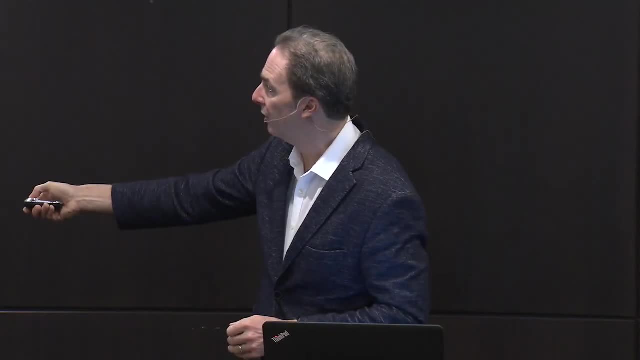 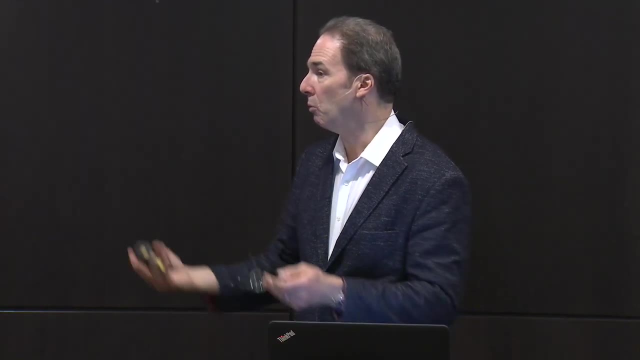 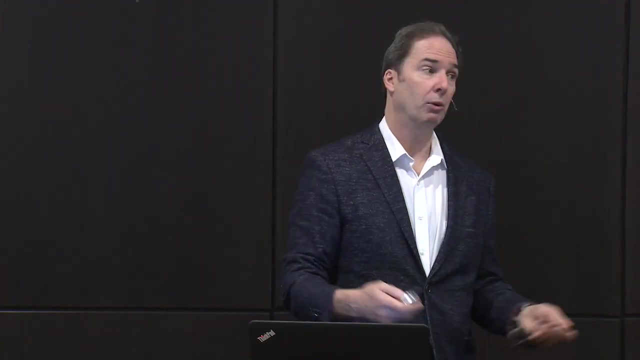 And as they got bigger they put roots deeper. they're switching their sources, basically from rainfall to more of a groundwater supply, a groundwater source. And this was a real shocker because these trees were sitting next to the stream and the ecologists at the time thought, well, surely they're going to be taking something. 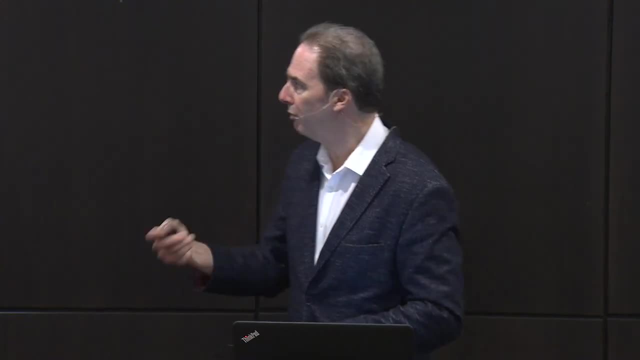 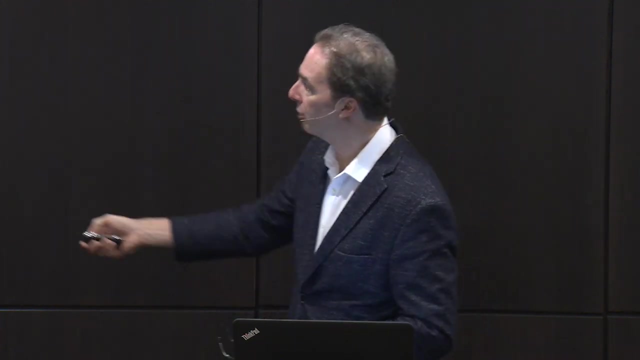 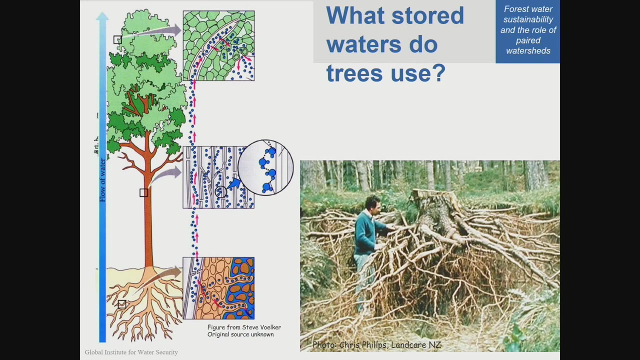 that looks much more like stream water. This field has evolved a lot over the intervening years. That was early 90s, Fast forward- and there have been hundreds and hundreds of papers published looking at where trees get their water using stable isotopes. So the idea is just like a stream in the watershed, a proper stream, you can sample the water. 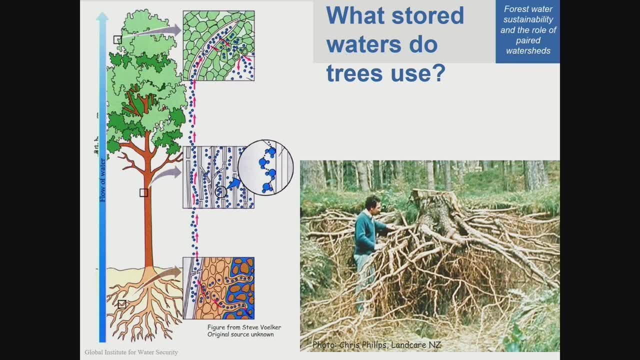 from the xylem stream, if you like, in the tree, and you can extract that water and relate it to its water source in the root system or with depth in the soil profile. And, as you can see, forest soils are really a dense network of these roots. 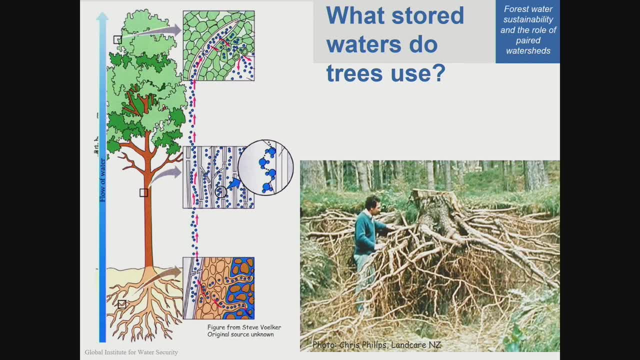 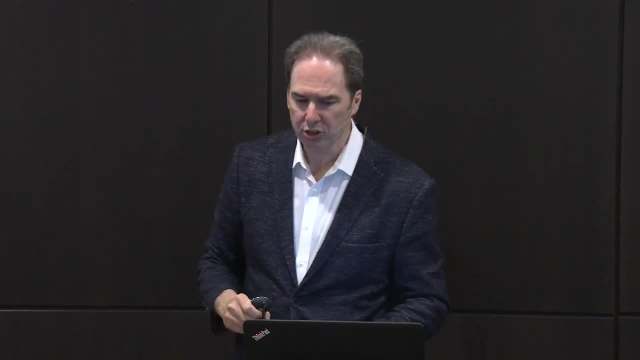 This is some hydro exposure of roots from a group in New Zealand at Landcare And what I want to ask the question now is what stored water do trees use? And what we've realized in this intervening period is you really just can't use one isotope. 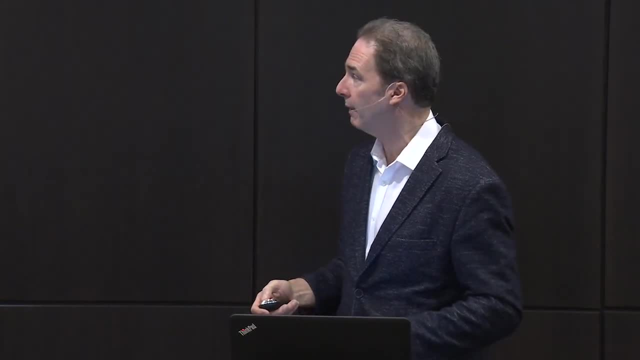 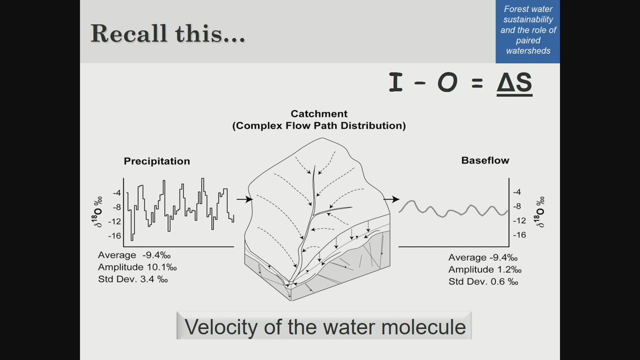 to get at this question You need to use both isotopes together. So remember I showed you this. This is that diagram of the rain input on the left and the lagging and damping of the output of the streamflow in the watershed on the right. 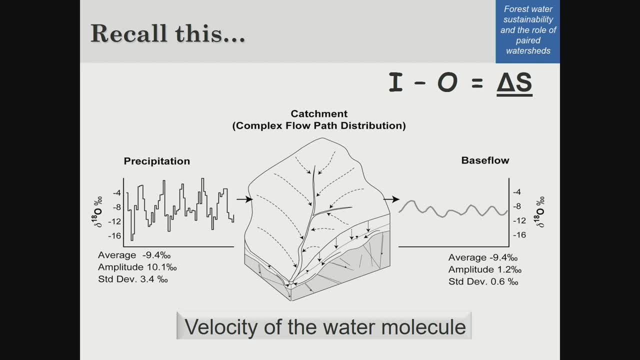 Well, this is just one isotope, O18.. We can look at O18 and deuterium together. These are the two stable isotopes of water, Okay, And we can see these same patterns now in so-called dual isotope space. 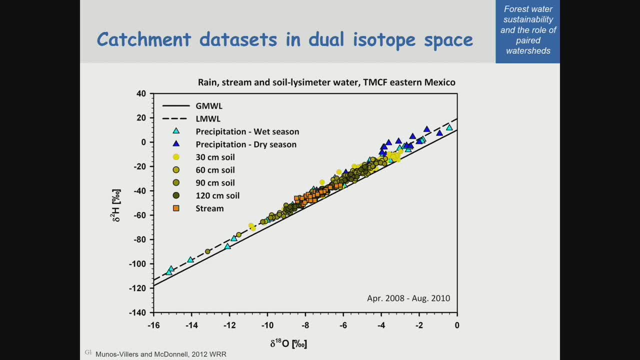 So just bear with me for a moment. I'm showing you basically the same thing now, but with the two isotopes plotted together. They behave very similarly, So they plot along this line. this so-called meteoric water line- The blue here- is spanning a wide swath of that line. 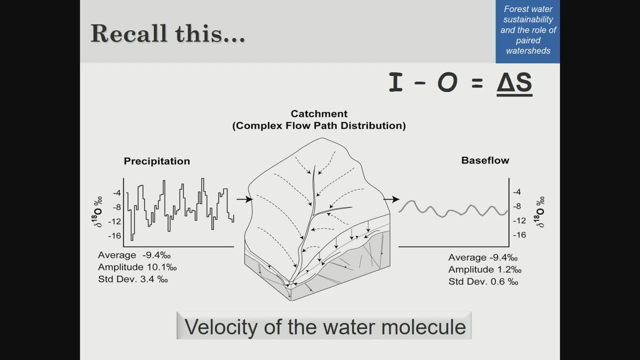 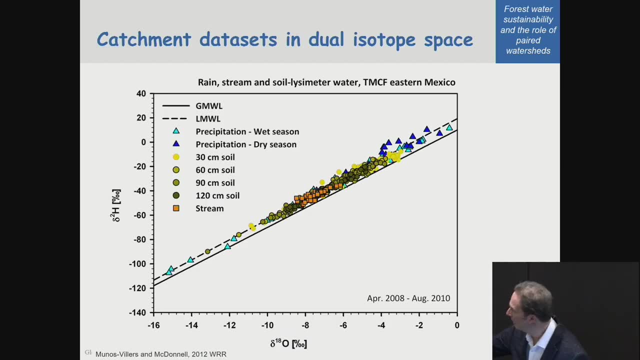 Just like in the previous slide. if you can see this part on the left, The rain is oscillating widely across that range. Well, that's what we're having here Now. you see O18 on the x-axis, deuterium on the y-axis, and the blue line is the rain. 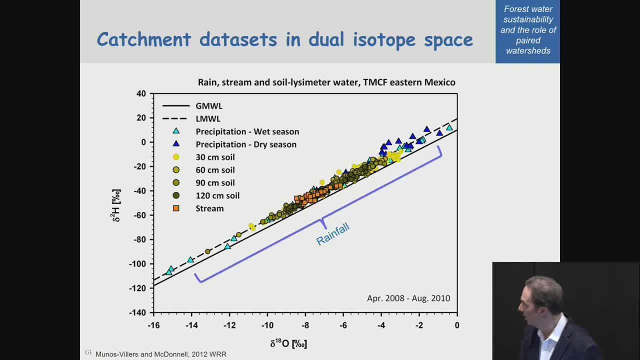 It's oscillating along that range And if we look at so, that's the rainfall. If we look at the soil, water or the streamflow, it's getting progressively lagged and damped, meaning it's compressed along that line. The point I want to make is that up until maybe 10 years from now, it's going to be. 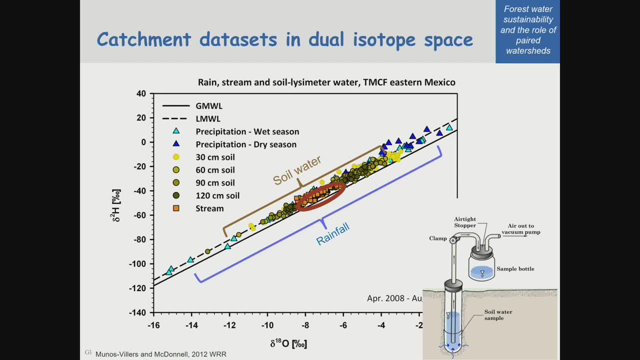 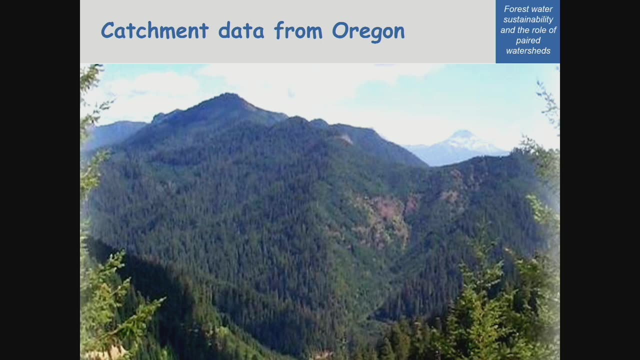 10 years ago, Every catchment I'd looked at in terms of isotope composition, the water had fallen on that meteoric water line. Sites in Asia, North America, Europe- all had had similar behavior, Until I started working with a forest ecologist in Oregon. 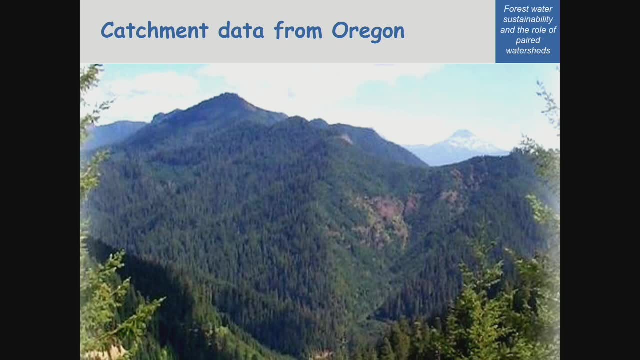 And this was a site, a paired watershed site. That's a 10-hectare catchment, And we were having coffee one day talking about the data that I'd collected- just like that site- I didn't mention it's from Mexico, but just like one of our field sites, all of the water. 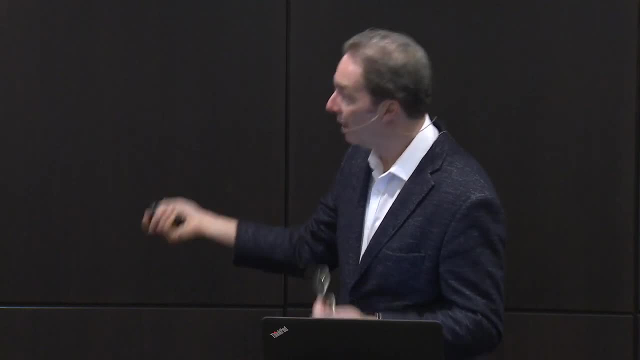 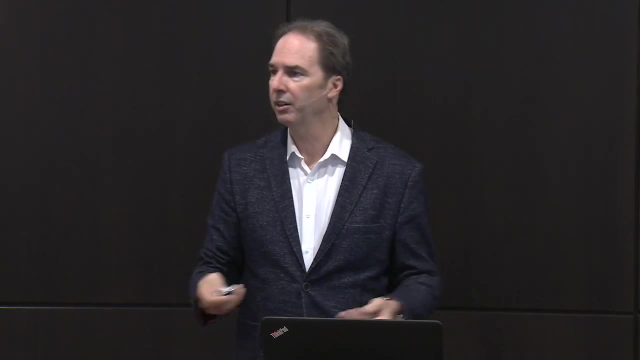 I'd ever looked at, had plotted on that meteoric water line, And my colleague Renee Brooks, who was sampling tree water- the xylem water in these Douglas fir stands- brought her data- isotope data- to coffee one day. 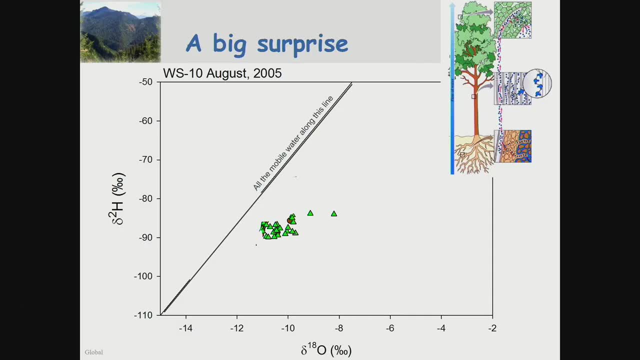 And this is where her data plotted. So this is that same meteoric water line plot with the two isotopes. That solid line is where all my data for years and years before that had plotted at this catchment as well And brings to coffee her data, which all plot over here on the right-hand side. 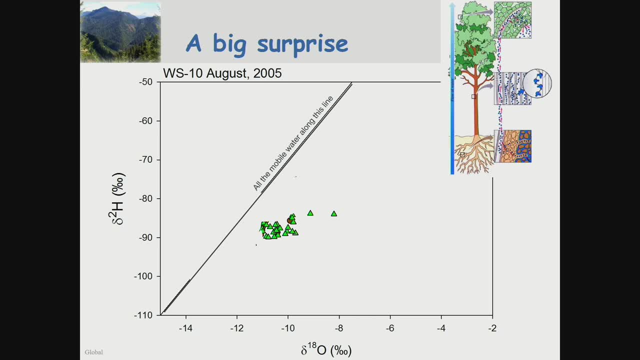 And anything that plots below the line is a tell-tale sign of some kind of evaporative fractionation. So the question was: where the heck are these trees getting their water? Because the water that I'd sampled with a suction lysimeter fell on that meteoric water. 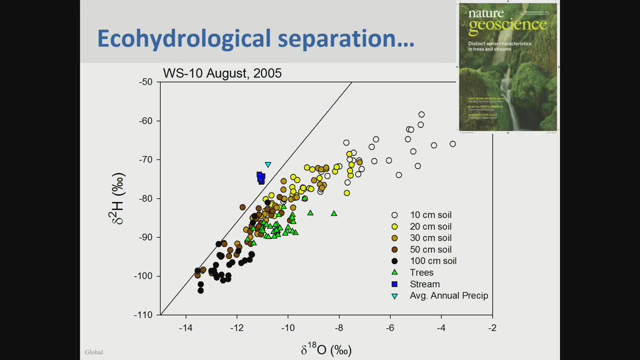 line. That's what prompted us to go into the field with a PhD student, Holly Barnard, who's now an assistant professor at University of Colorado. She's a professor at the University of Colorado. She's a professor at the University of Colorado. 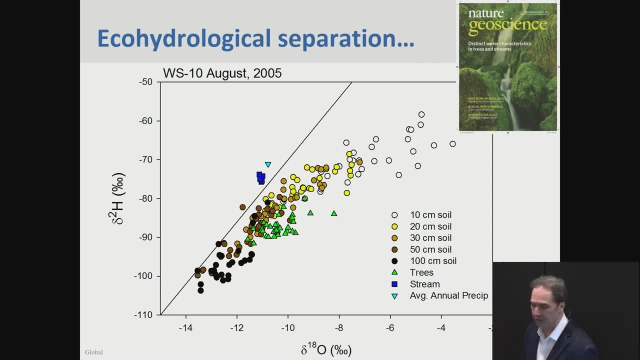 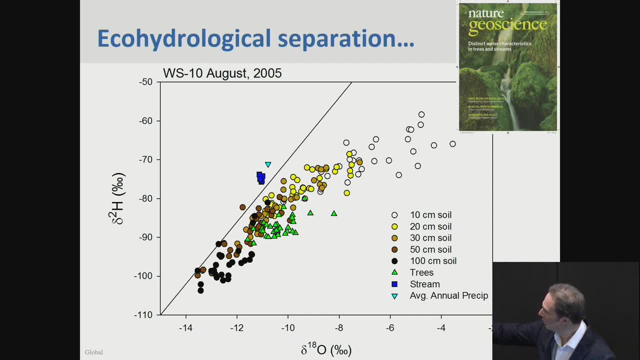 And as we move down that kind of slope back to that meteoric water line, we're getting deeper and deeper into the soil profile. So, not surprisingly, the trees are using soil water, but it's a certain type of soil water. These are soil waters that we brought back to the lab and we did an extraction to get. 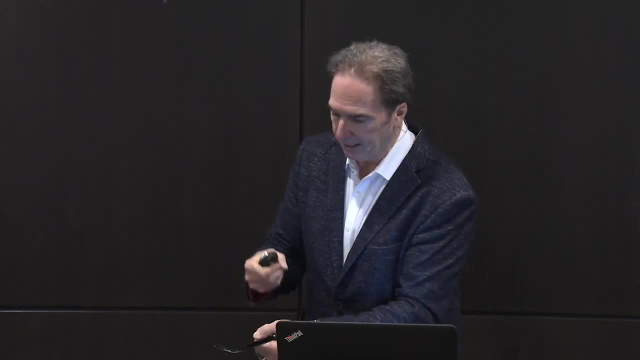 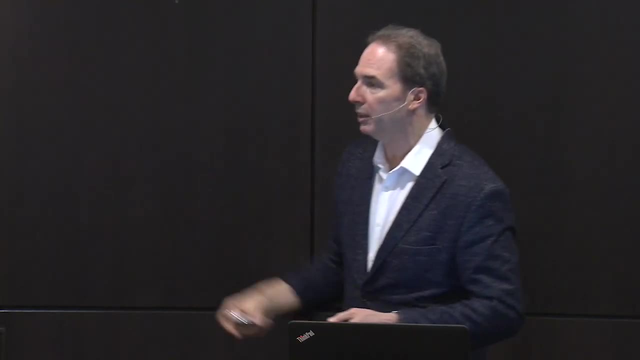 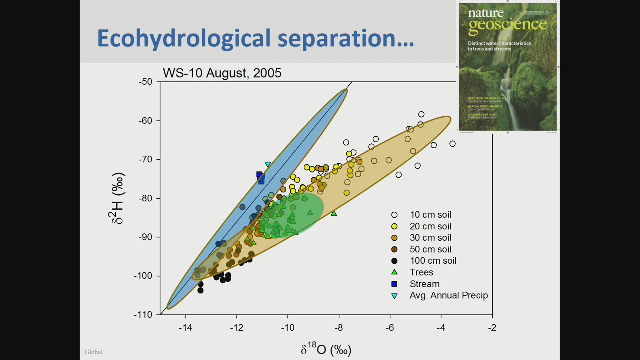 all the water out of the soil, Much more water than I could get out with a suction lysimeter- And what it suggested was that there was a mobile water world in the blue kind of hugging, that meteoric water line- and a lower mobility world, the more bound soil water, if you like. 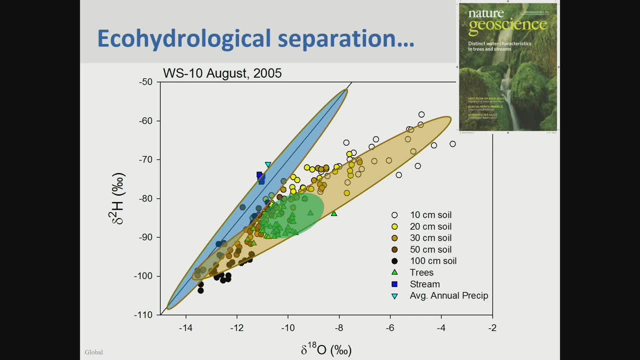 that the trees were tuned into, And the surprise of this is that it's a temperate rainforest. This is a picture of our site here. It's a mossy, wet place. It's seasonally dry in the summer, It's summertime, but it's a wet, wet environment. 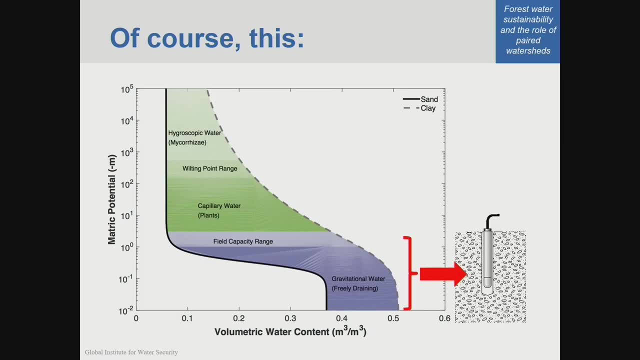 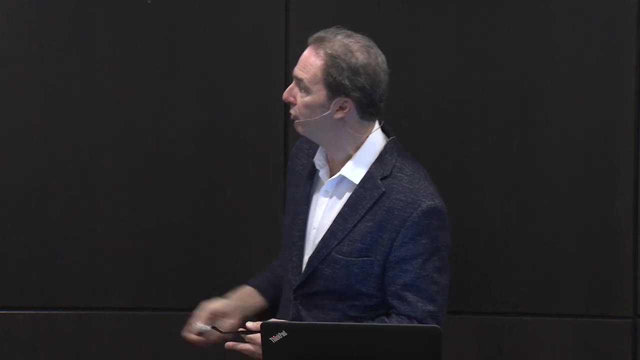 This isn't a semi-arid watershed by any means. So, of course, if some of you are in the Geography 420 class, you've looked at the moisture release curve as a basic descriptor of soil water movement and behavior. metric potential on the y-axis versus volumetric water content. 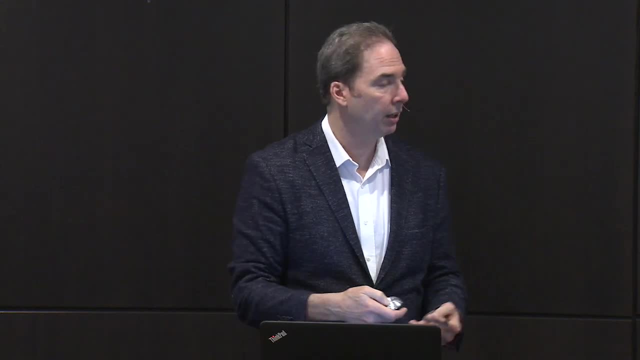 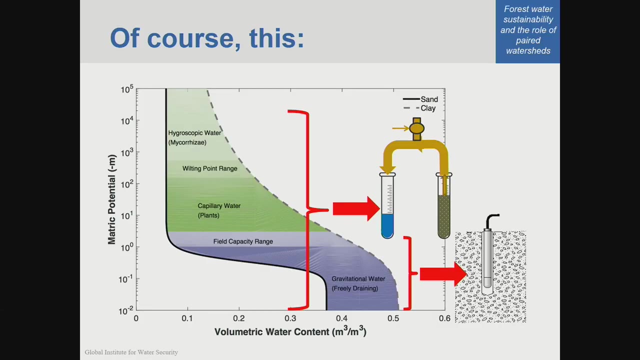 This soil. this suction lysimeter that we used to sample soil was really just getting this easy-to-get water, the so-called gravitational water, Whereas the tougher-to-get water that this extraction technique gets out really gets all the water, even the much more tightly bound water. 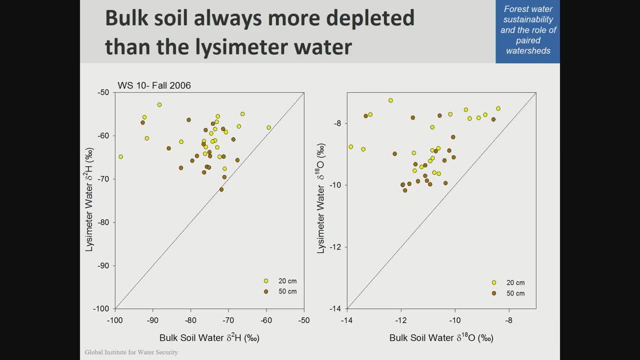 The point, though, is that when you compare these two waters, they're not mixing. So here's one plotted against the other. It's the lysimeter water on the y-axis versus this extracted bulk- so-called bulk water, And in each case, these pools aren't mixing. 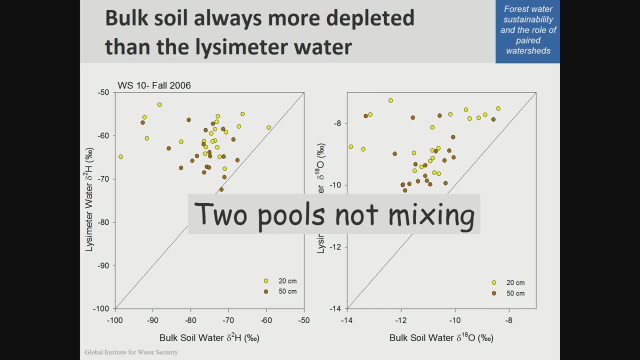 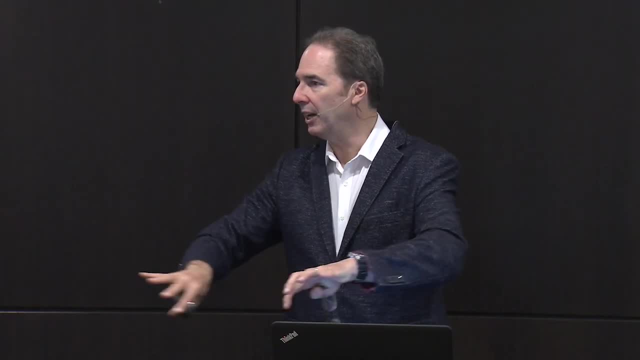 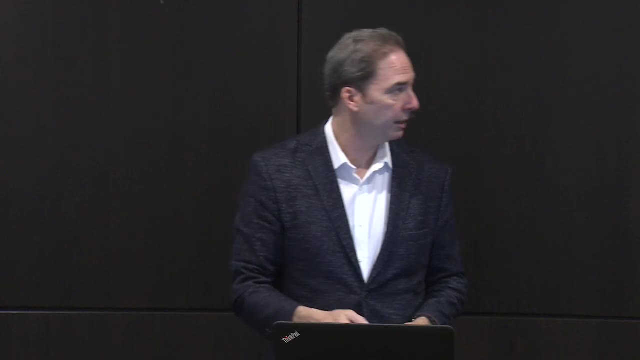 This was very surprising for us. We thought It would be one big, well-mixed pool. the trees would draw from it. what was left would go to groundwater recharge, and what this is saying is that these cycles are somewhat separate, And this is a cartoon of the separateness, if you like. 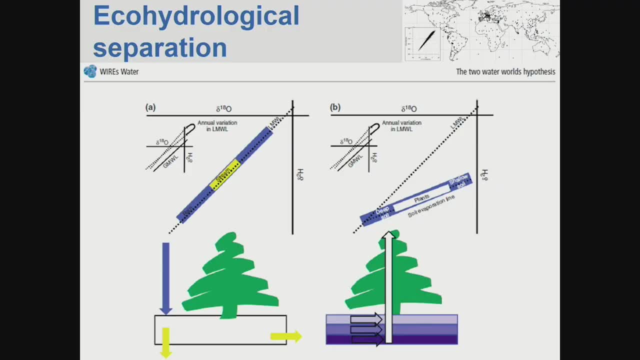 You've seen the one on the left a lot now. This is really the mobile part of the system. The rain is spanning a wide range of that meteoric water line. The stream is a lagged and damp version of that rain And on the right side, 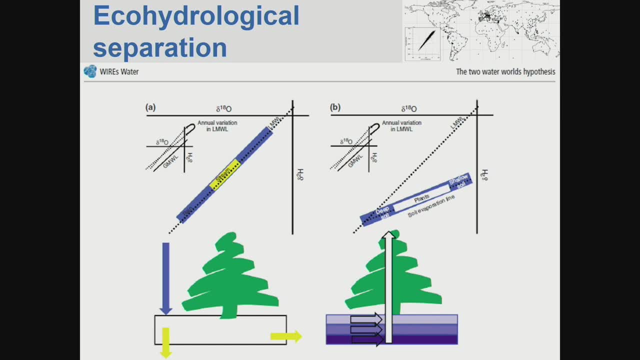 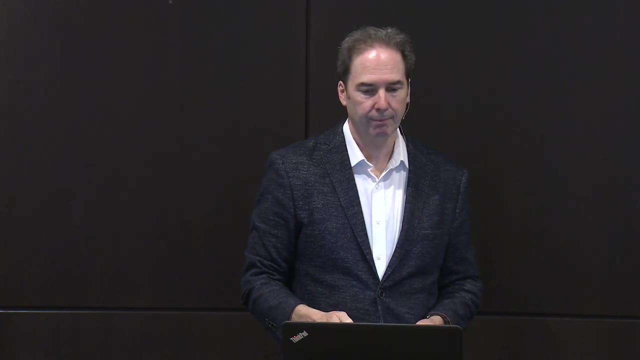 This is more what seems to be happening with the vegetation. It's keyed into the soil water evaporation line. It's a lagged and damp version of that soil water And these two lines, these two pools of water don't seem to be mixing or interacting. 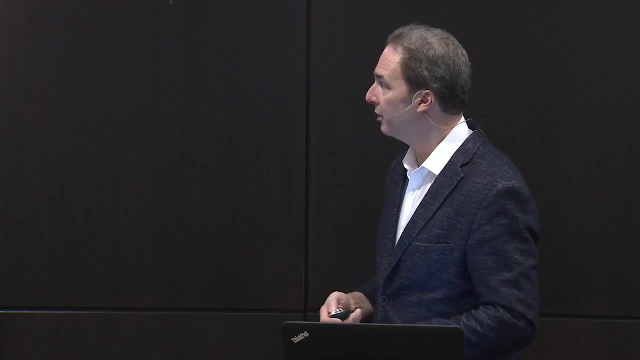 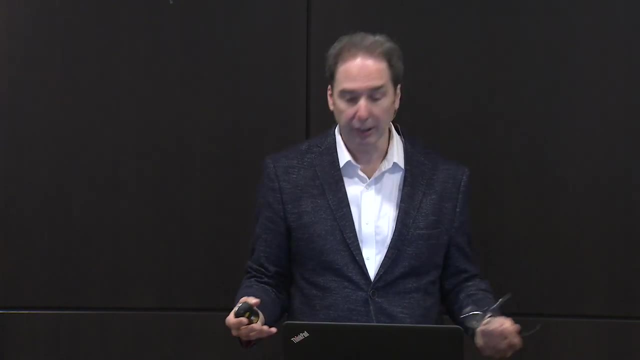 We thought this might just be an anomaly at this particular site. Habame's first task for his PhD was to see whether or not there was widespread evidence of this. It's in the literature. He did a meta-analysis of about 50 sites. 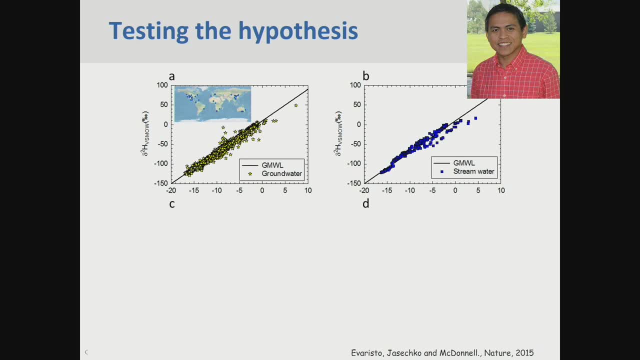 You see a map of them in the upper left And basically the two plots up top are this global dataset, if you can call it, that of stream water and groundwater, all hugging that meteoric water line, as we might expect. But then the plant water and the soil water that went with these datasets is all drifting. 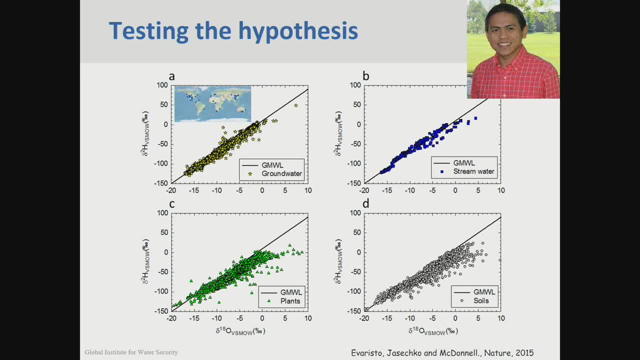 off on that shallower evaporation slope. So this was kind of some evidence that this is in keeping with the literature and this is covering many different biomes. I think we had seven different biomes that are being represented by these data. 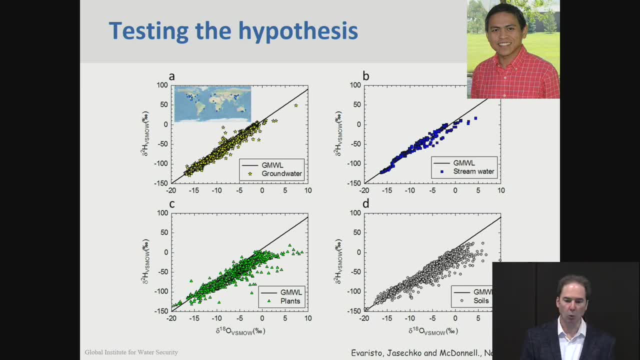 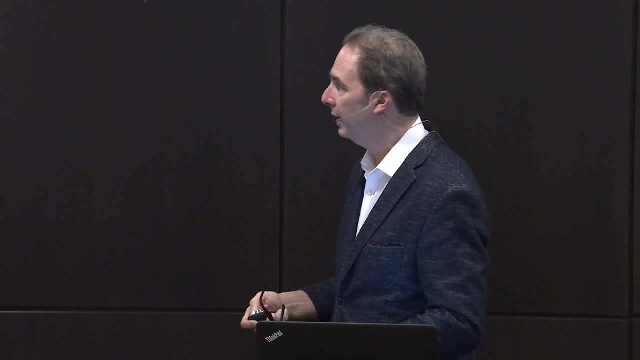 So this is an issue with para-watershed studies: One that the trees may be using water that's not well-connected to the streamflow response. The other thing is that trees can also use groundwater. This is another meta-analysis Habameh recently completed. 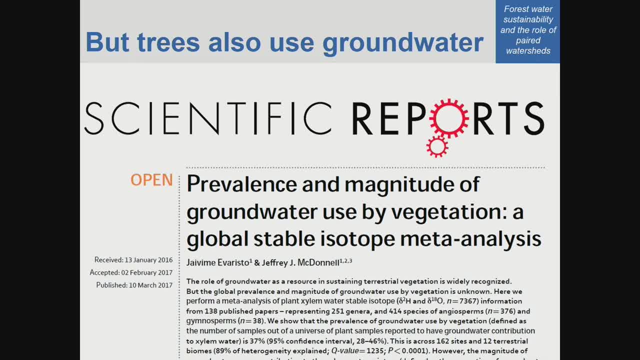 showing that groundwater use by vegetation is fairly prevalent. from an analysis of over 100 papers- There were 138 papers we were able to find in this study. The prevalence of groundwater use by vegetation was high, about 35% or 37%, but the magnitude of groundwater use 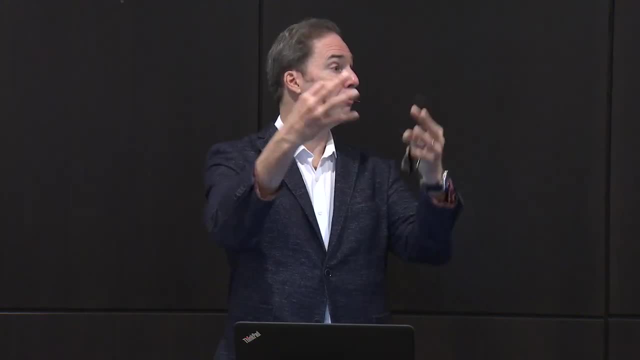 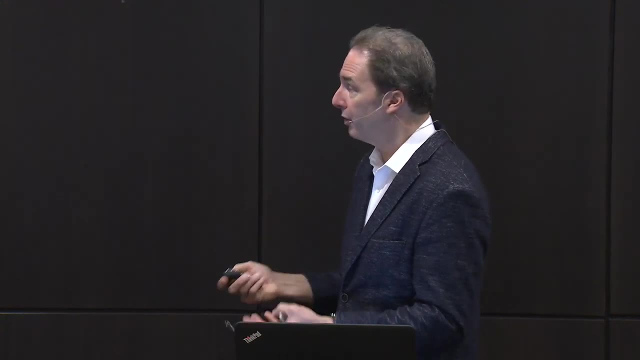 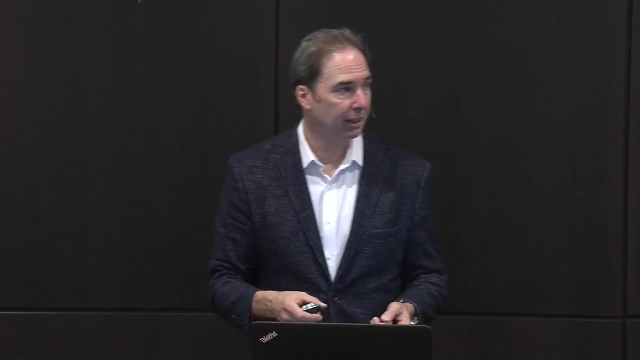 meaning how much groundwater was represented in that xylem transport was closer to 20%. But trees also use groundwater and that's another factor that we need to think about in this kind of paired watershed approach. And the last example I'll give: 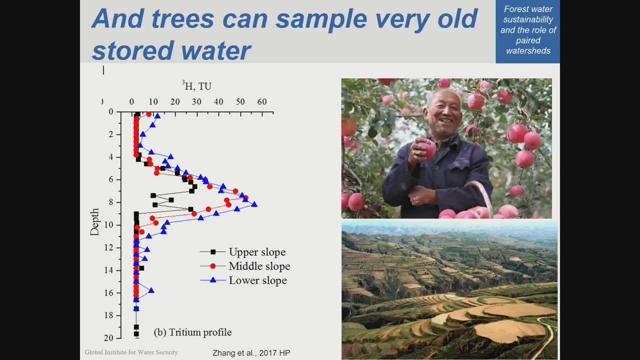 sometimes this water can be really old. Now we're in China, we're on the Luz Plateau and we're looking at trees. Here the big afforestation is with agricultural trees, apple trees. Just look at this plot on the left. 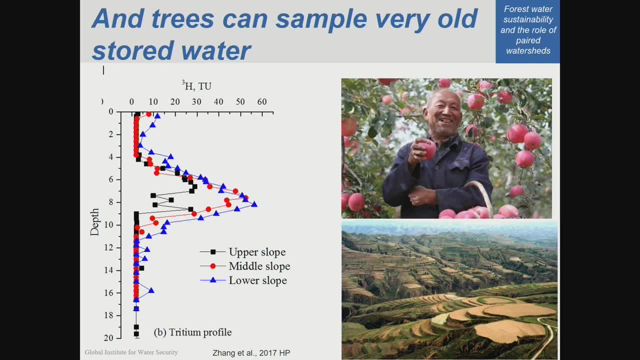 This is depth, from zero to about 20 meters, and now we're looking at a different isotope. This is tritium and this is bomb tritium. So remember, back in post-Second World War, there was thermonuclear testing. 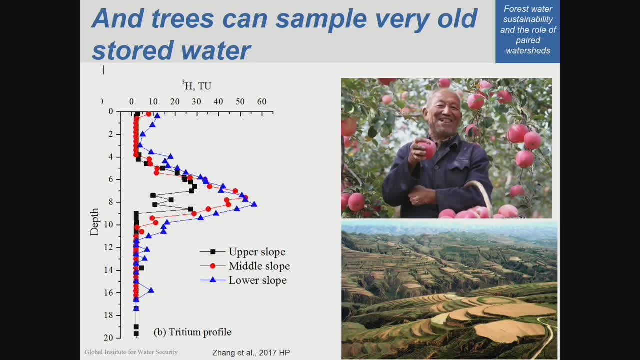 We had a test-bound treaty that came out in 1963, and the tritium composition in the atmosphere peaked then and it's been on the decline ever since. It's largely washed out of the atmosphere in the southern hemisphere. We still see remnants of it in the circulating north. 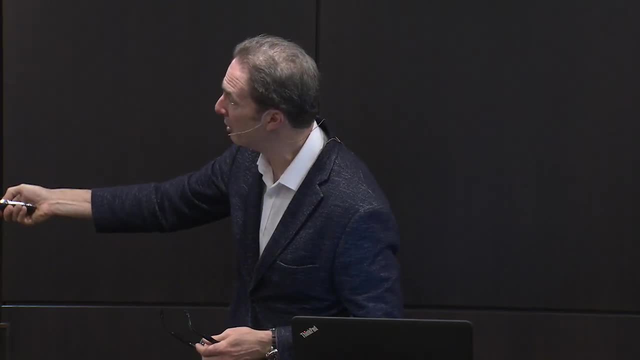 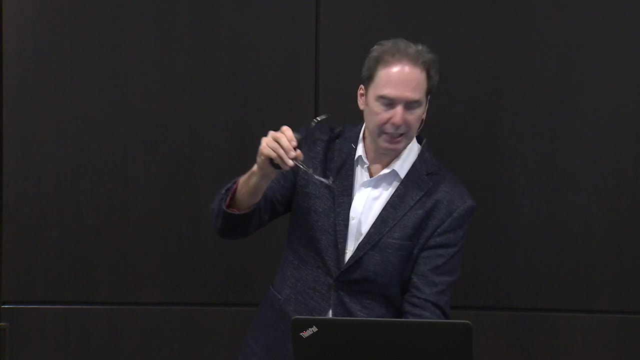 southern hemisphere. Well, here's a beautiful preservation of that in soil: water from zero to 20 meters on this Luz Plateau. The Luz Plateau- very deep soils- We're talking over 100 meters of silty, wind-blown soil. 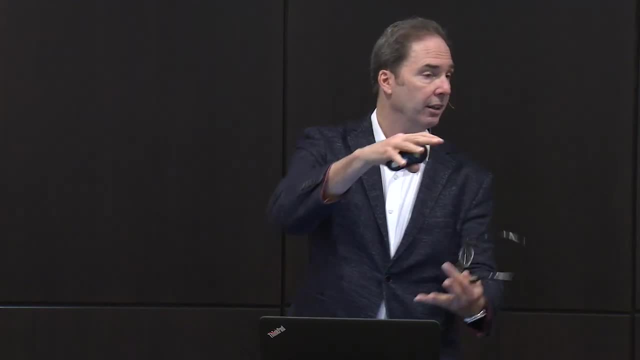 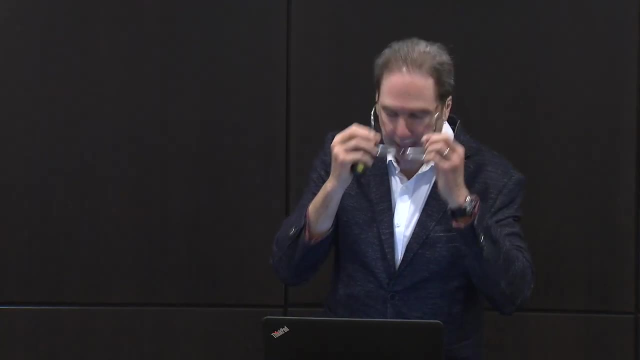 The water table is 50 meters down. So this is in the unsaturated zone, the Vedos zone, And what you see is that 1963 peak is sitting there at about 8 meters or so. That's kind of the slow movement of that tritium. 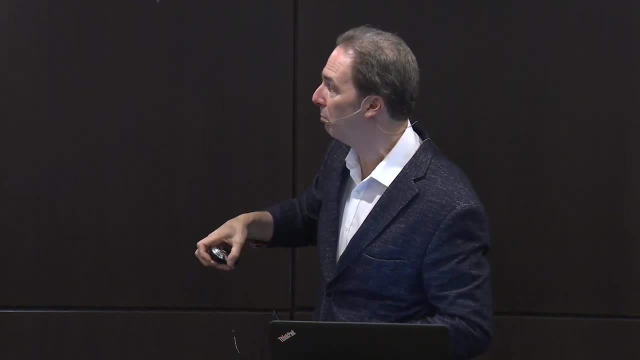 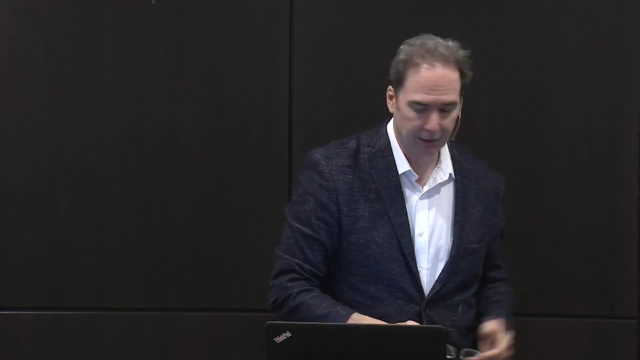 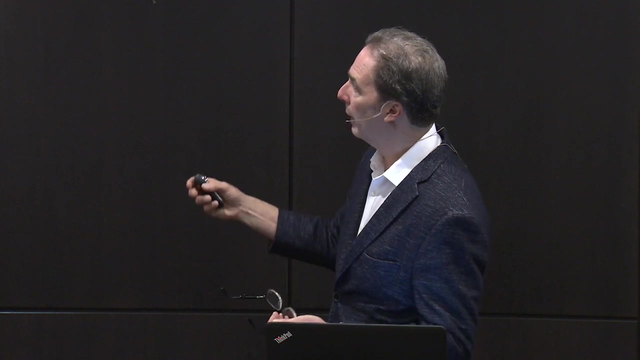 it's taken since 1963 to get to that plot. The trees are rooting through that depth. This is the fascinating opportunity here, with a graduate student from Northwest Ag and Forestry University named Zhang who's working with Bing Si, where we were able to do a mixing analysis. 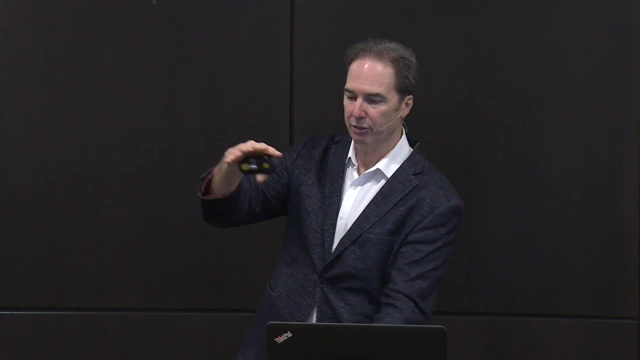 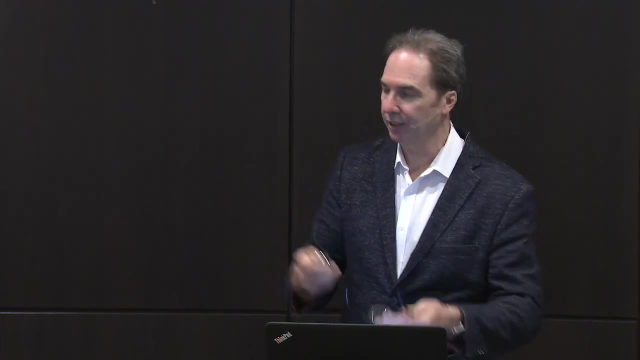 to ask the question: well, if we have a beautiful preservation of age, how old is the water in these apples? Because, again, most of our thinking is that this is this season's water And what we found was the water in these apples. 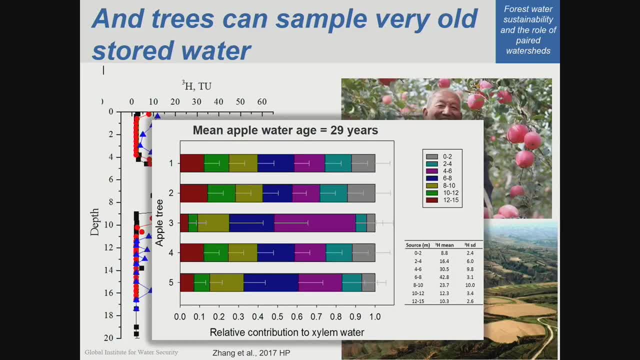 was, on average, 29 years old And we were able to age date that with the tritium and showed that in fact, this is now looking at five of the apple trees and these colors represent the depth distribution of water uptake And you can see that water uptake was fairly distributed. 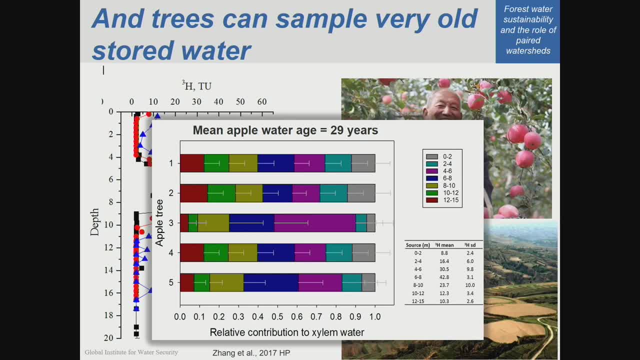 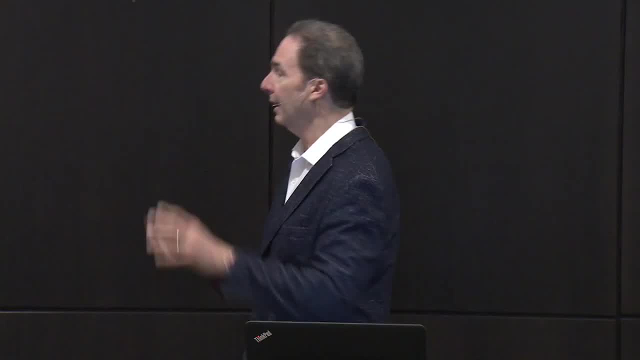 in terms of the relative contribution on the x-axis here throughout that profile. So it was kind of the perfect experiment. So it was kind of the perfect experiment to try to quantify this age. I'm not saying that the, you know, the jack pine at the berm site north of Saskatoon. 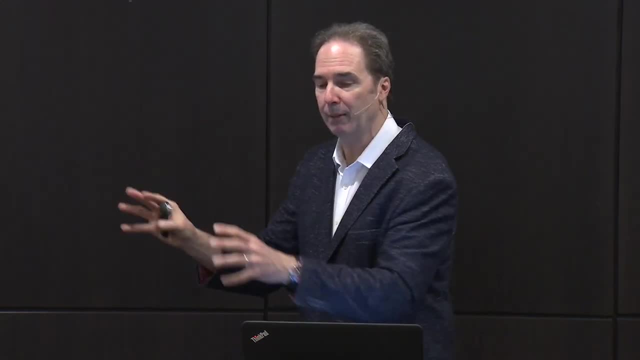 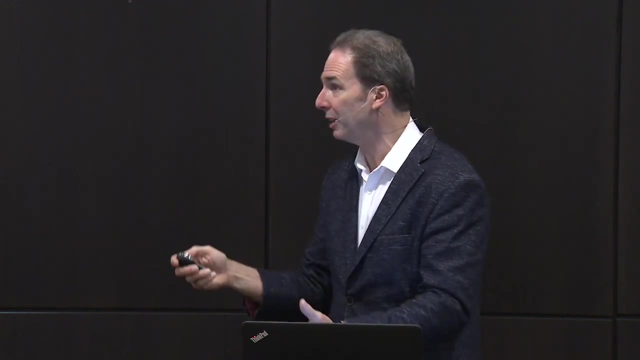 are using 29-year-old water. This is an anomalous site, but it kind of gets the point across that if we're doing paired watershed studies and we're not thinking about the subsurface, which we've not really thought about in these compilations or individual studies, 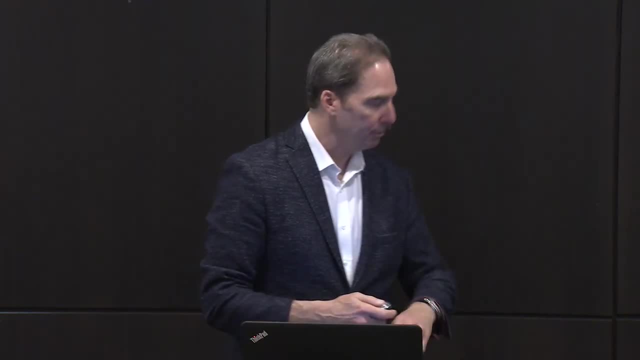 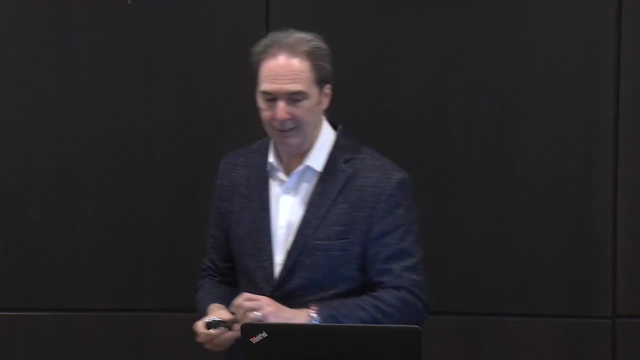 we could really be missing the boat. So let me try and wrap up with a few comments about what all this means, maybe for sustainability. And let's go back to this odds ratio meta-analysis. Basically, these red lines are showing that there's a lot of variability. 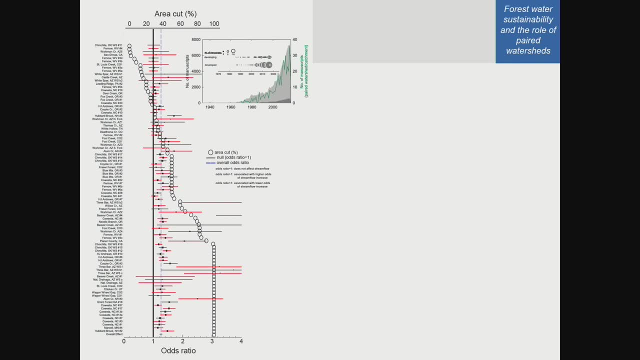 And, as we saw before, you could have a little area cut with a big response, a lot of area cut with a little response and everything in between. And I guess the hypothesis I'm throwing out there is that storage and how kind of storage selection. 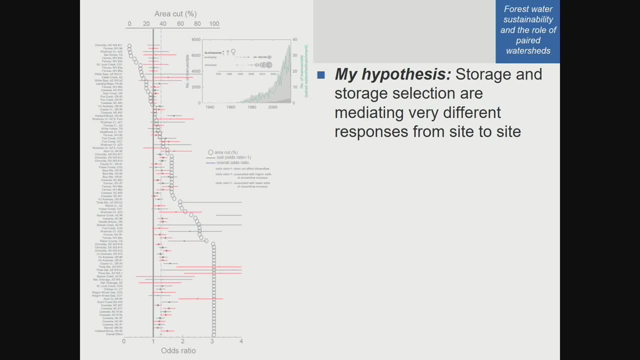 for want of a better word, I think could be mediating these very different responses from site to site, And this is something we've not looked at. And maybe this new question for sustainability is to get at the inventory in the system, in the water balance, if you like. 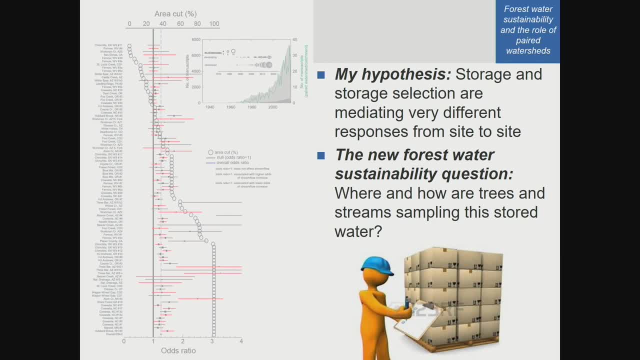 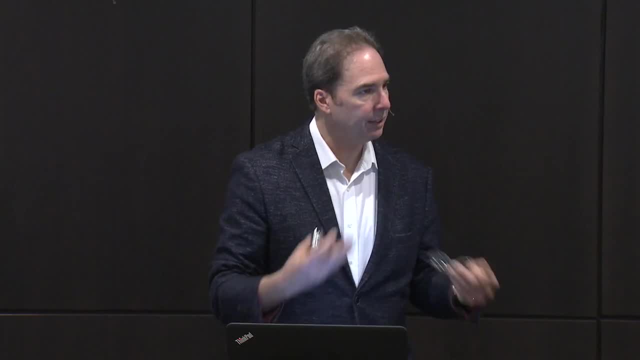 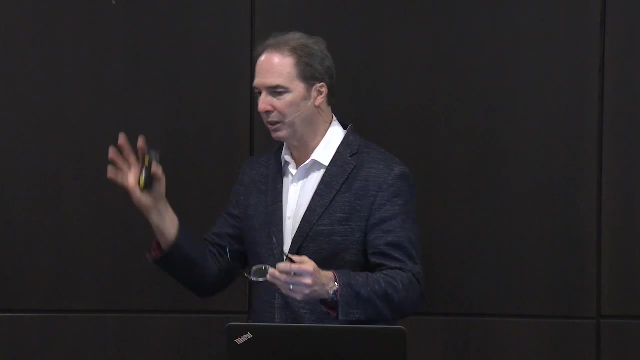 and ask the question: where are the trees and streams sampling the stored water? And that is a question that we can go after and maybe begin to shed new light on sustainability, Because just think, I mean, would your sustainability framework if you were doing a consulting job? 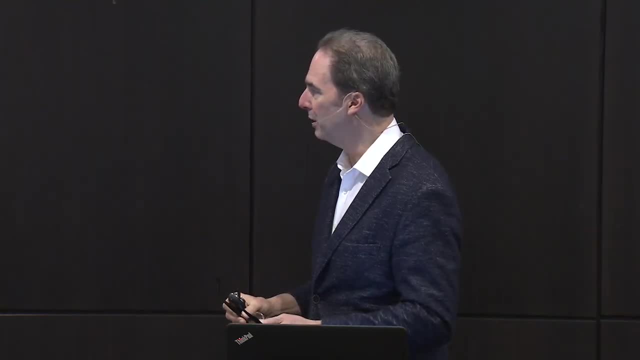 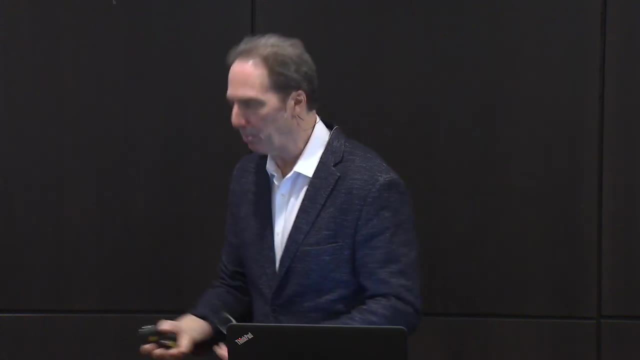 for the World Bank be changed. if you knew the trees were using day month-old water versus 30-year-old water. It's kind of like the sustainability of pumping an aquifer: Are you pumping a fossil groundwater that's not going to be recharged on a human lifespan? 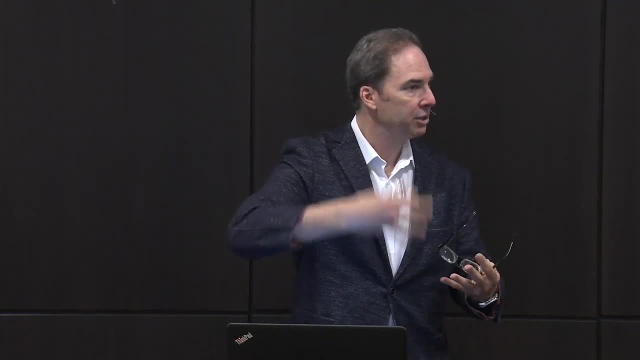 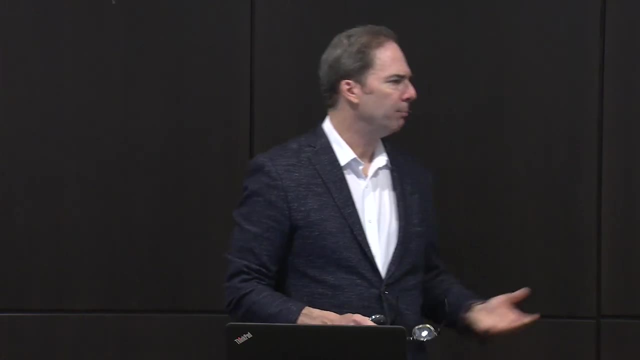 Or are you pumping a very young water that you know is being recharged actively each year, And I think this is going to require kind of rethinking paired water, And I think we're going to need to really understand how we're going to be. 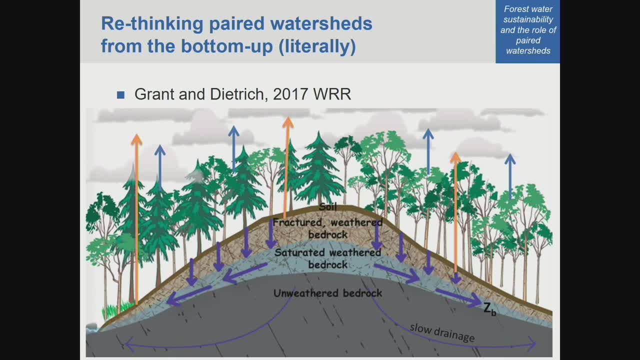 able to get these water sheds from the bottom up. pardon the pun. literally meaning we really need to understand what is the storage, the dynamic storage, the passive storage. We had Bill Dietrich here in our first lecture. This is a paper that Gordon Grant and Bill 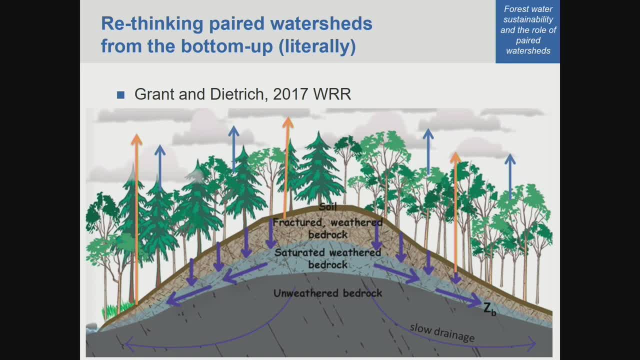 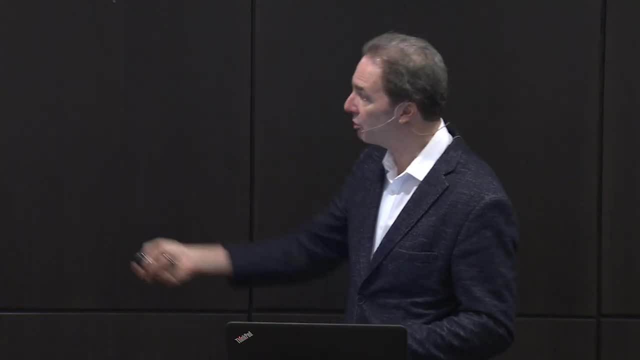 published a couple of months ago just talking about this critical zone and how streams and trees are sampling from these storages. I think is really the key question And I think it's important to think about how these storages can be highly variable. 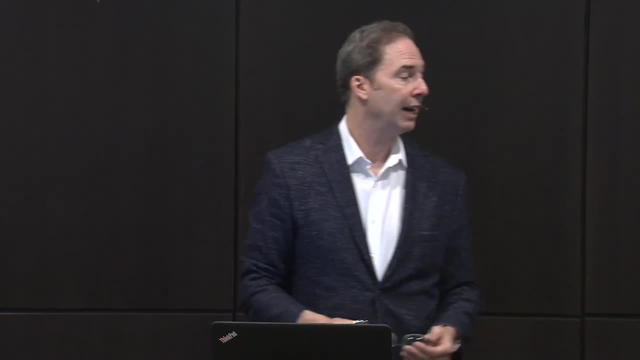 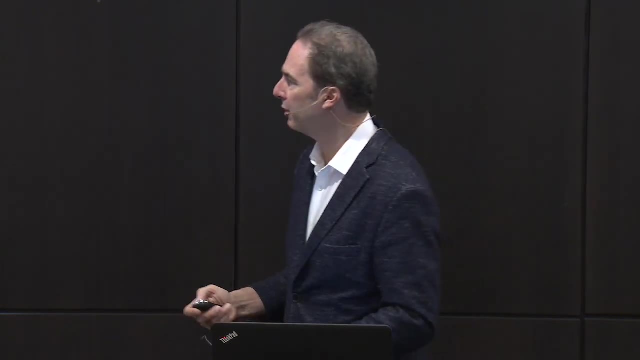 and can be quite large. Some watersheds where I've worked, it might be 50 millimeters, Some could be over 1,000 millimeters of storage, So the storage could be greater than the annual rainfall. This is, I think, a big factor. 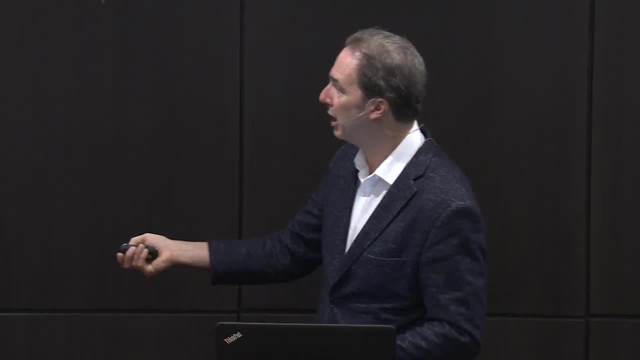 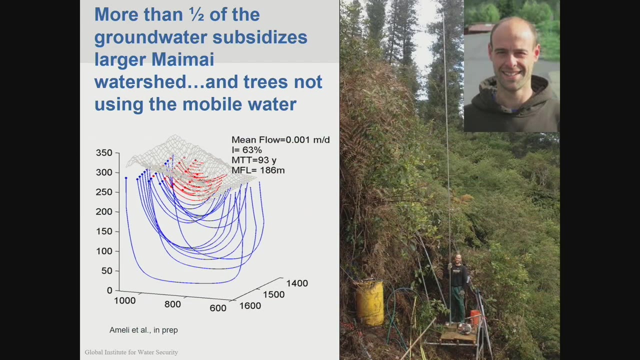 in the paired watershed approach. And the last example maybe, and coming back to the scene of the crime, at least for me, this is the Maimai watershed in New Zealand, where we've continued to work. This is Chris Gabrielli, who's just finished his PhD. 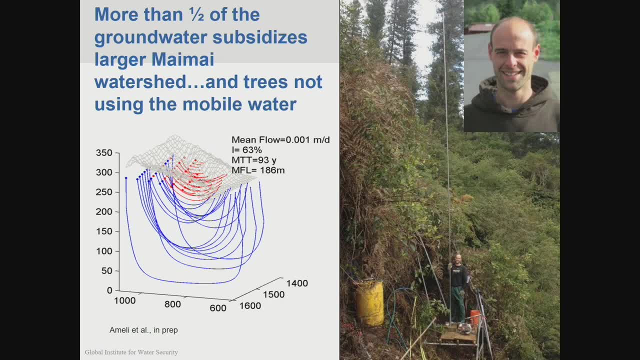 we've been drilling into this bedrock. So here's Chris on a drill string. He's going down about 10 meters into the bedrock below the soil in this forested catchment And, working with Ali Ameli, we've been using these data. 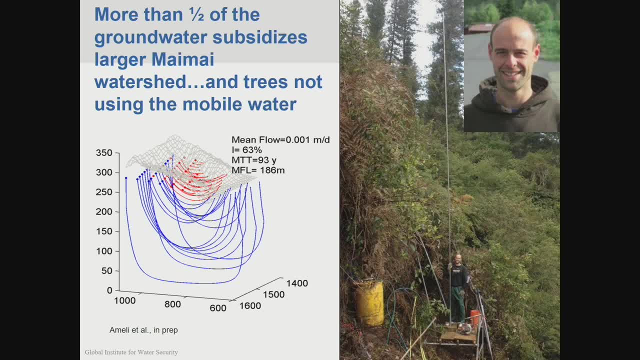 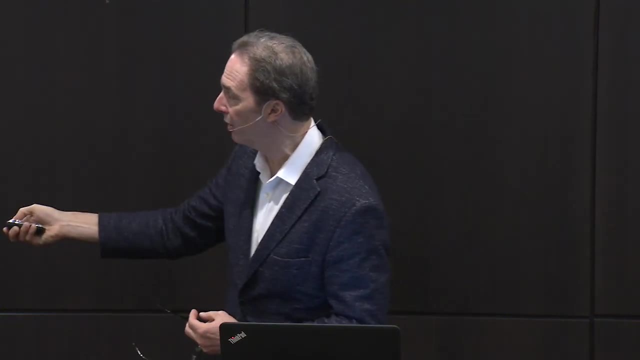 where we age date the groundwater with tritium. We understand the kind of the bedrock permeability architecture from the 40 or 50 wells Chris has drilled And we can use that to model where that water is going after it gets into the catchment and recharges. 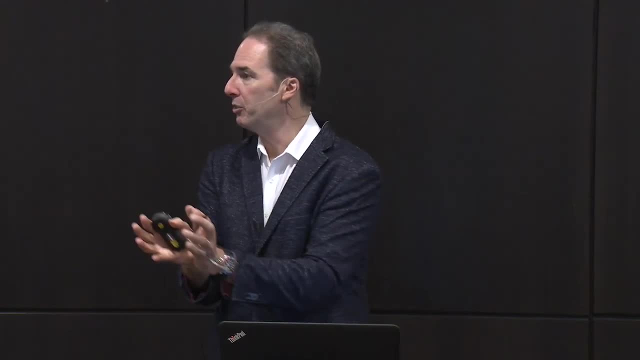 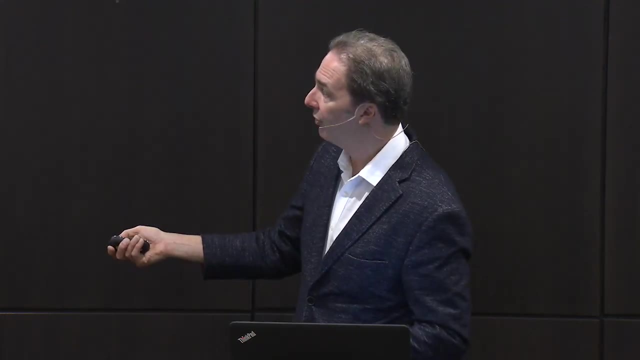 Previous thinking was that, like most of these forested catchments, they were tight and anything that fell, if it didn't transpire, it would make its way out as streamflow, And what we're finding is that about half of the water. 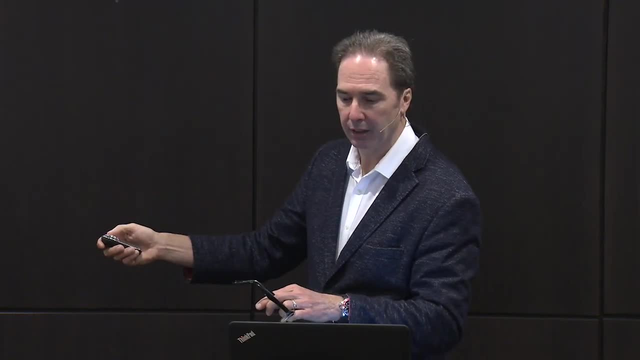 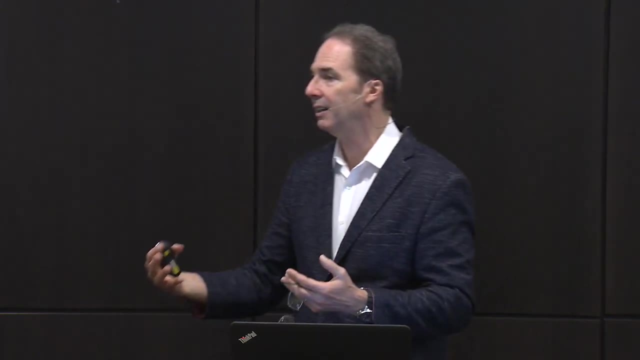 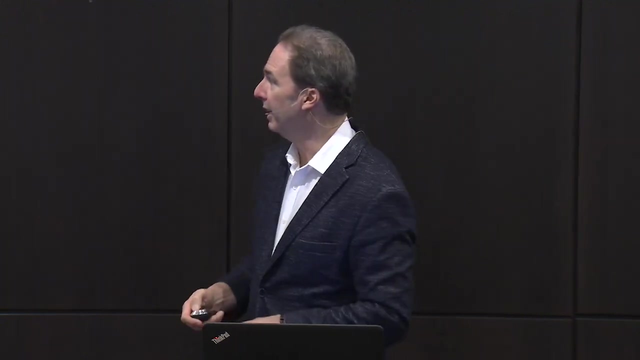 that's recharging groundwater in these headwater catchments is not coming out in the headwater catchment, It's subsidizing larger watersheds down valley, which is really an issue for these headwater paired catchment studies. Okay, so I'll try and wrap up. 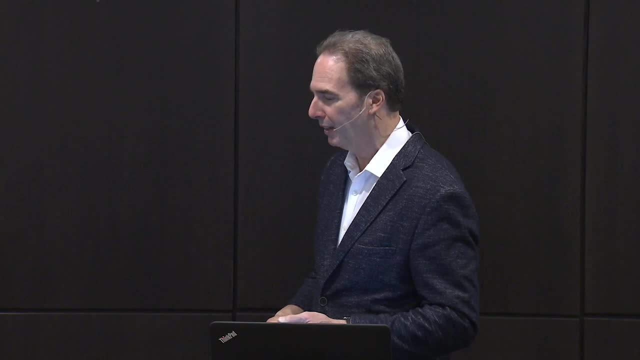 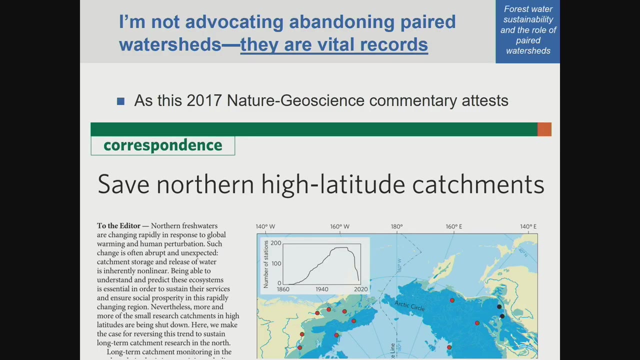 I guess the first thing I want to say- and this was really a concern of one of my co-authors- we need to make the point that we're not advocating, you know, throwing the baby out with the bathwater. We don't want to get rid of paired watersheds. 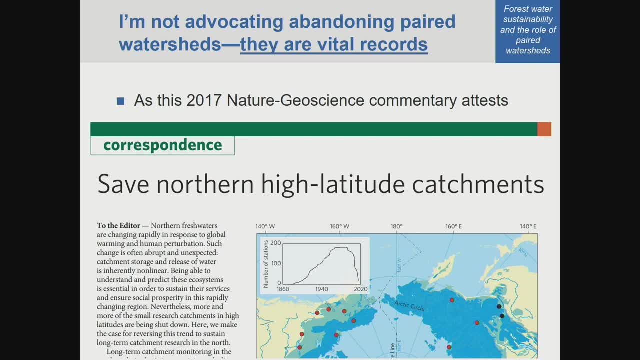 No, they're critical. Any watershed, long-term watershed study is critical, because they're going the way of the dodo. This is a commentary that came out a couple of months ago, led by Yalmar Laude. He's at the Swedish Agricultural University. 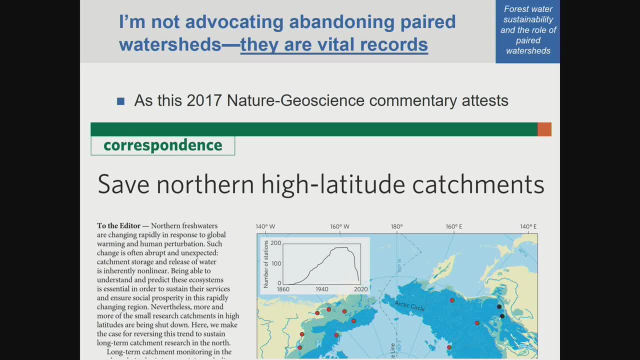 This plot for some of you who are in the Global Institute. this plot sits on a pegboard outside the restrooms on the first floor. if you've ever taken notice of that as you walked by, It's showing you the precipitous decline. 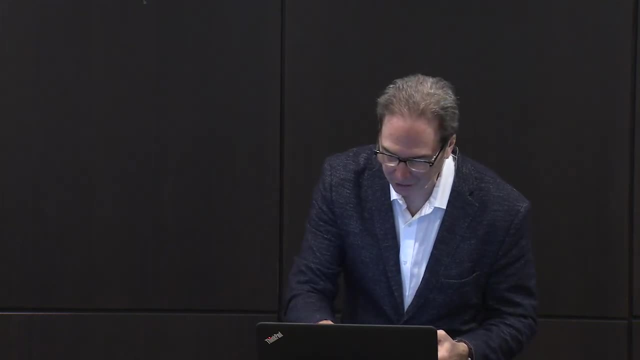 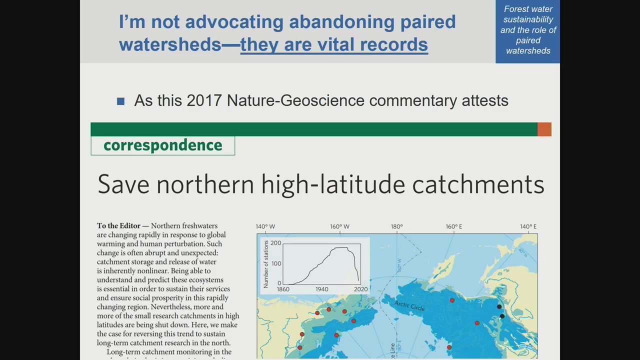 of stations in northern latitudes. So the x-axis is time from the late 1800s to now and the number of stations is shown on the y-axis, And I think this is true. It's true for paired watershed studies as much as it is for northern high-latitude catchments. 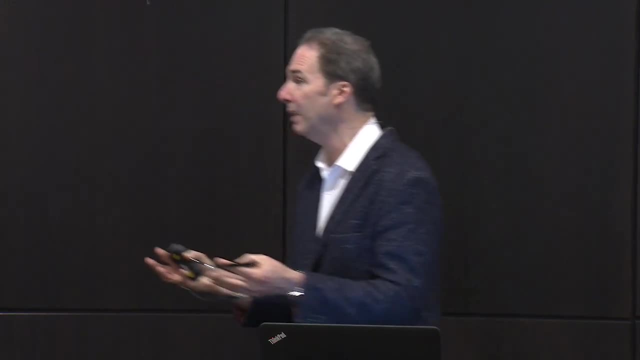 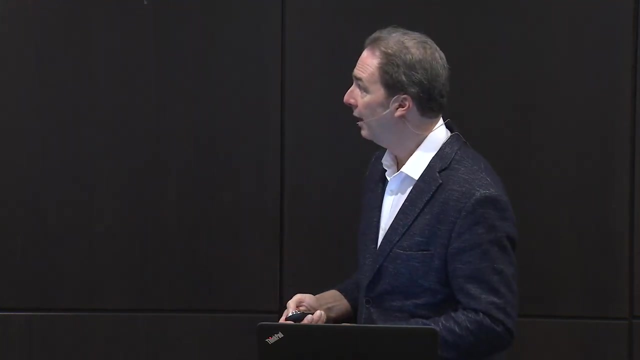 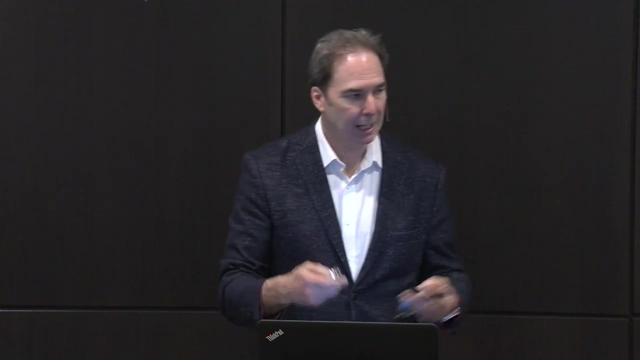 These are canaries and coal mines that we need to keep and to not lose sight of. What I'm advocating is augmenting the paired watershed approach by thinking about storage, by thinking about what's below ground, So thinking about how isotopes can be helpful. 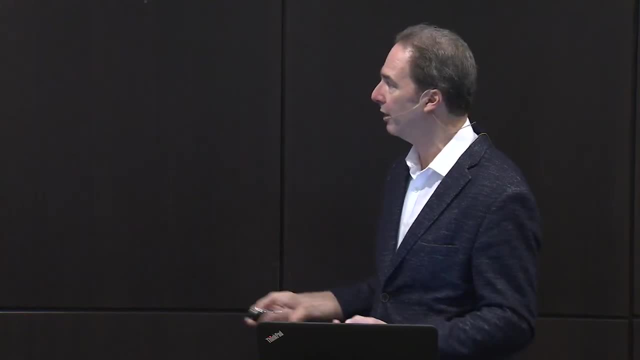 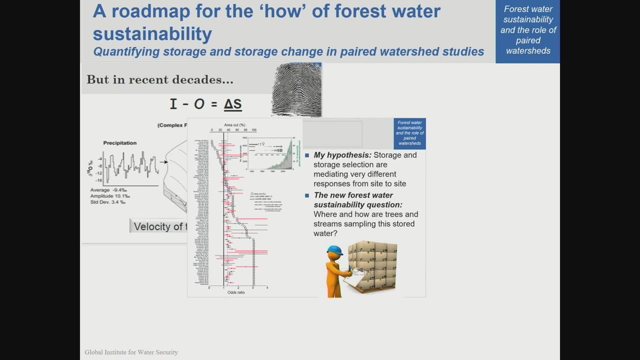 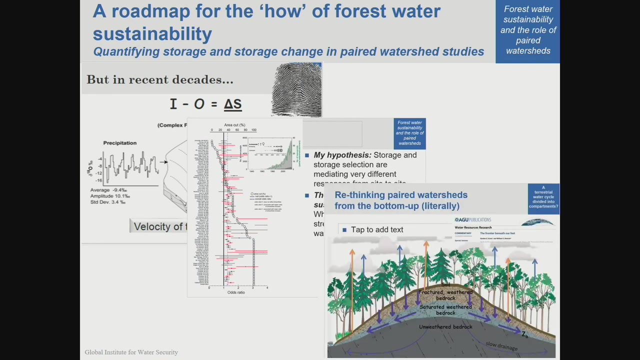 but not just isotopes, How this might help make sense of a lot of confusion. I think that exists because when you start to look across the many sites or many studies that have been done again, you get all manner of responses And I think these subsurface characteristics- 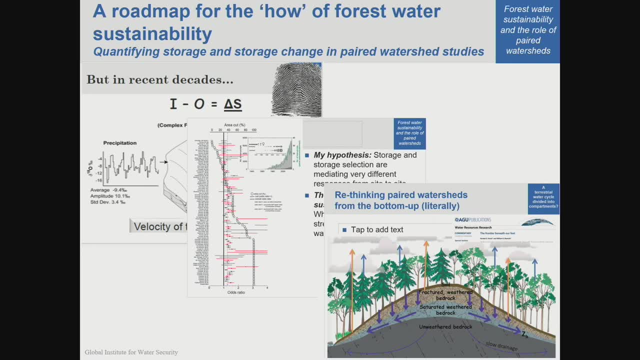 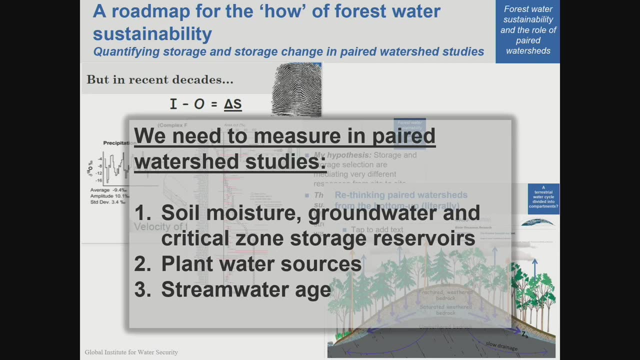 could be at work, And getting at this kind of critical zone is indeed critical, and it's measuring things like soil, moisture, groundwater. We don't have these measures across our paired watershed studies. It's simply a black box input-output kind of approach. 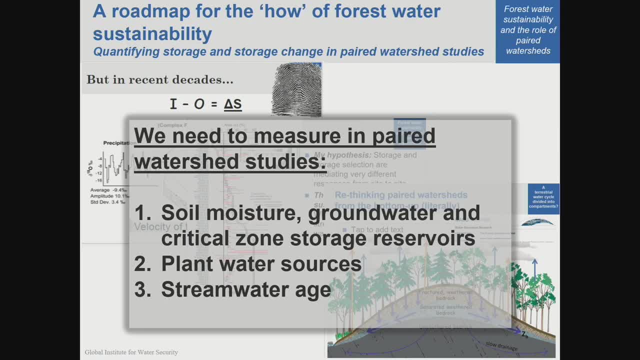 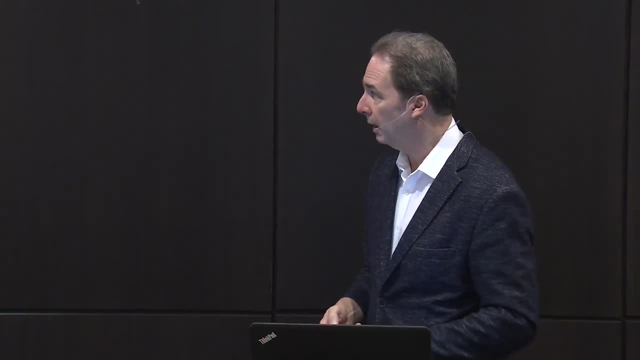 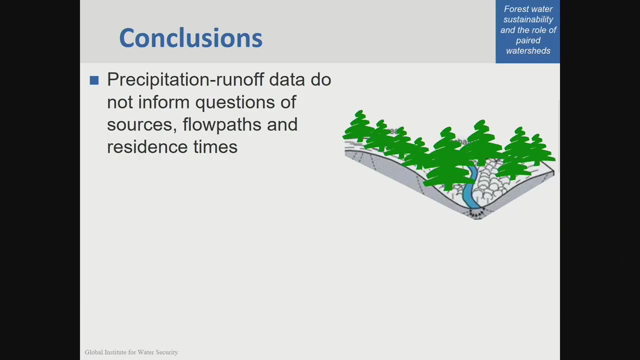 It's getting after plant water sources, It's getting after stream water age, because these are the things that can help illuminate the storage piece of the equation. So, if I try to conclude, I guess the main message is that precipitation runoff data really don't get at these questions of where water goes when it rains. 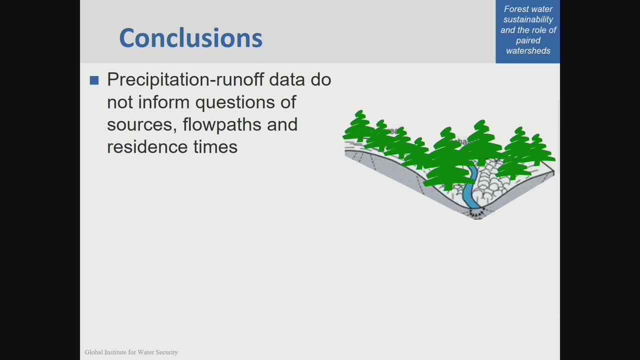 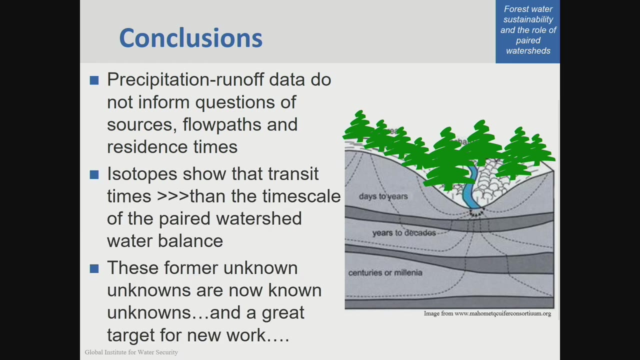 or flow path and residence time. And this kind of picture has to kind of change, If I can do the big reveal here showing this simple diagram to really think about how big the box is, how old that water is, Because this says something about the memory. 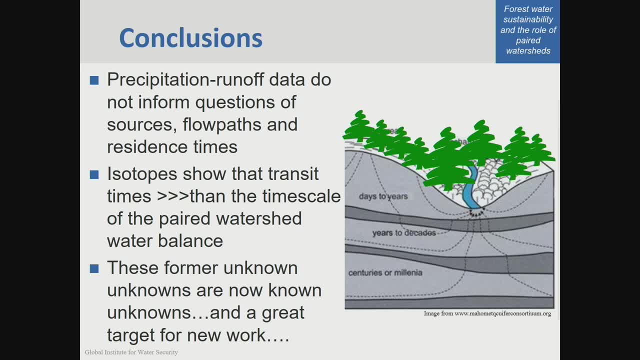 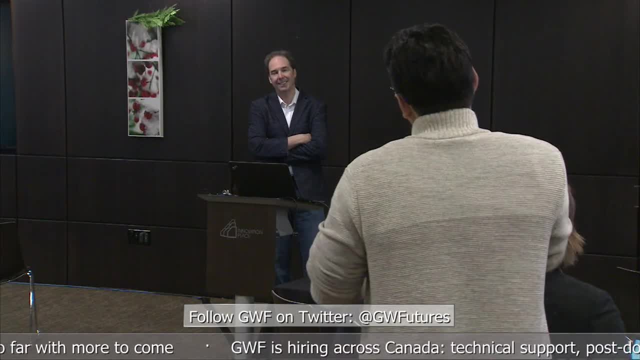 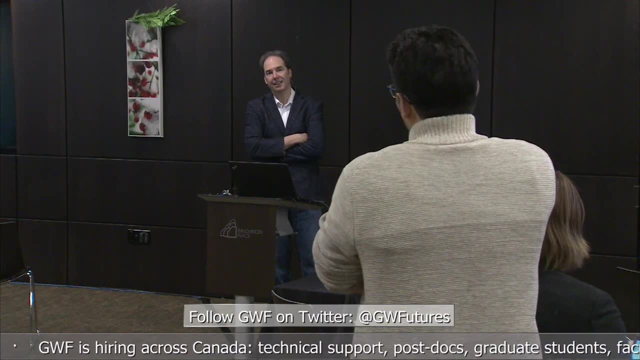 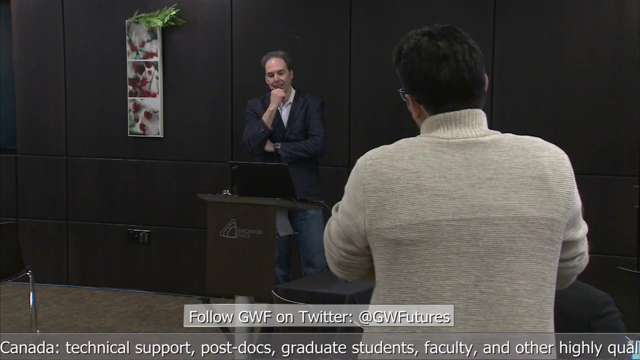 a can of worms for modelers, and you're questioning or challenging us about the quality or credibility of our predictions when we talk about the future to the end of the century. So I think fascinating stuff but very difficult for us. It is difficult. 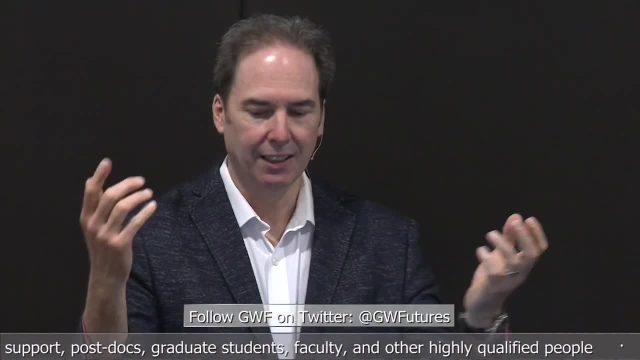 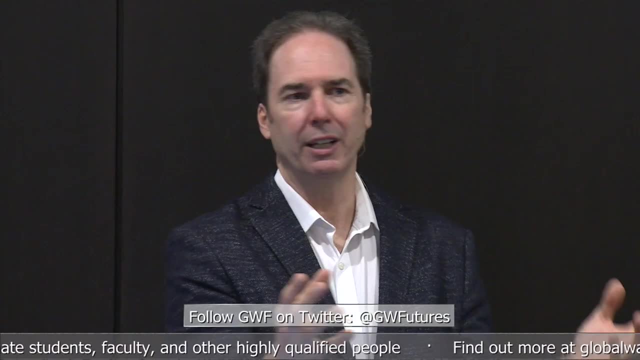 This came up in class today, Some of the students were asking: well, do you need all this detail? if you're really just trying to size a culvert and use a model, You don't really care if it's right for the right or wrong reasons. 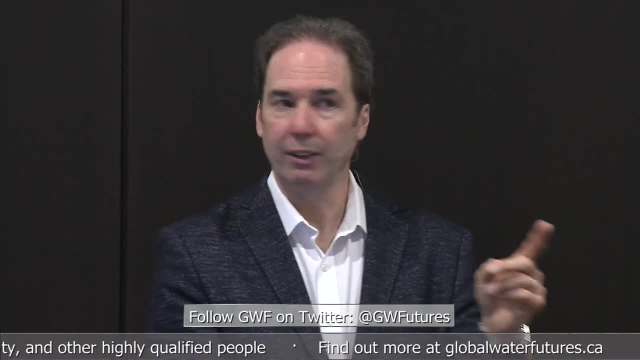 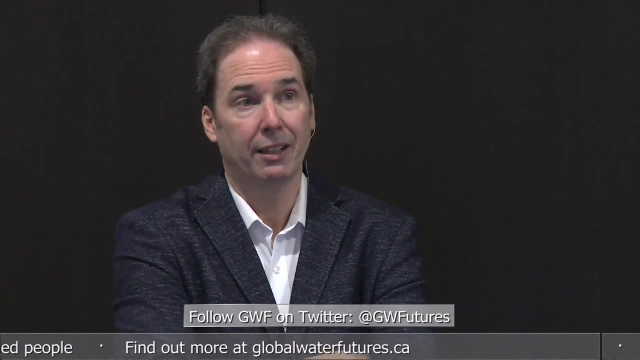 And I think that's a really good point and I agree, But right for questions of change in response to climate or land use change, where some of these timescales can be long, it can be a big issue. We work with simple catchment models. 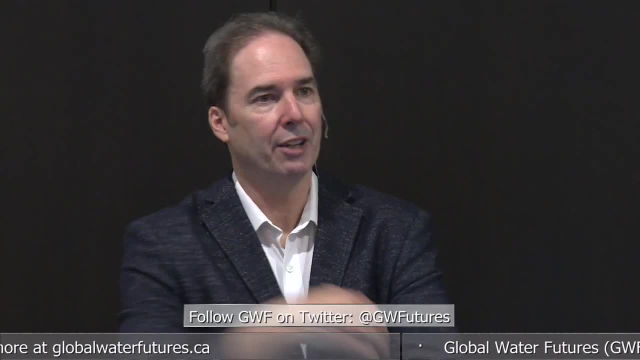 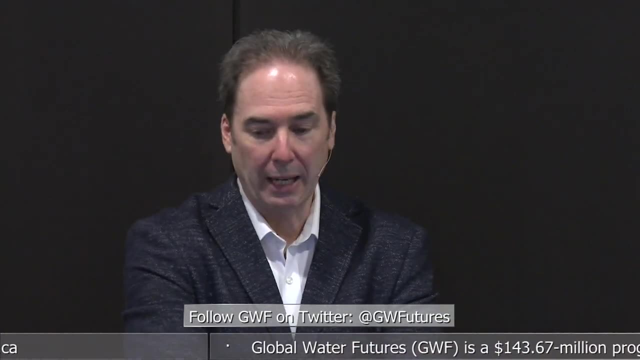 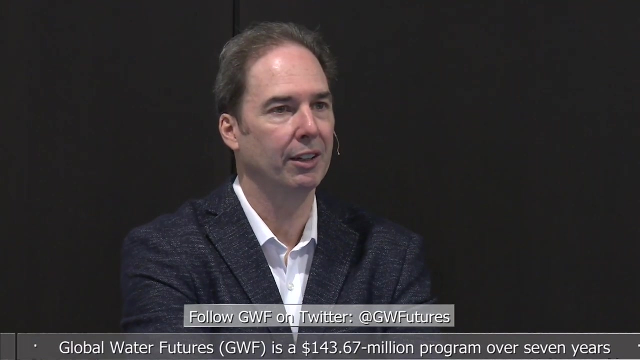 and our spin-up might be 100 years because we've got some old recalcitrant water that has to make its way through into the system And I guess the practical issue is that for a lot of water chemistry, nutrient studies, you're a pig farmer in North Carolina. 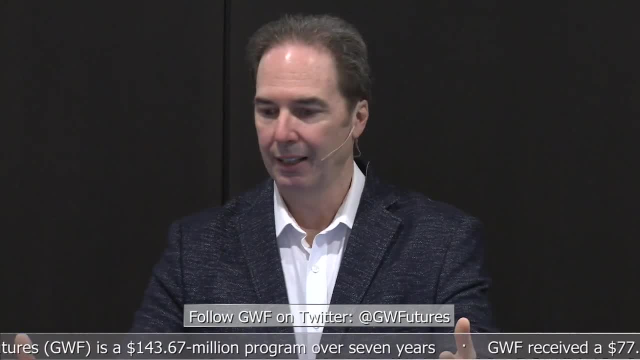 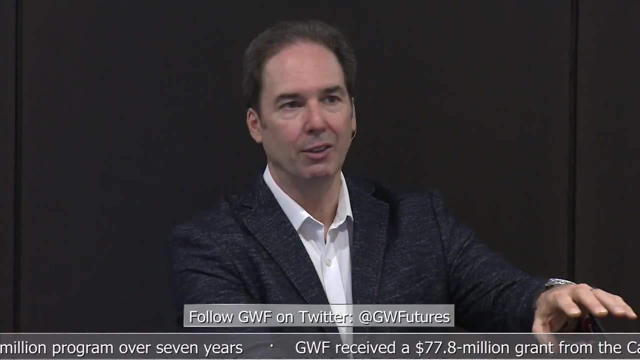 and you're putting out manure on your fields, That's going to get into the groundwater in this coastal plain watershed and it's like a ticking time bomb to get to the stream, which could be decades, And if you're trying to model stream water, 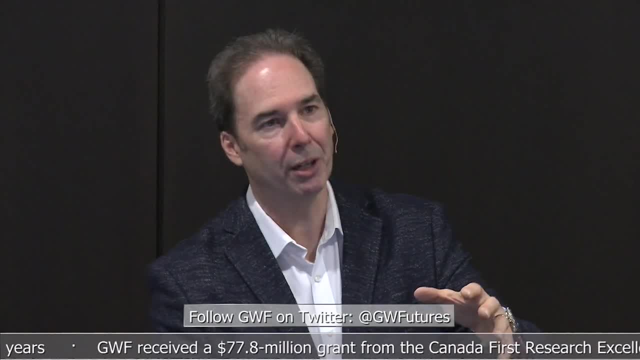 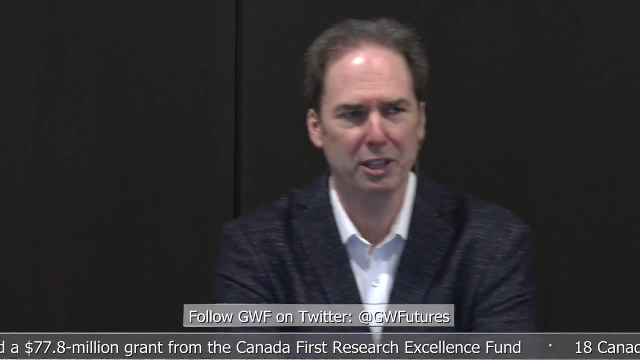 or nutrient dynamics, and you've not taken into account that long conveyor belt. yeah, it could be really a different outcome. So I agree it's super challenging, but I think getting some data will be helpful And I've been working with Al Petranero. 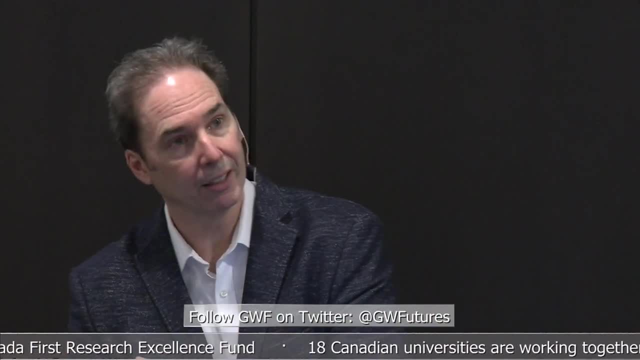 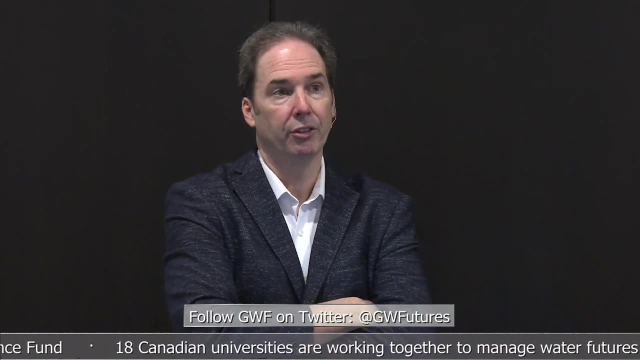 to see if we could get the Water Survey of Canada to start collecting stable isotopes on gauging stations under his purview. The US Geological Survey did this with about 390 of their catchments. They got some fragments of data. Man, it was a game changer. 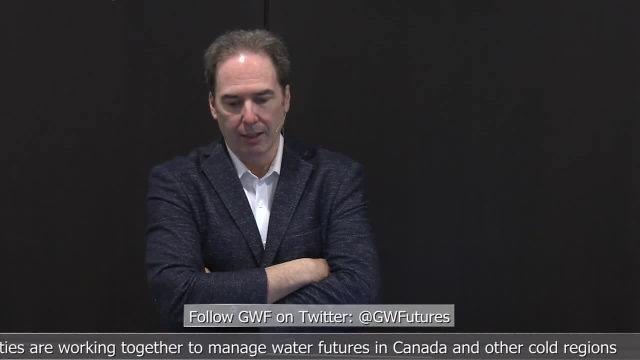 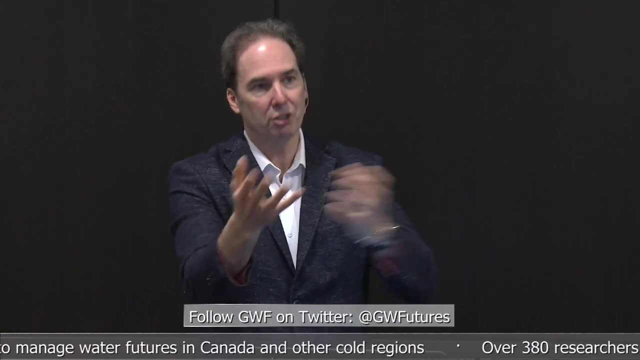 It's now being used with models, models being developed in some of these sites, and it's been really revealing, I think, And I think if we could start to collect some of these data and show the power, maybe usefulness, where it could be really important. 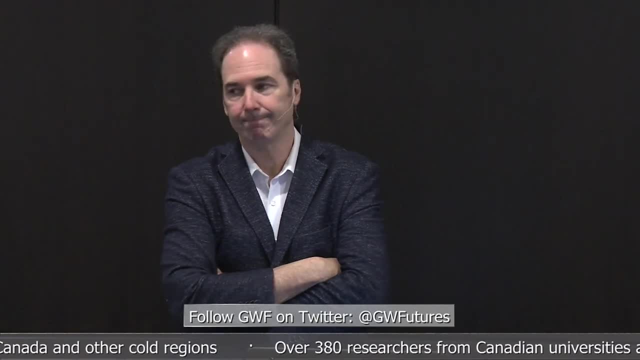 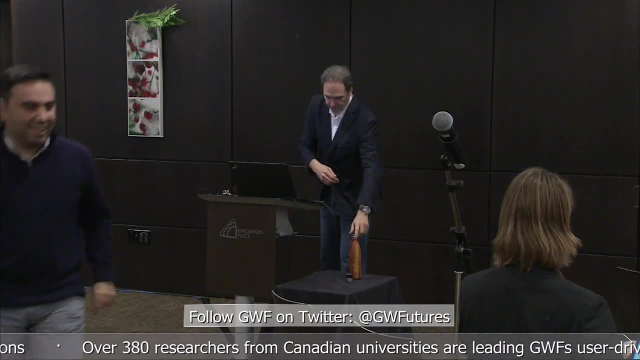 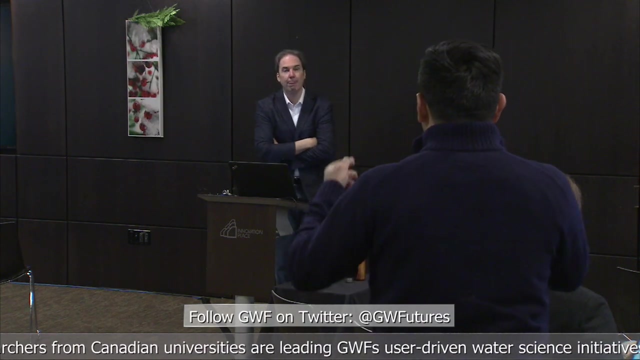 where it's less important. that'd be helpful. Yeah Yeah, Razi, I have a very simple- I mean sorry if it looks simple- question, but you talk about the old water in the stream. So then my question is: 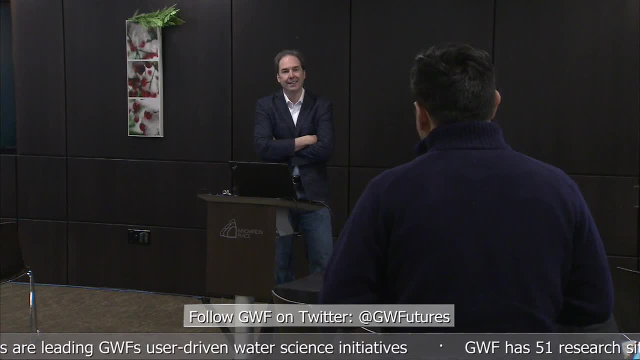 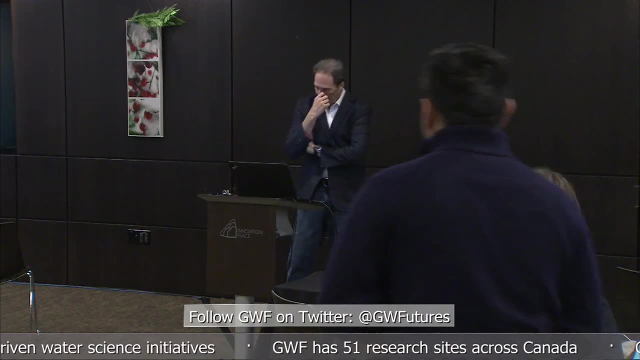 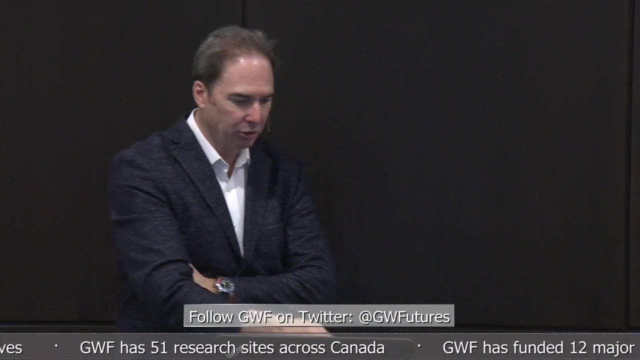 so where does young water goes? Yeah, So if it's that much old, so what happens to that? the young water, Right? Yeah, So maybe a super simple analogy, just to kind of kick it off, is: imagine a full garden hose in the summertime. 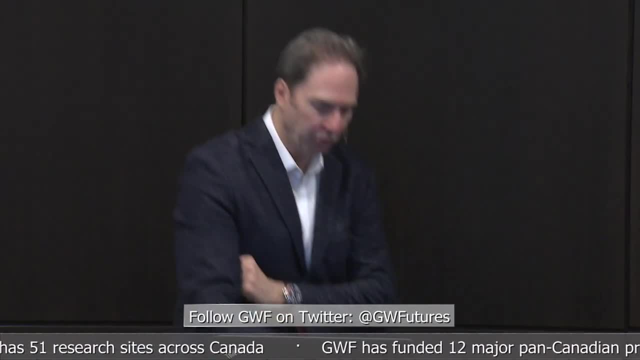 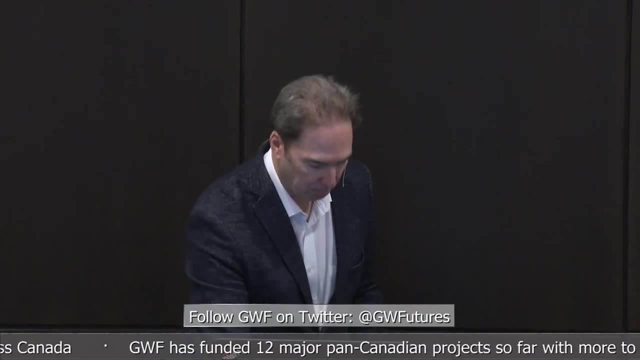 in your backyard and you pick up the end of the hose and instantaneously water squirts out the other end, 10 meters Down the other end of the hose. So that's kind of the pressure propagation through the hose, if you like. 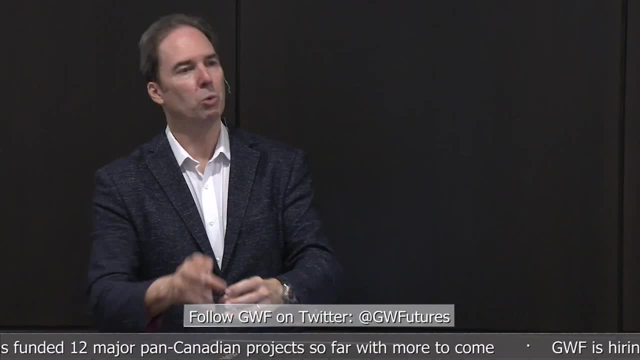 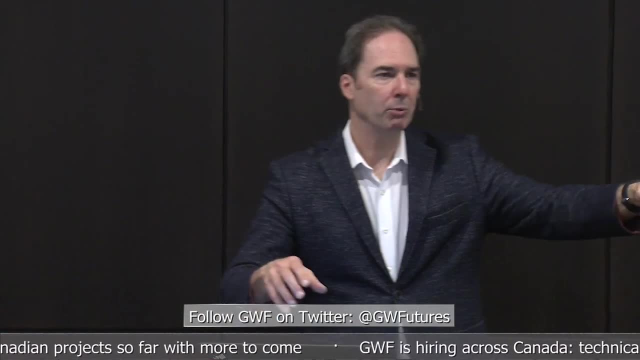 And then if you hook that hose up to the cold water tap outside and you turn the water on instantly, water is coming out the end of the hose but it's warm because it's been sitting out in the sun on the summer day. Cold water from the tap could take many minutes- 20 minutes maybe- to get to the end of the hose, And that's illustrating a difference between the pressure propagation and now the velocity of the water itself. So I think that's the issue. 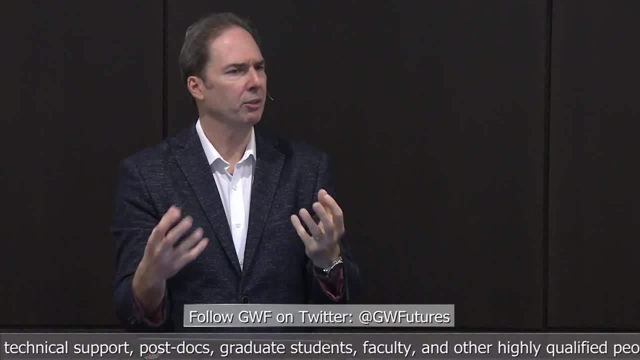 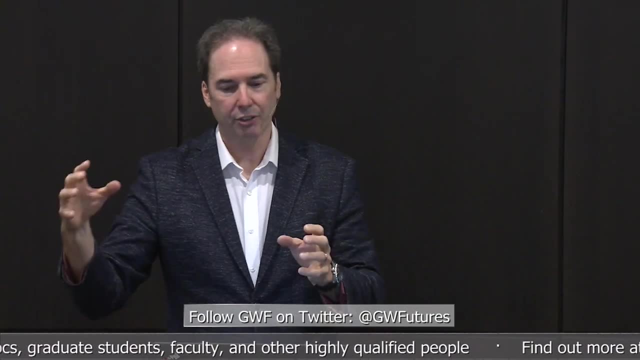 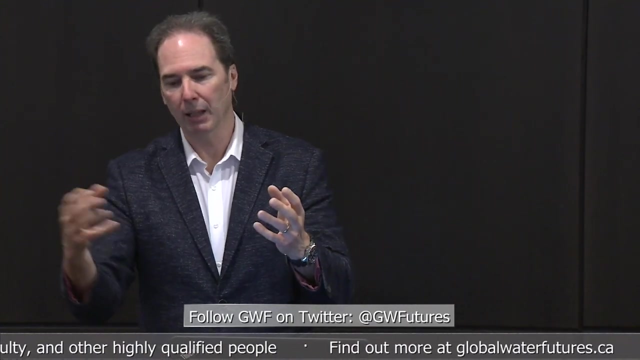 It's two different things that we're kind of talking about. So the ups and downs of the stream is the pressure impulses and it's some form of displacement, but the way the catchment's plumbed, the flow paths, how they blend together. 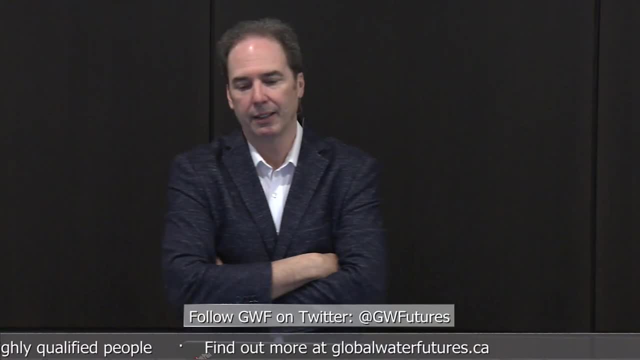 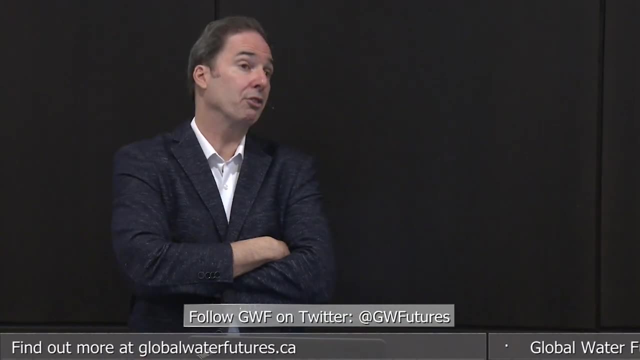 that's what's determining how it's being pushed out, And man the devil's in those details. I think what many groups are trying to do is to try to classify or bin or come up with a typology of these responses, And it's in its infancy. 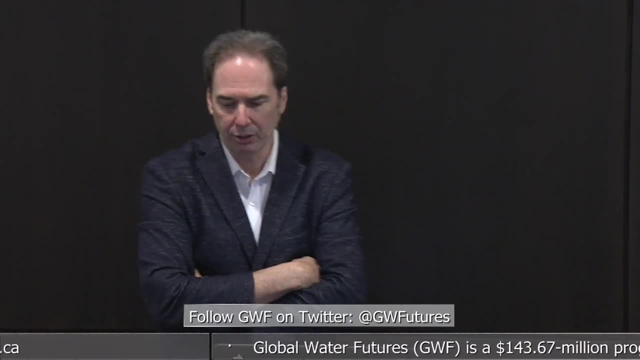 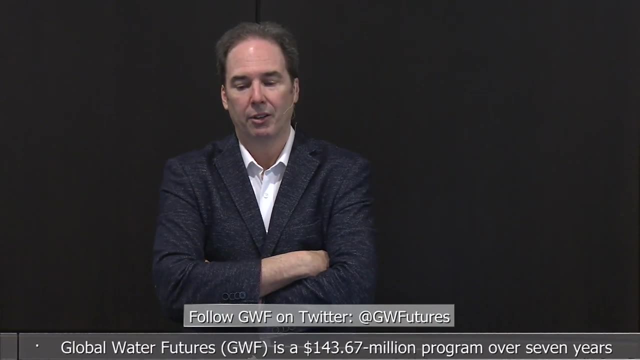 but I think that's a important way to go. I was just chatting with Tom Gleason at University of Victoria who's pushing on this again. There have been attempts over the years to try and get at that. So yeah, these are tough questions. 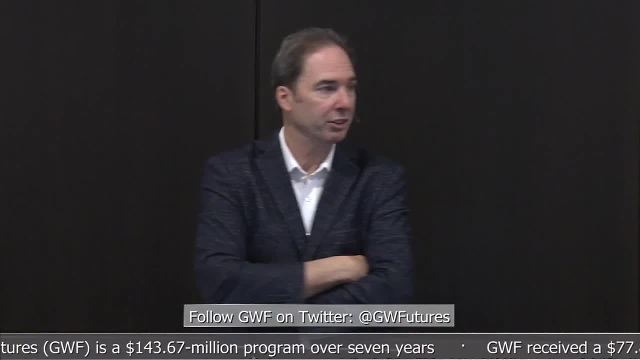 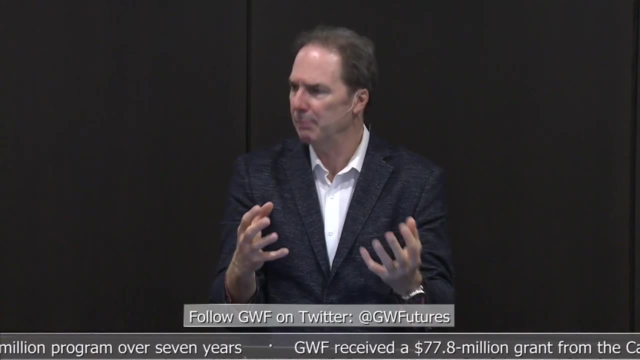 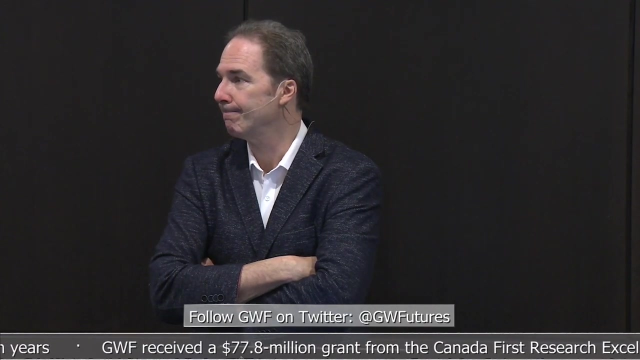 but I think where the field needs to be headed to tackle questions that are beyond the scope of science, beyond sizing a culvert, where you're really thinking deeply about climate, land use change and how it's going to express itself in river systems. Okay, well, seeing no hands and a lot of thirsty faces.